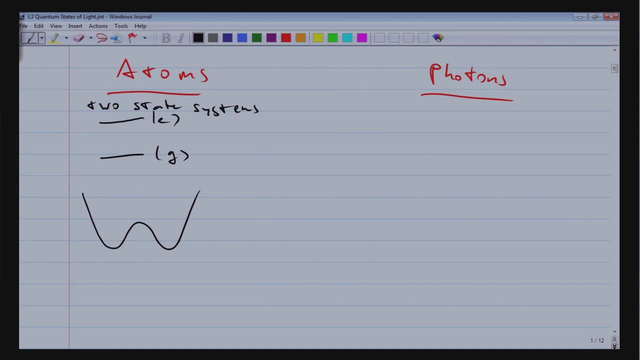 And photons are different. Photons are not two-state systems. They are actually harmonic oscillators, usually electromagnetic waves, But Hamiltonians for photons can be, and have been, realized By replacing the harmonic oscillator with a photon with vibrations, for example of ions in an ion trap. 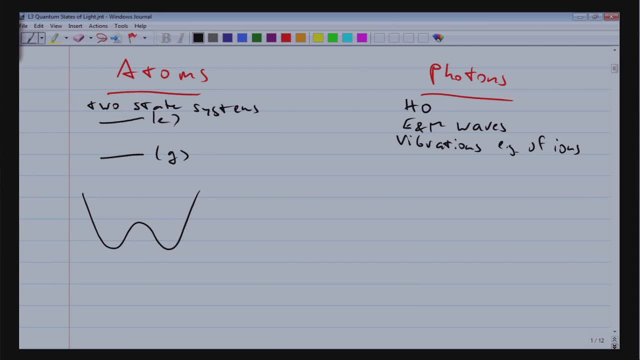 or micro-mechanical oscillators. So cartoon picture again is photons in a cavity. But this is just another, Another harmonic oscillator. So we have the atoms, And most of what you should know about atoms has been discussed in 8.421.. 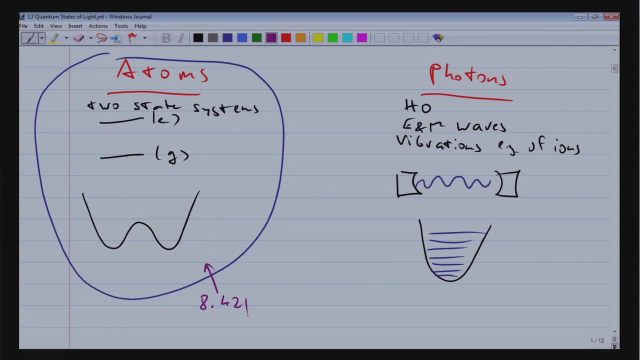 For those of you who will take 8.421 next year, we'll have a lot of fun talking about the structure of atoms, Photons. well, I would hope a lot of it, at least the harmonic oscillator aspects you took in 8.05 or in 8.321.. 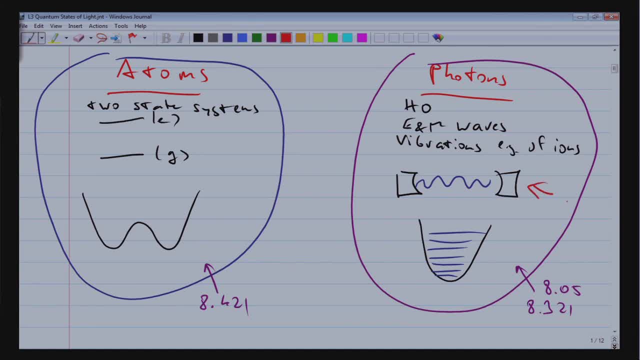 And actually starting today in this unit, we want to talk about the quantum nature of light. So you can say 8.421, we had a deep look at the 8.421.. The atoms: we have now a look at the photons. 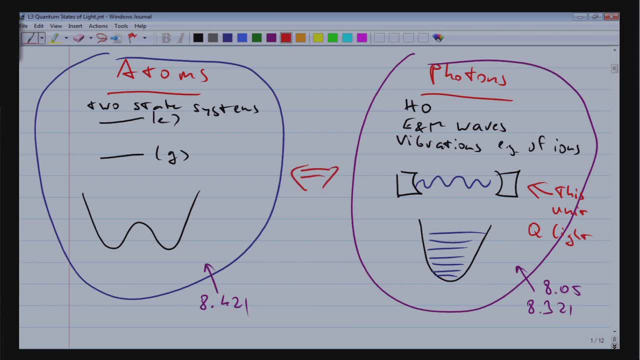 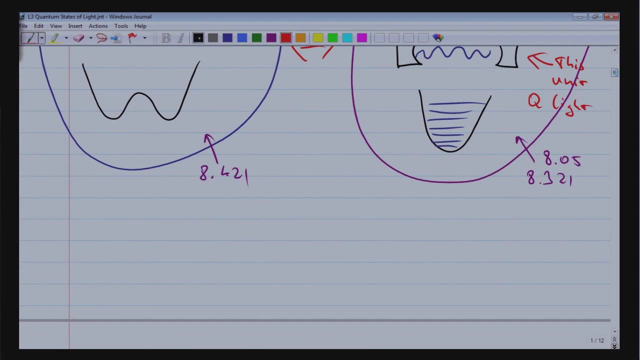 But eventually, what is very important is the interactions between the atoms and the photons. That's not all. This is sort of a very well-defined system, a two-level system and one mode of the harmonic oscillator, But it will become very important. 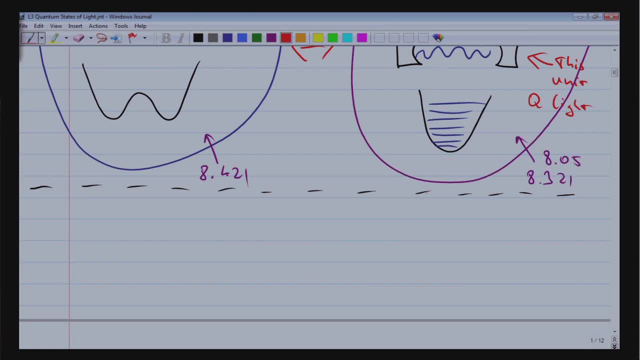 and that's what we do in a few weeks, to discuss what happens when this system, the system above the dotted line, becomes an open system and we interact with the reservoir. The reservoir will be relevant for relaxation. Atoms can decohere, can lose their decoherence. 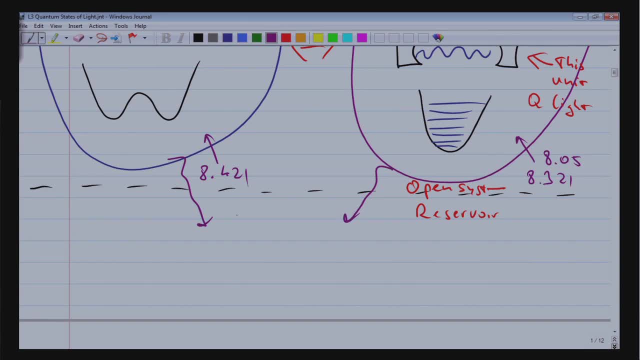 Photons will decay or decohere, Entanglement will get decayed, It will get lost, And this phenomenon of relaxation requires the formalism of the master equation. And we will find the master equation in the form of the optical block equation. 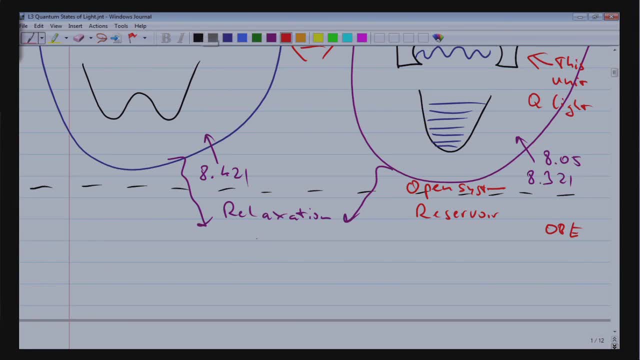 If you want me to add a cartoon picture of the reservoir, I would add many, many harmonic oscillators. So a reservoir is characterized by having many modes and having a capacity to absorb energy without changing its state. So this is another kind of illustrated summary. 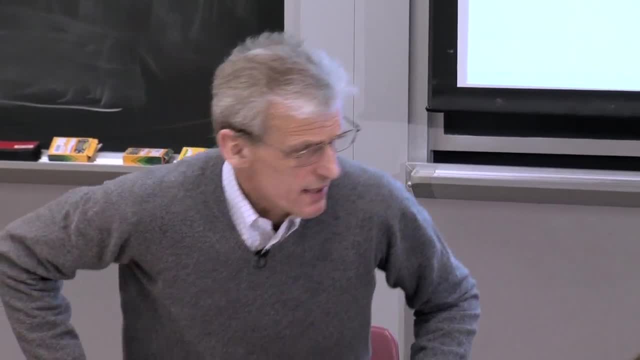 of what we will be doing in the next few weeks, And this is a photo of the reservoir, And today we will be reviewing the theory of this And, if you ask me, I'm going to write a summary. and I'm going to write a summary of this. 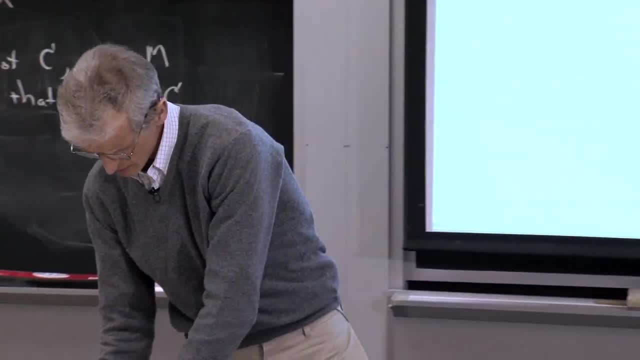 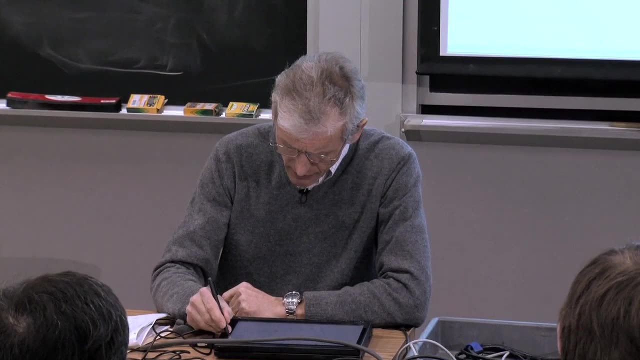 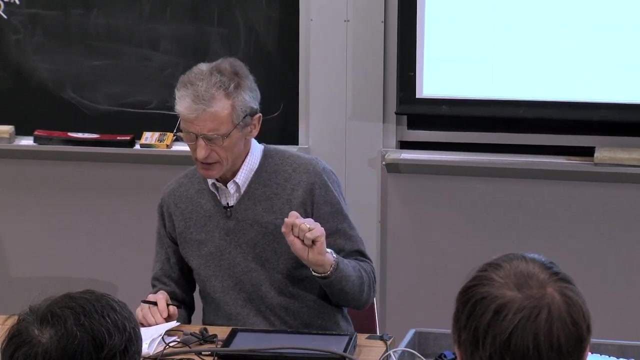 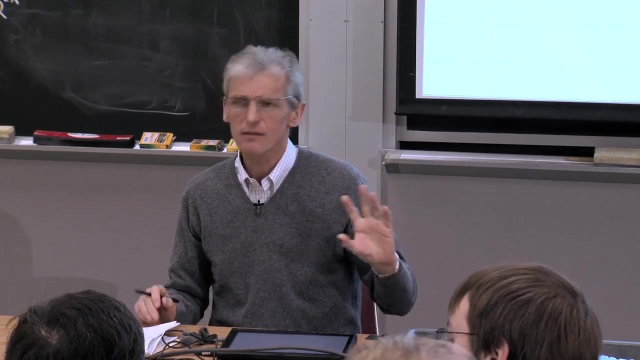 we want to talk about the quantum nature of light. We're actually talking mainly about already a very special form of light, namely monochromatic light in a single mode of the harmonic oscillator, And there is still a lot to be discussed about the statistics. 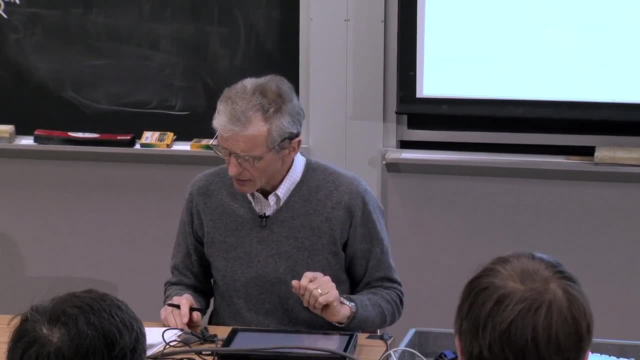 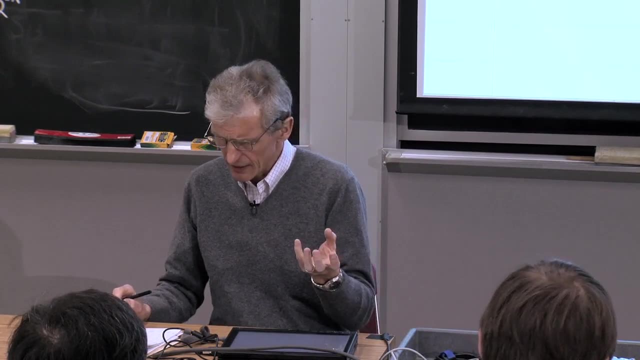 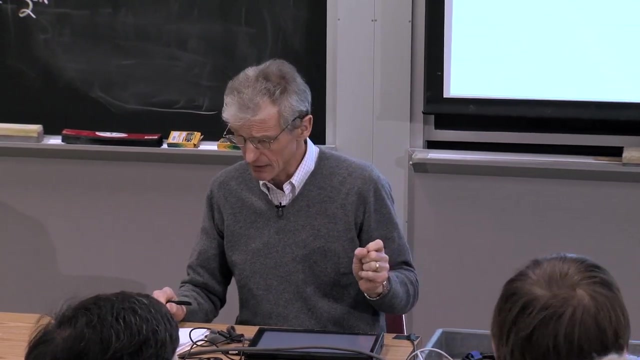 about squeeze states, about coherent states. We want to understand how the quantum state of light is modified, is transformed by propagation, or how it's modified when the light runs through a beam splitter. And all this is already relevant for just a single mode. 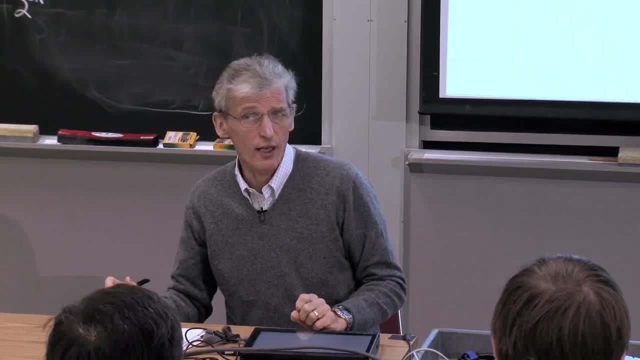 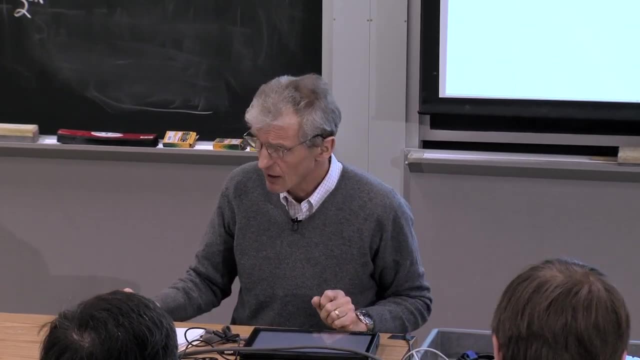 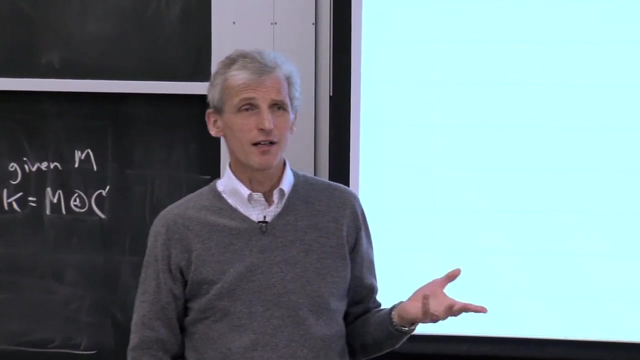 And then, very soon, we will also talk about two modes of light, because we need two modes. if we want to talk about light, We want to talk about entanglement of two modes. I hope you will realize in this discussion that the quantum nature of light is more than light. 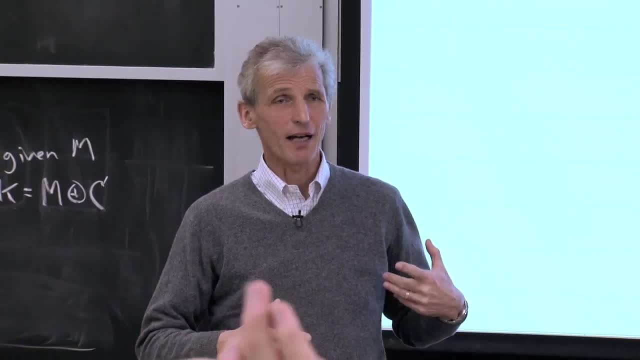 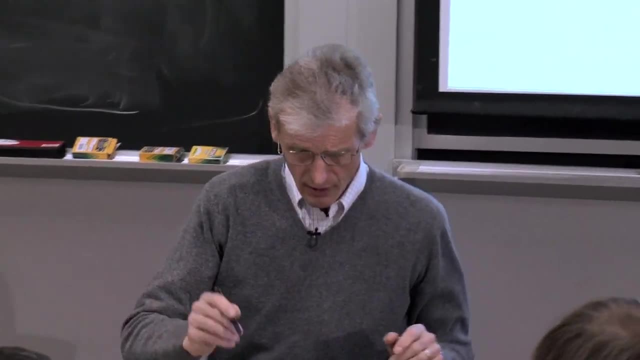 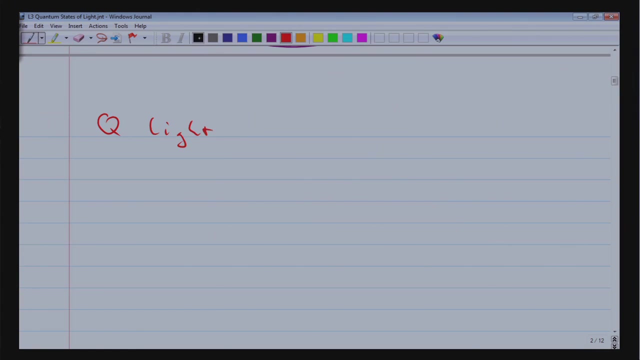 is a wave in the form of electromagnetic wave, or light is a particle in the form of photons. Things go much, much deeper. So the unit on quantum light will actually evolve in Six stages. Today we will be talking about photons and statistics. 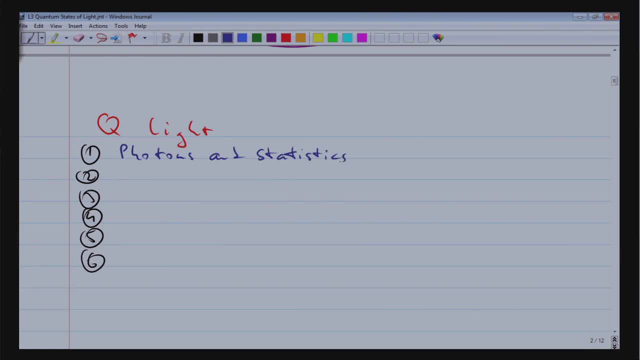 fluctuation coherent states. Next week, on Monday, we want to talk about non-classical light states, which have no classical analogy, and squeeze states. Eventually, we want to focus on single photons. We will then talk about entangled photons. 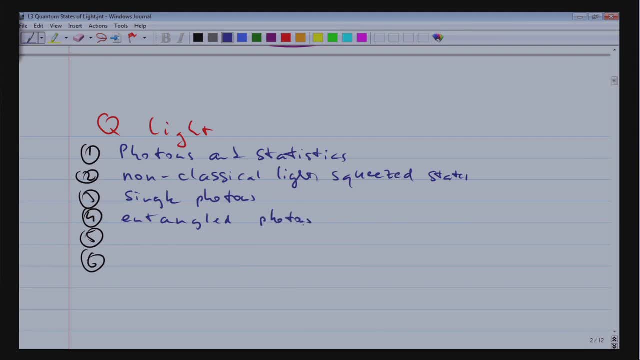 The fifth part is on interferometry or more generally on metrology. We will talk about the shot noise limit and the fundamental Heisenberg limit of performing quantum measurements, And the last one is now opening up situations where we actually up the light to interactions with atoms. 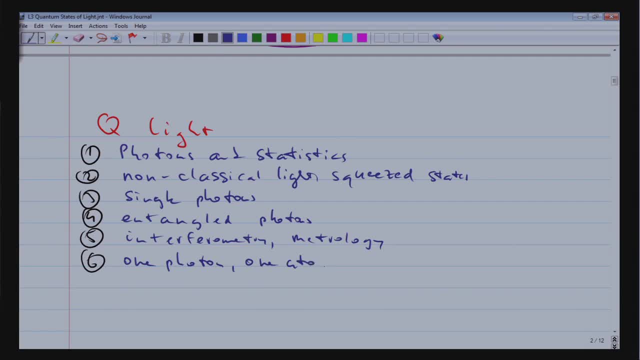 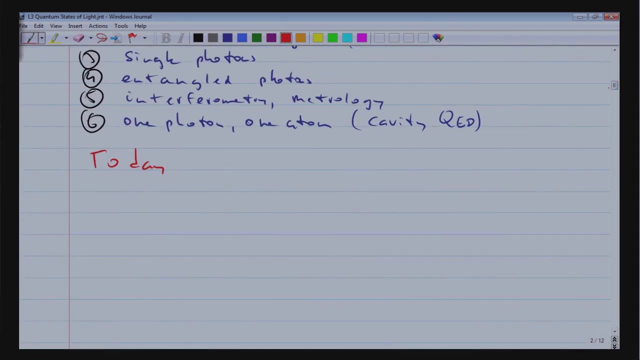 So we will talk about the interaction of one photon and one atom in this specific situation of cavity QED. So this is an overview over the next- I don't know- three, four, five, six lectures. Today we start with a very, very short review. 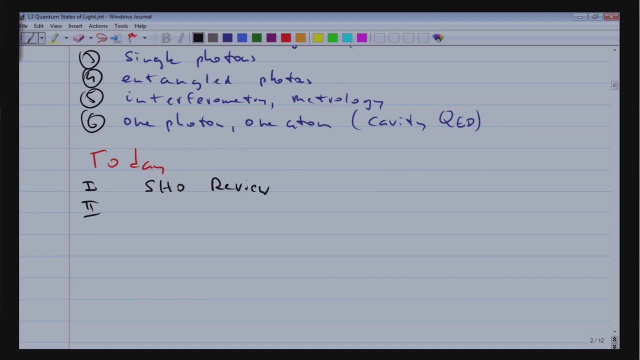 of the simple harmonic oscillator just to set the stage. I then want to show you that in three minutes I can discuss thermal light and the Planck law by just writing down one or two equations in the formalism we have chosen. So we cover thermal states. 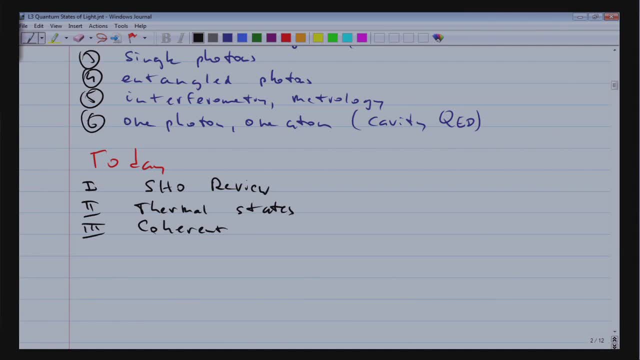 When we do laser physics, when we have light-atom interaction, we always need coherent states And we talk about quasi-probability distribution. We then want to understand fluctuations, noise and second-order correlation functions. Probably this will spill over into the next class. 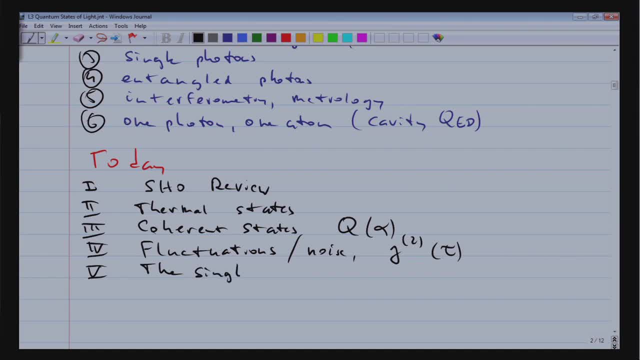 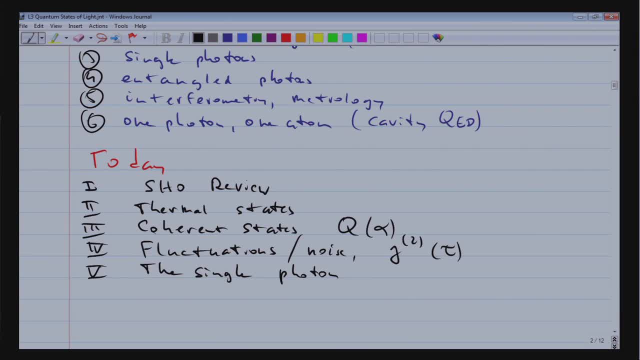 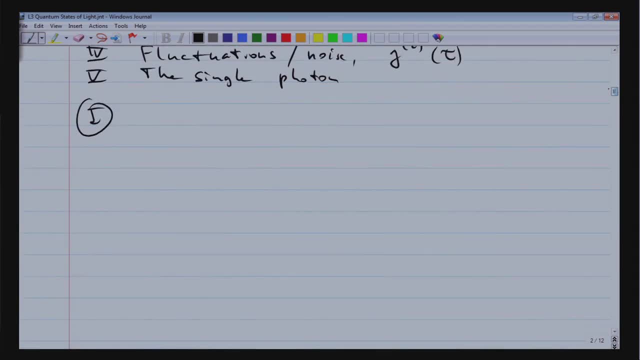 you can have a single photon, But we'll come to that. OK, Let's start with a very, very short review of the simple harmonic oscillator. It just also connects me with the last lecture. So how do we describe light in a single mode? 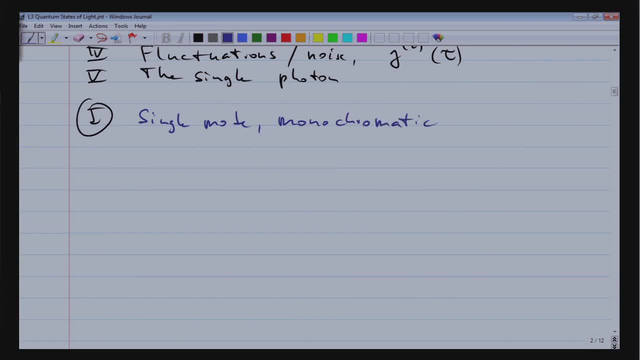 And single mode means it is perfectly monochromatic. Well, we know that, and that's what we did last class- that we have the Hamiltonian for the electromagnetic field, which is the quantum version of the electromagnetic energy: B square, E square. 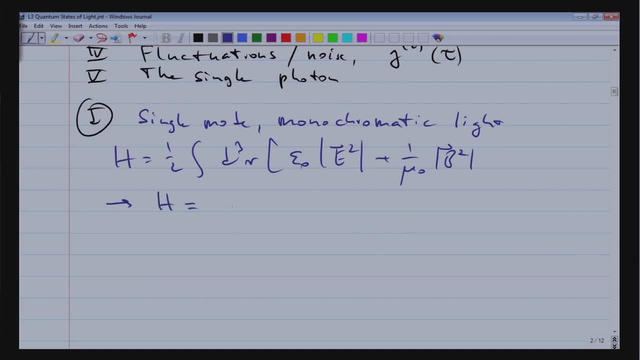 And from that we derived the quantized Hamiltonian. We introduced, just as a reminder, vector potentials, normal modes and the normal mode operators became the a-diggers, And in second quantization this is the Hamiltonian for light. 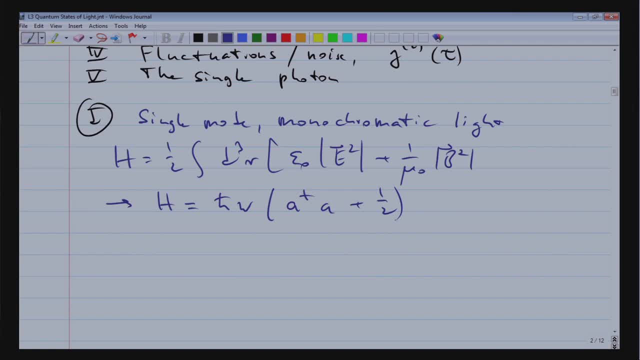 which is, of course, the Hamiltonian for a harmonic oscillator. What I need today is: I need to be able to do this. I have to rewrite the harmonic oscillator and we have to look at two variables: the momentum and the position. 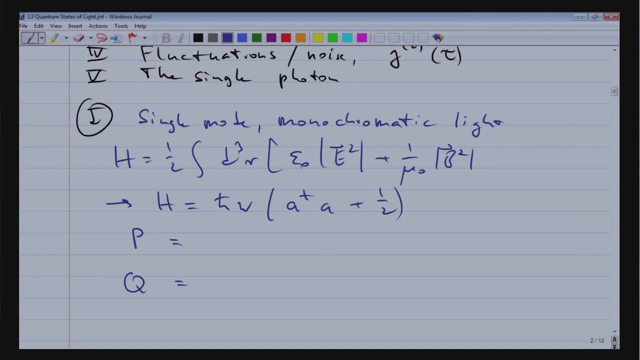 Actually the momentum. we later I will show you that the momentum of this harmonic oscillator is actually the operator of the electric field. so we need that in a second. And of course I assume you know from your knowledge of the harmonic oscillator that position and position and time. 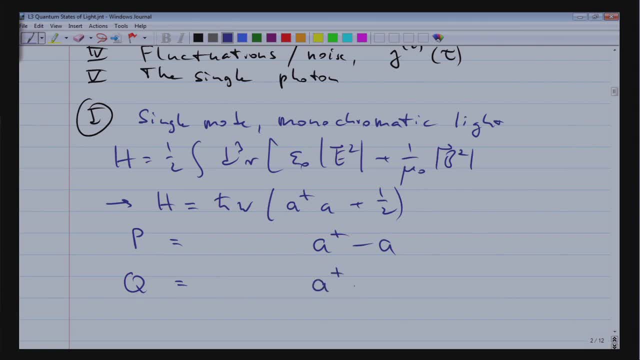 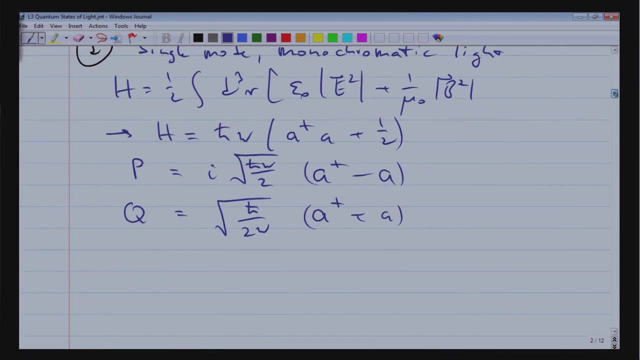 are all related and momentum are linear combinations, symmetric and anti-symmetric, of a dagger, a, And the unit is the prefactor square root of h bar, omega over 2, or here it is h bar over 2 omega, And, of course, in position and momentum, operators. 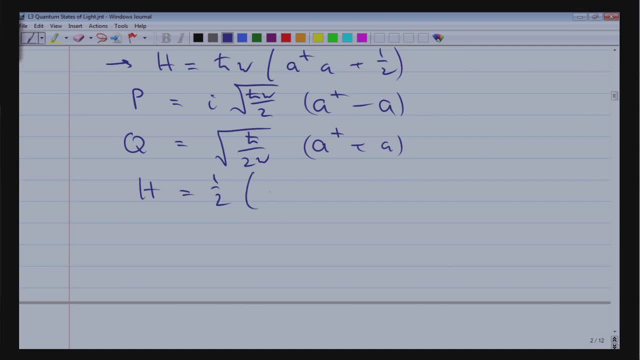 the Hamiltonian is simply p square should remind you of kinetic energy. Omega square, q square should remind you of potential energy. When we discuss light, we want to discuss the electric field We had. I had shown you in one of those hundred equations. 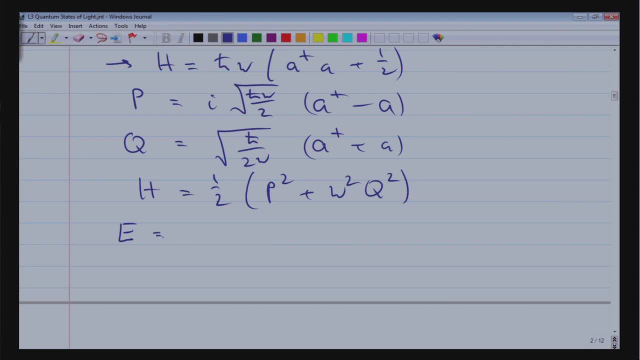 the operator for The operator for the electric field. The operator for the electric field was, of course, related to the vector potential And the vector potential we did a normal mode expansion And then we put everything backward And we found that the electric field operator 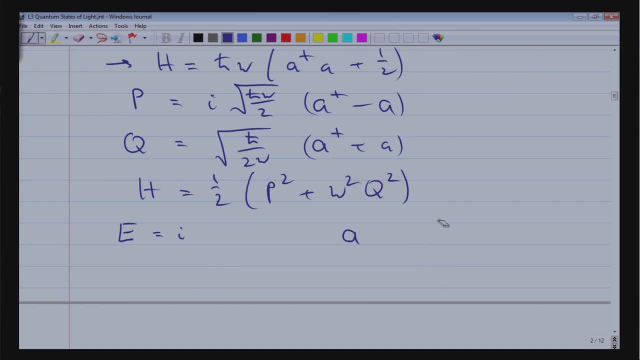 can actually be written. I have to fill in a few things, but essentially the operator is a minus a dagger, And a minus a dagger is nothing else than the momentum of the harmonic oscillator. So here the momentum has a special role. 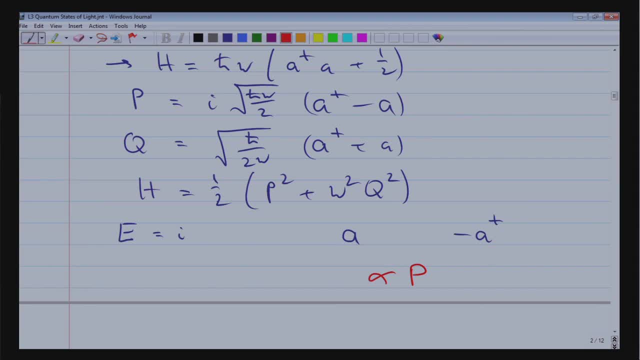 because it is the operator of the electric field. If you have light in a single mode, it has a harmonic oscillator representation And the operator for the electric field is. I put in a few bells and we're done. We're done. 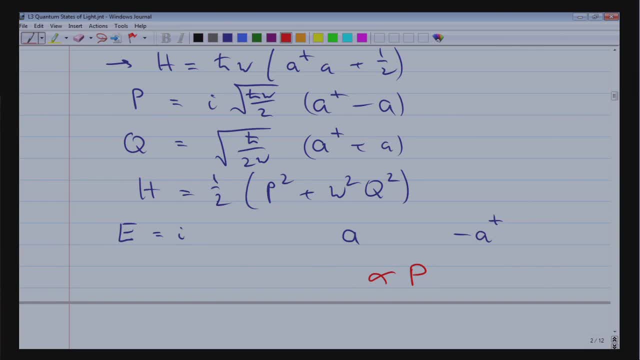 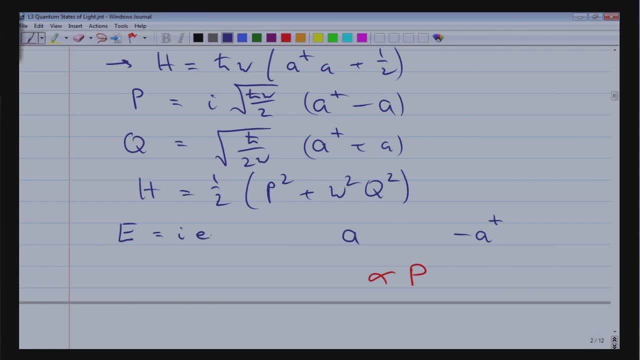 OK, But the electric field has a polarization. We need that. It has the photon energy and the quantization volume. What I'm writing down here is actually the electric field. This square root is the electric field strings of a single photon in the quantized 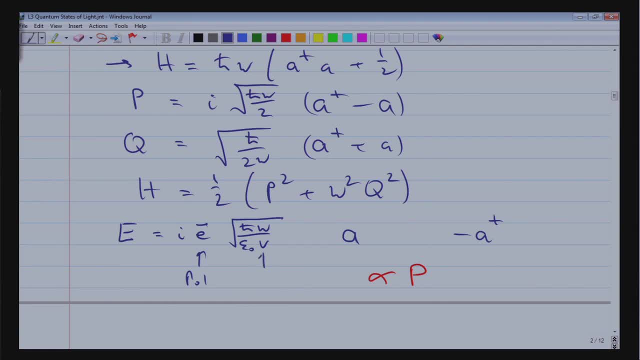 volume of our cavity. So V is the quantization volume. Then, if we have a single mode of the electromagnetic field, well, in contrast to a harmonic oscillator, we have a propagation: kr plus omega t, And here we have e to the minus i. 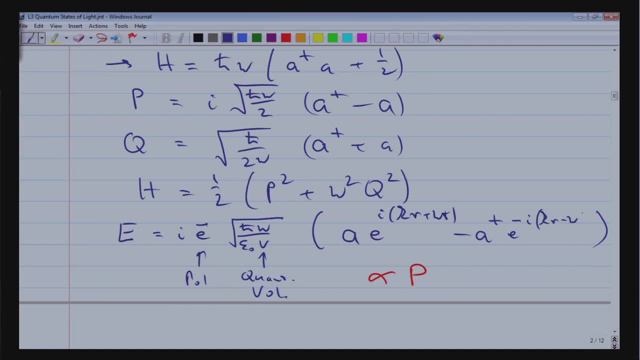 I hope I get the signs wrong here- Minus omega t, So therefore, but OK, we will mainly be looking at an atom at the origin. That's what we did in the dipole approximation. So when I said that the electric field operator corresponds to the momentum, 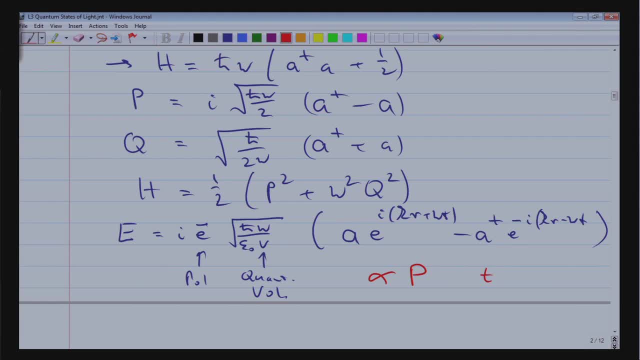 I have to add now that it is at t equals 0 and at r equals 0.. We'll come back to that in a few moments. OK, since I've given you the operator, let me just put the operator symbol on it. 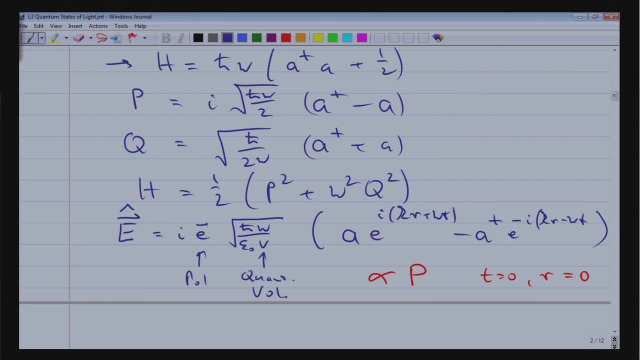 The operator of the electric field I have to say now one word about Heisenberg operators versus Schrodinger operators. I assume you're all familiar with the two different representations of quantum mechanics. We often use the Schrodinger representation where the operators are time independent. 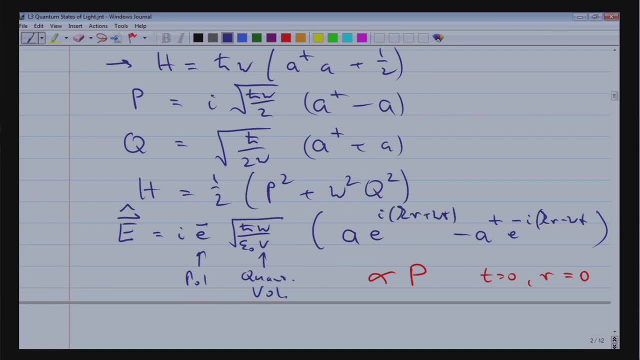 But in the Heisenberg representation the wave function, the state vector, is time independent, And the time dependence of the evolution of the quantum system leads to a time dependence of the operator. So what I've written down for you here is actually the Heisenberg operator. 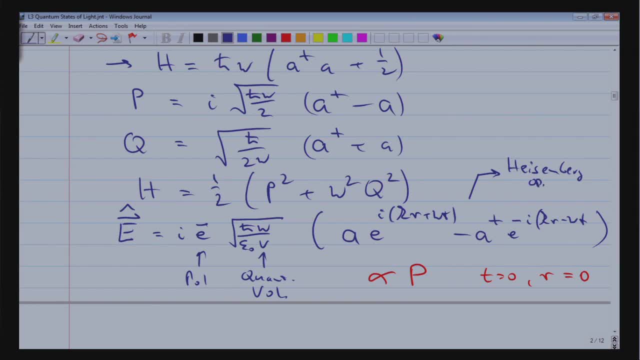 because it has a time evolution. But for a single mode, monochromatic electromagnetic field, the time evolution is just e to the i, omega t. So if you want to obtain the Schrodinger operator, you have to eliminate the time dependence by setting t equals 0.. 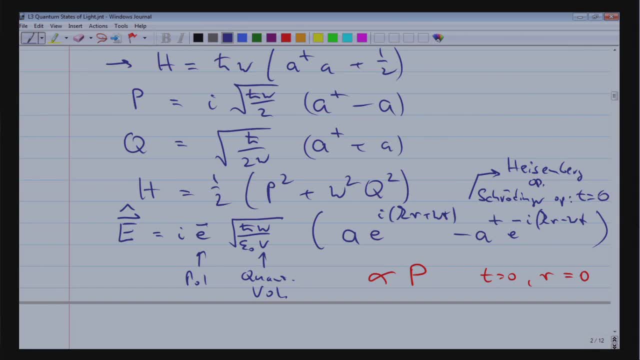 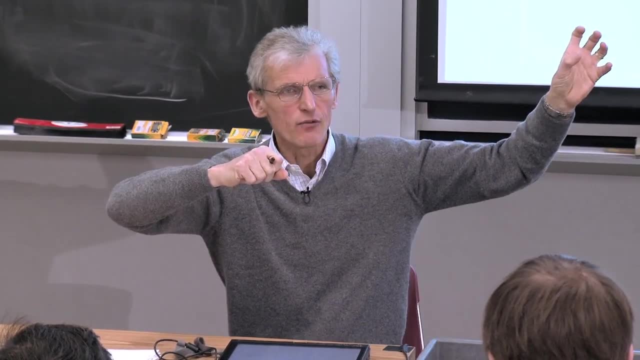 At t equals 0,. by definition the Schrodinger operator and the Heisenberg operator are the same. But then in the Schrodinger picture the quantum state evolves and the operator stays. So if you put in the Heisenberg picture: 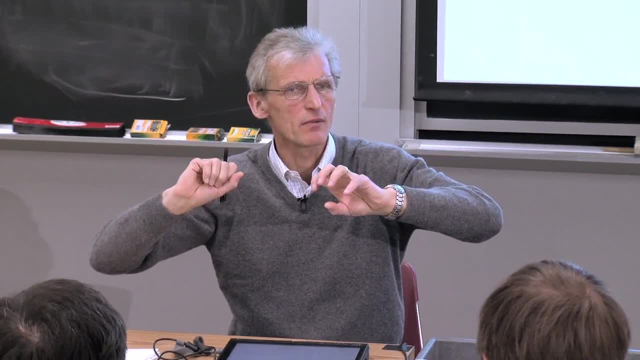 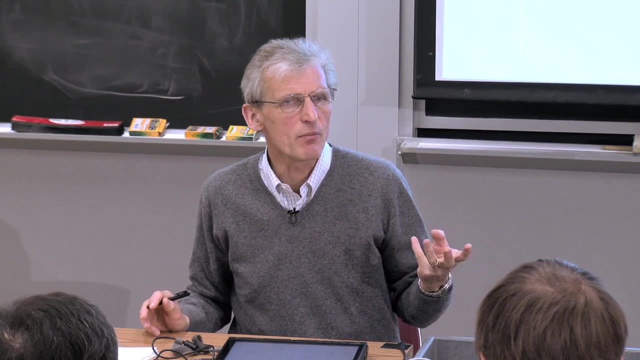 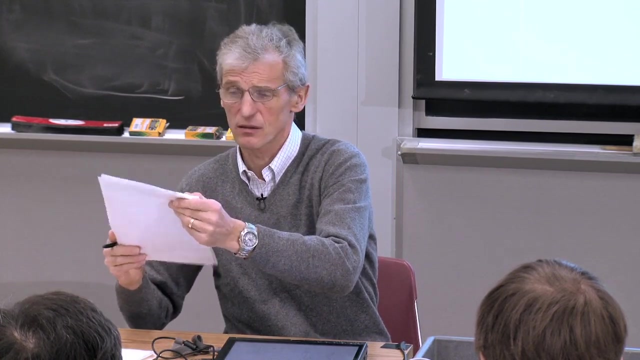 the quantum state stays constant and the operator evolves. So I'm usually writing down for you expressions for Heisenberg operators. But if you simply set t equals 0 in this expression, you have the Schrodinger operator Questions. Yes, Colin, 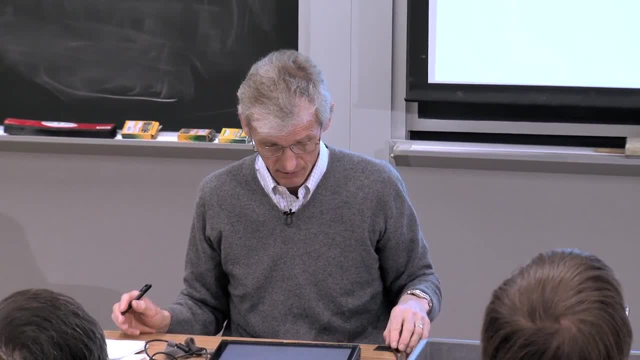 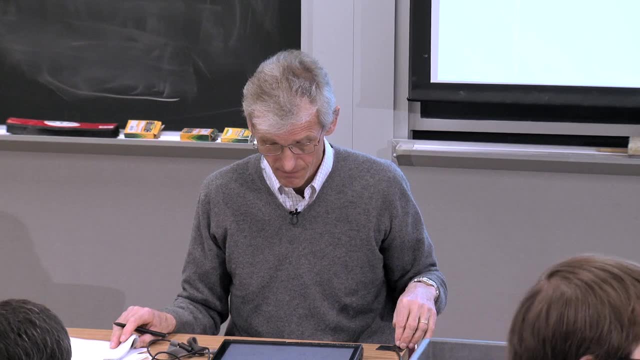 How does it factor 2 that shows up in the electric field for a single photon, like the amplitude expression? I thought it was like. I mean it's just factor 2, right? Yes, You have to be careful with factors of 2.. 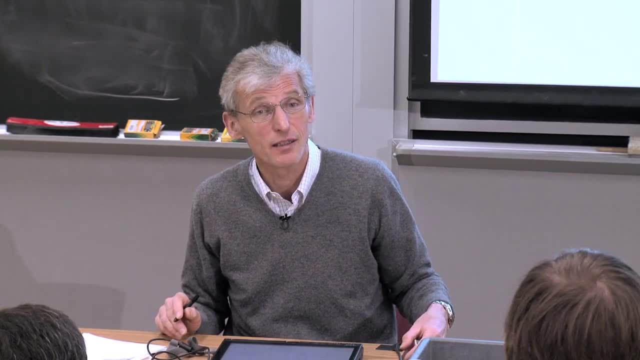 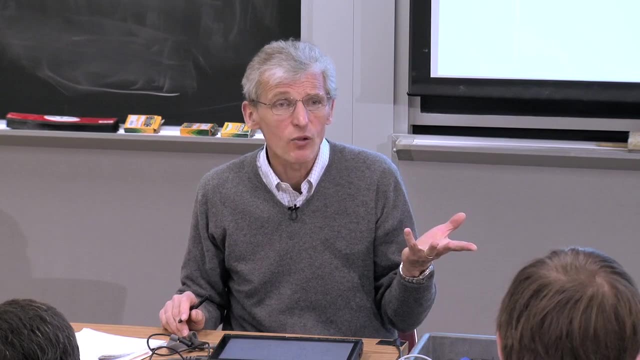 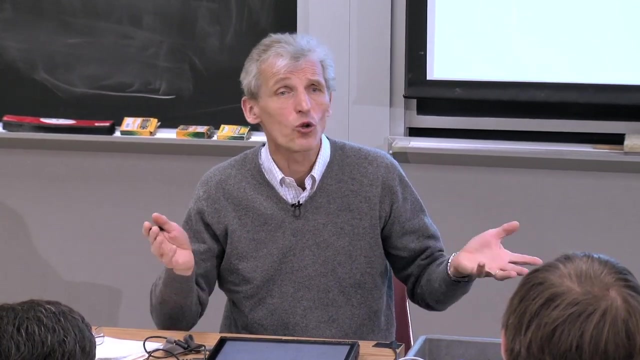 I think I got it right here. There is no extra factor of 2.. But the question is OK. whenever you write down equations for the electric field you want to sort of use a and a daggers, photon number or create photon numbers, so they're dimensions. 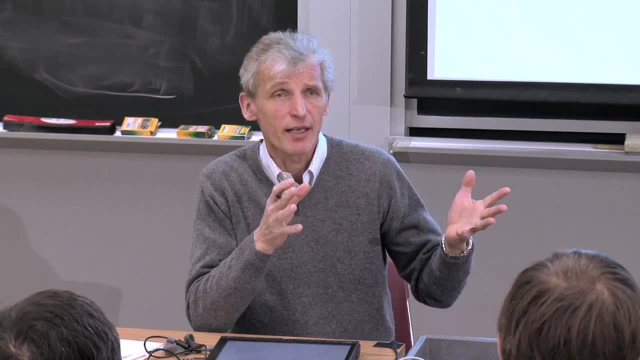 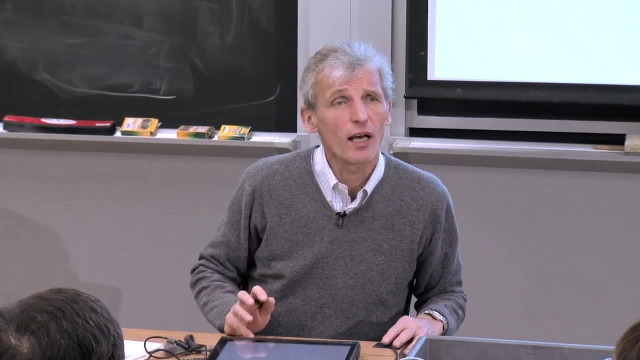 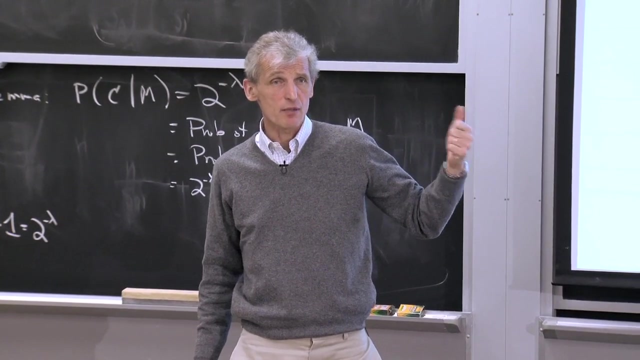 OK, So you always need a prefactor which has a dimension of the electric field. And for the quantization of light you have two choices. One is I can take the electric field associated with a single photon. That's one option. The other option is I take as a prefactor. 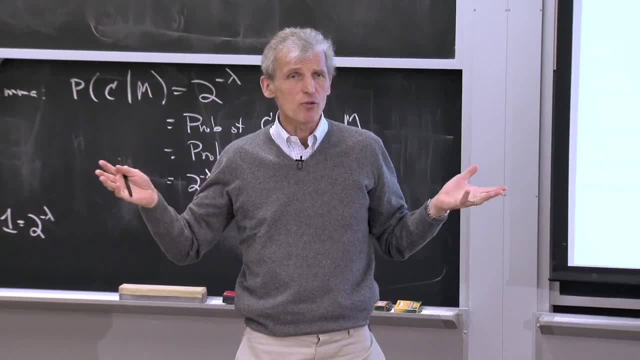 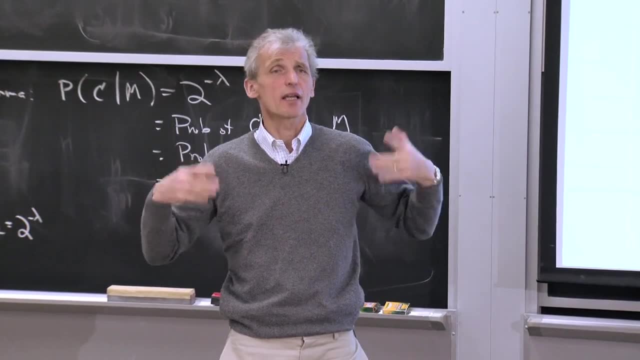 the electric field in the ground state, which you can say is the zero point. fluctuations of the electric field. OK, And the two differ by factor of 2. Because the energy of the vacuum field is 1 half h bar omega, whereas one quantum has h bar omega. 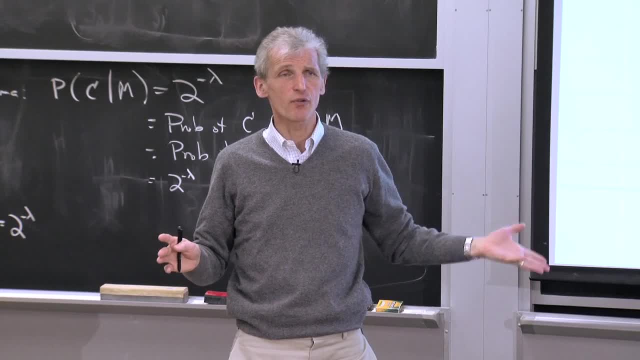 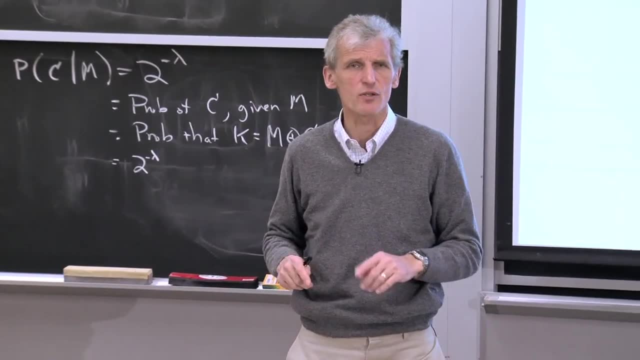 So that's one reason why you may sometimes find factors of 2 in some textbooks or not in others, But I think what I'm, I checked it. I think, as far as I know, it is consistent. So the operator for e. 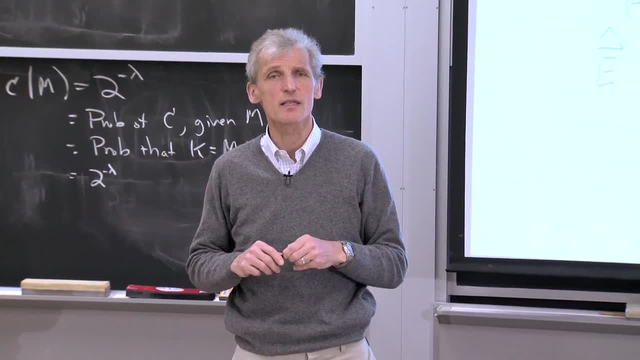 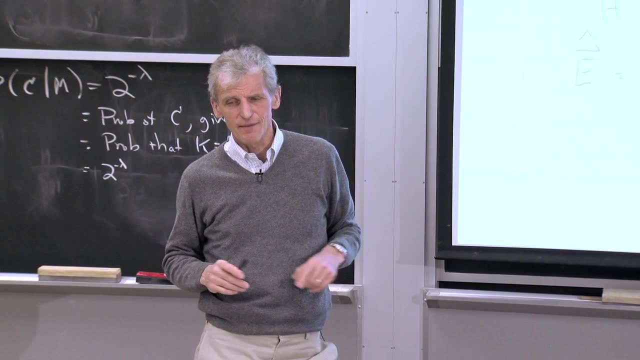 this is the Heisenberg operator with the. This is the Heisenberg operator for the electric field. OK, But it differs. I mean, at that point don't there's nothing really to worry about or get concerned about? The question is for monochromatic light. 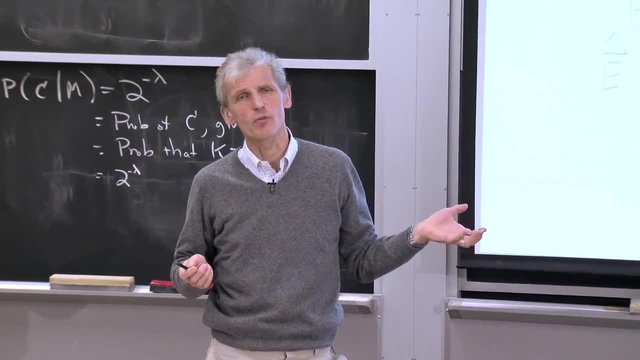 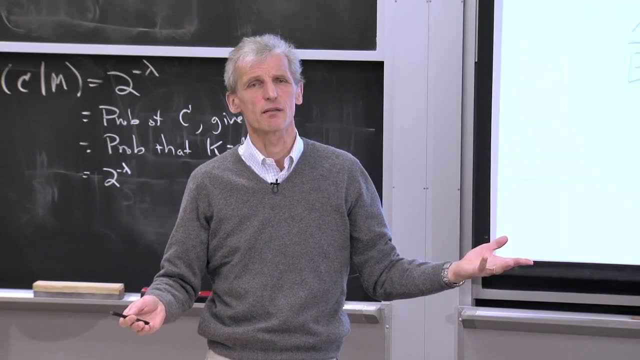 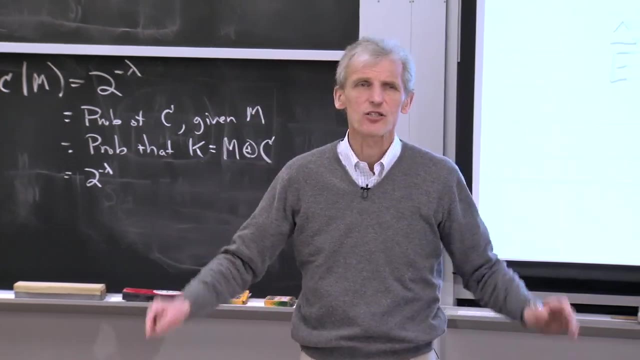 do we put the e to the i omega t into the state or in the operator? It's really just an e to the i omega t factor has to be put either on the state or on the operator. These are the two choices, Actually. 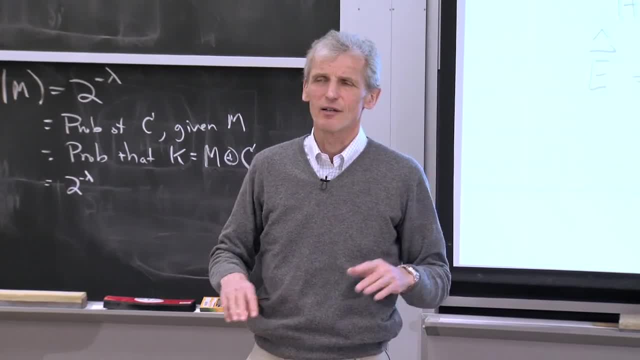 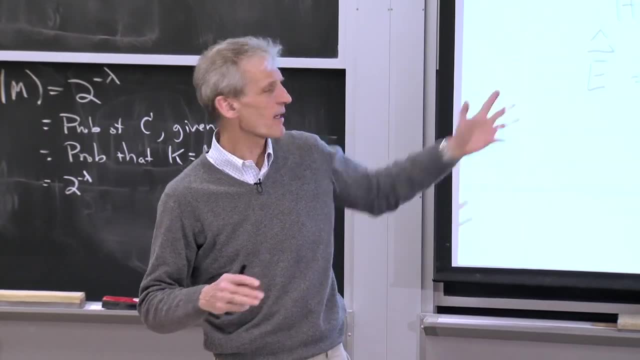 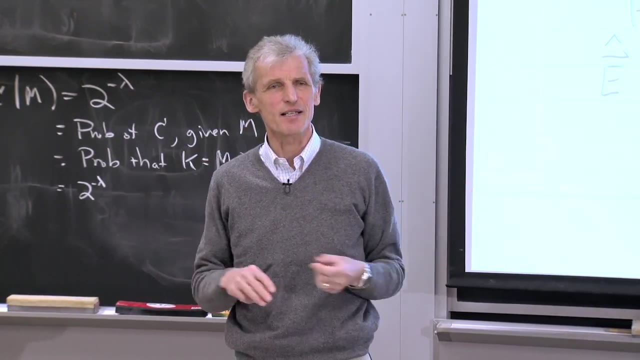 My advice, OK, My advice to you is: don't even develop an intuitive conceptual understanding And, whether you are in the Schrodinger, try to sort of see the structure of the operator. I sometimes like the omega t because it shows you how the electric field evolves and you see that explicitly. 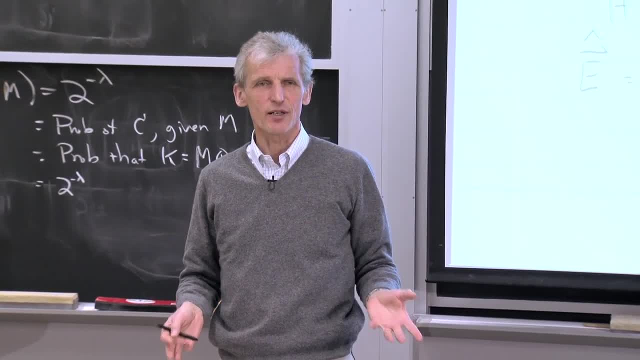 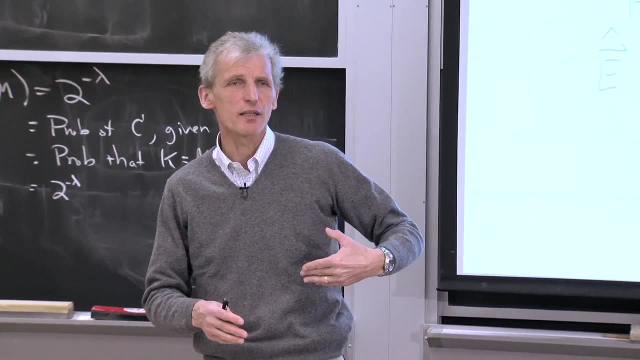 But in the end it's only when you do real calculation that you have to think hard. OK, which picture am I using now? Which representation am I using now? I'm probably not 100% rigorous in this course when I write down. 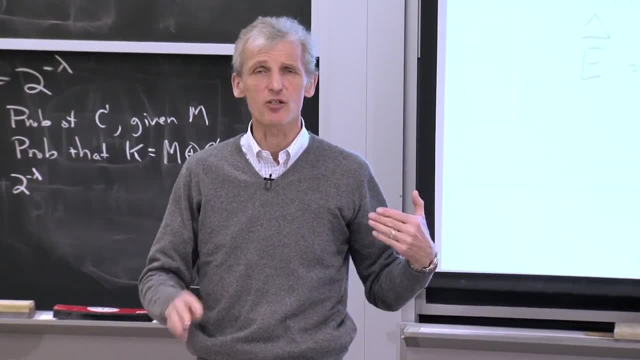 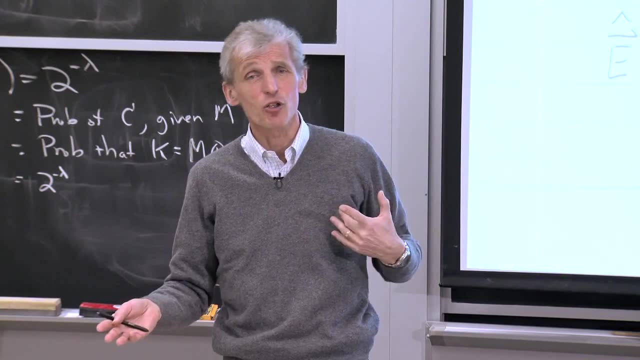 quantum states and operators, whether I'm always in the Schrodinger picture or in the Heisenberg picture, But by simply looking, does it have a time dependence? Yes, It's a Heisenberg picture If I write down a quantum state which has a time dependence. 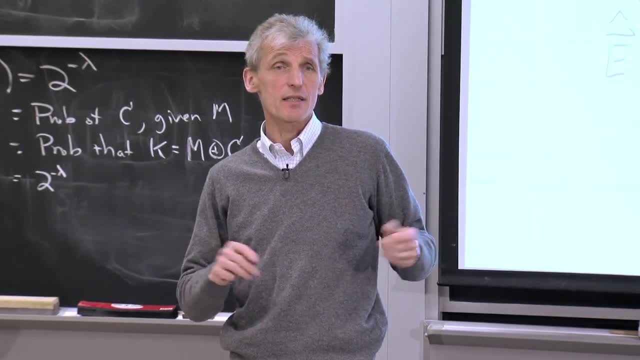 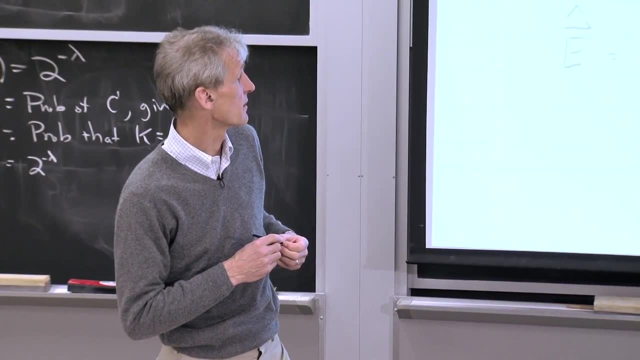 then I've chosen the Schrodinger representation. It's as easy as that. There was other. There's a sign wrong up there, Because both a and a dagger goes to the i, omega t, as you have written down. So they should be counted. 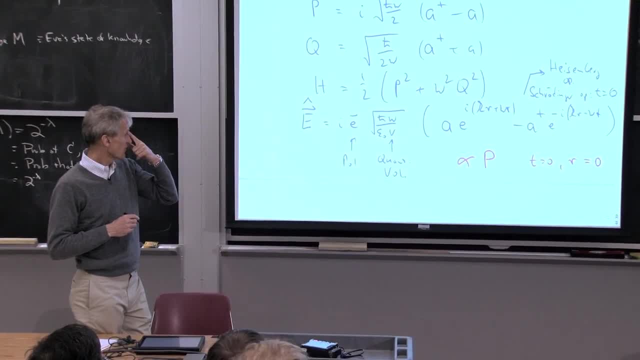 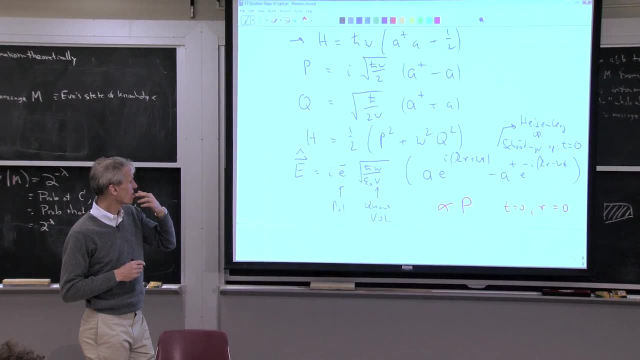 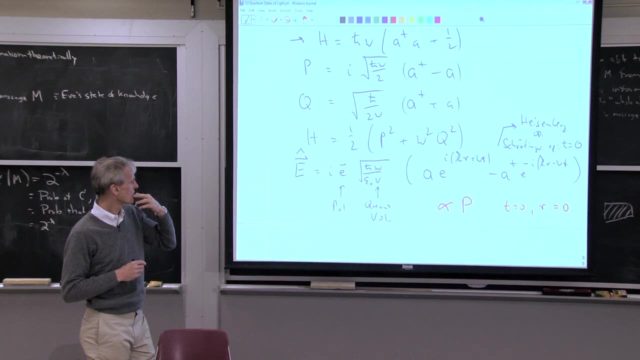 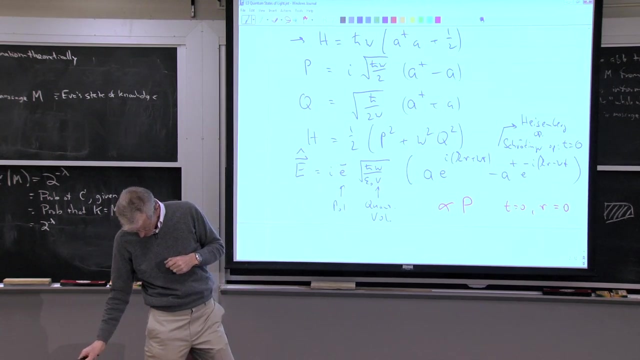 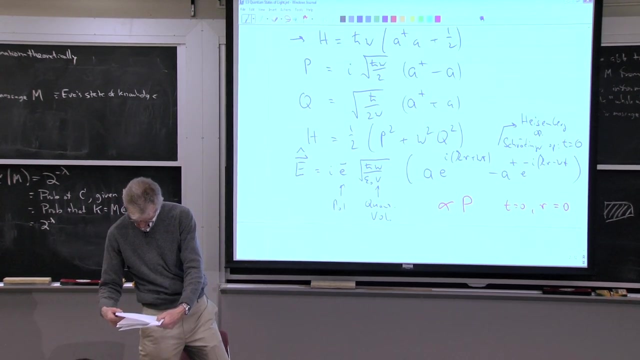 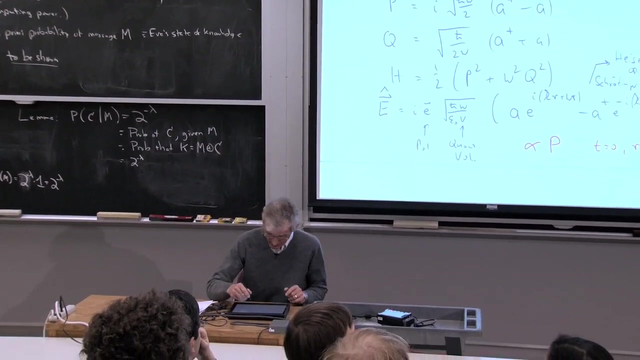 They're chaining right. Give me one second. I'm actually. I just wanted to say I was careful with my notes, but I didn't carefully look at my notes. This is what I have in my notes. Does that satisfy you? 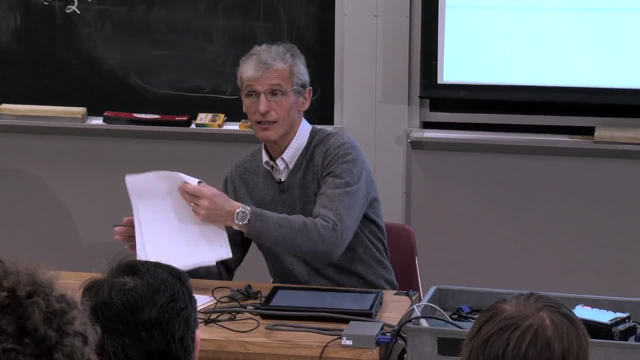 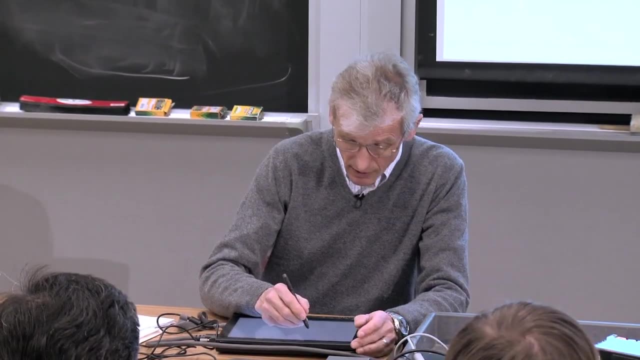 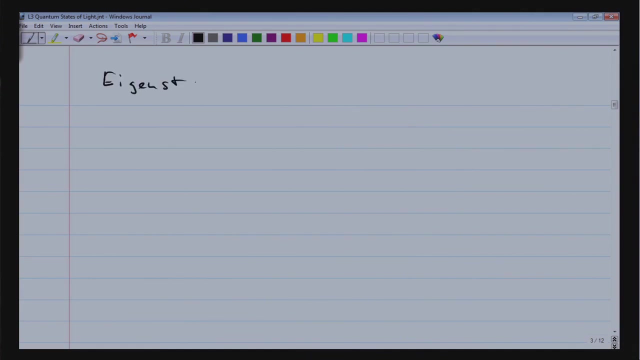 Yes, OK, Good, OK, So we want to talk about quantum states of light. The simplest eigenstates are, of course, the harmonic oscillator eigenstates, But, as I've already mentioned, and we'll elaborate on it further, these are actually non-classical states. 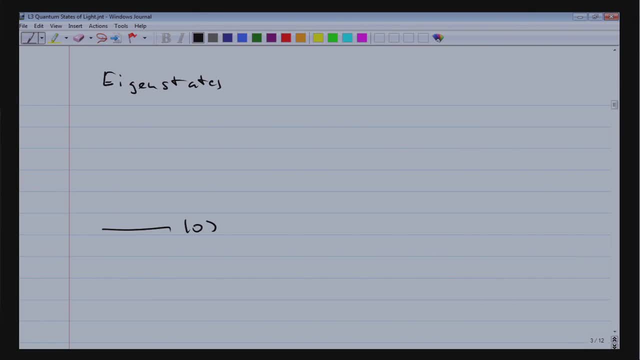 So quite often we don't want those states, We want coherent states. But we need those number states as one representation. So let me just introduce them. So we label by n the states with n photons And the energy of those states is n plus 1 half h by omega. 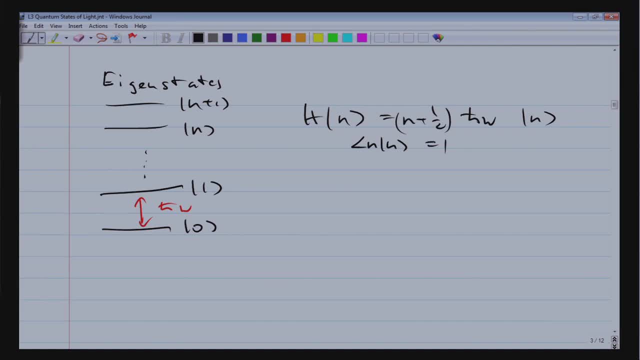 The states are normalized, Sometimes out of laziness, because it doesn't matter. we can eliminate the 1 half. It just makes some equations more compact, And if I do that, I can write The Hamiltonian like this: You are familiar, of course, with commutators. 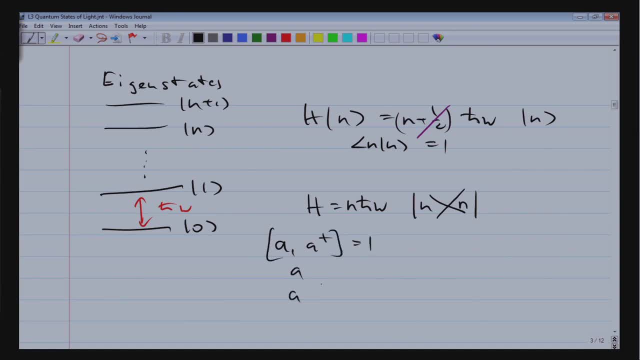 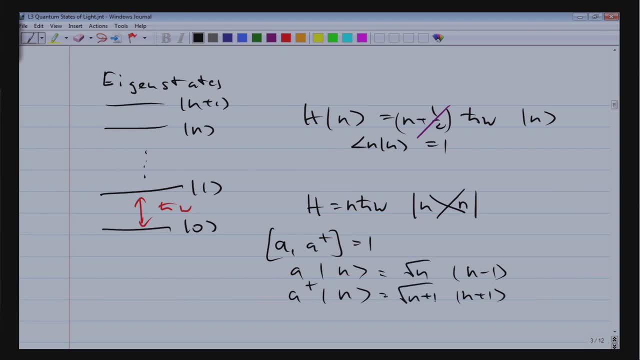 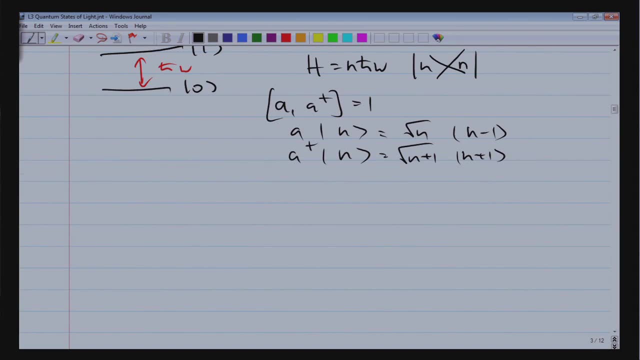 OK, OK, OK, OK OK. This was a short review of the simple harmonic oscillator as it applies to a single mode of the electromagnetic field. Now, just as a short example, in subsection 2, we want to discuss the thermal state. 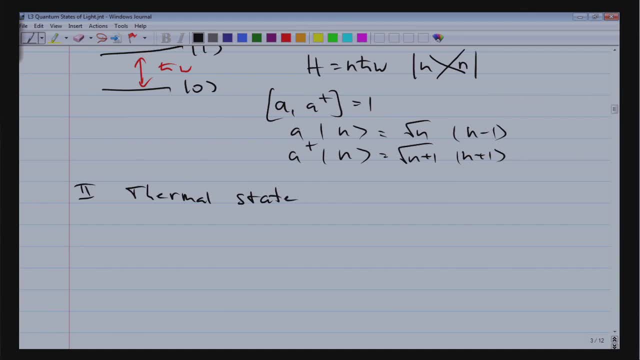 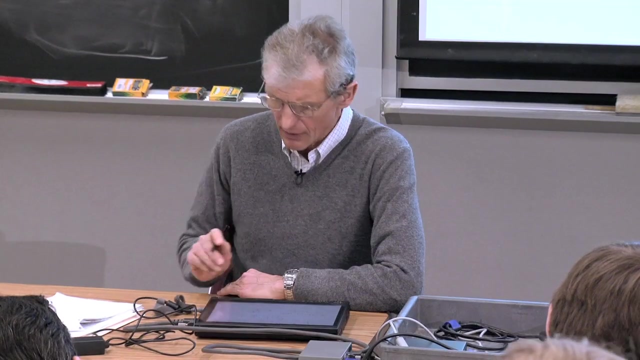 And the thermal state is nothing else than photons. in a black body cavity We have a photon field which is in equilibrium at temperature T. So if we use the canonical ensemble, our statistical operator is given by this well-known expression, And if I use, I mean that's all. 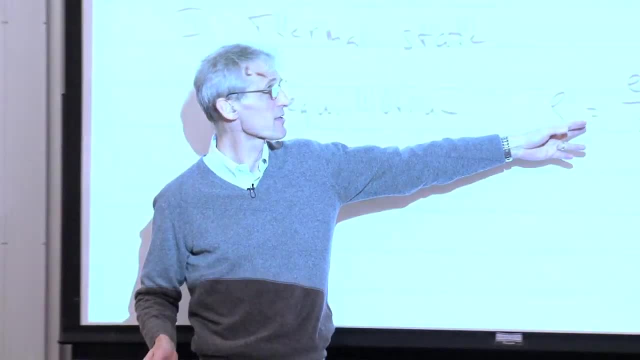 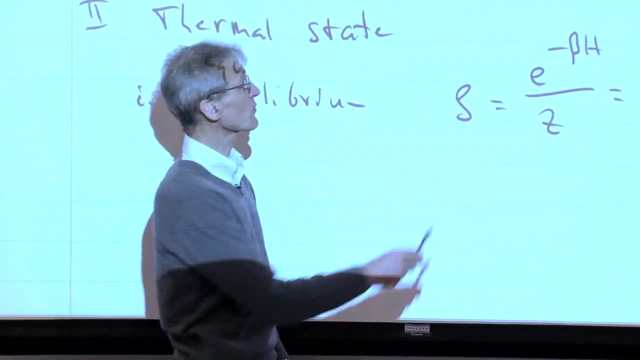 I mean, isn't it wonderful, once you're trained in statistical mechanics, this is all you have to know about a thermal state of light. That's it. This is the Planck law. All we have to do is take the Hamiltonian, which. 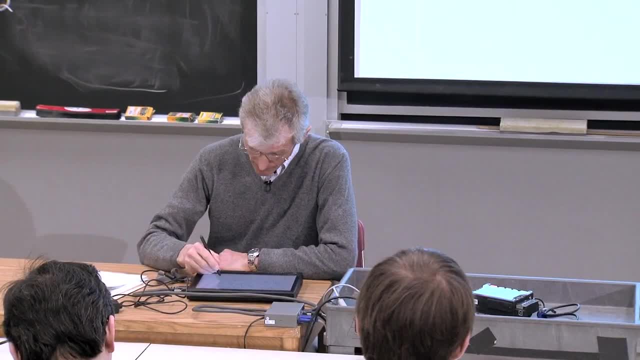 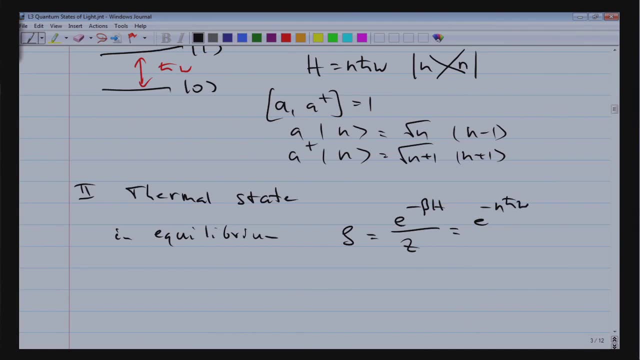 we have written down upstairs. So this is e to the minus n photons n times h. bar omega is the energy over kT divided by the partition function. This is the density matrix, the statistical operator for single mode light in thermal equilibrium. The partition function is very simple. 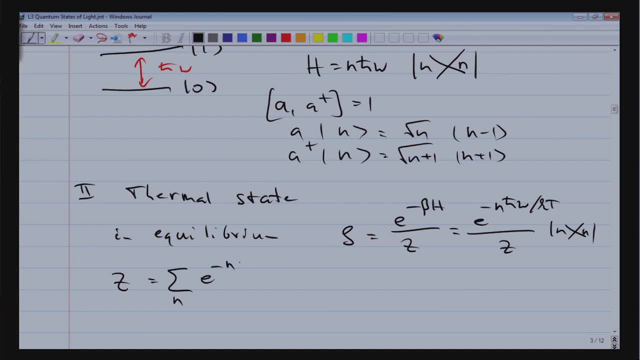 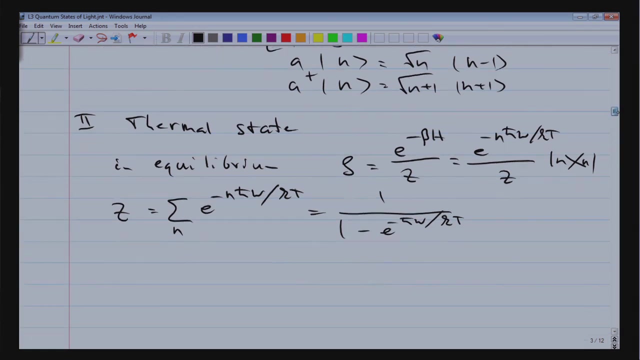 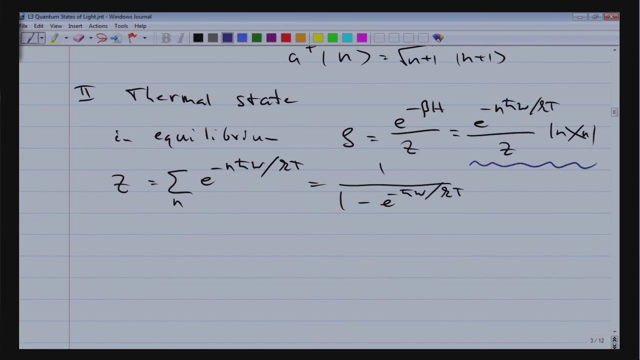 because this sum over all Boltzmann factors is a geometric. It's a geometric series which can be simply summed up in this way: divided by kT. So therefore this expression here can be written as the density matrix in thermal equilibrium. 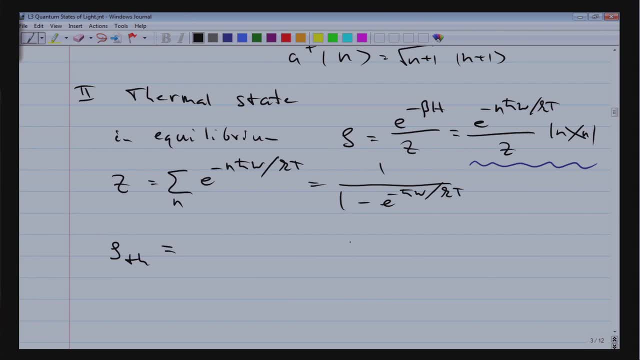 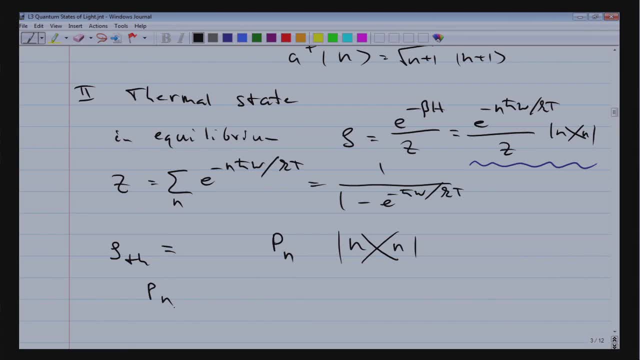 And the probability for n photons is given. here We've evaluated the partition function. So then, if you put it together, we simply get this- You can call it Bose-Einstein factor- which tells us what is the probability to find an harmonic oscillator with n quanta. 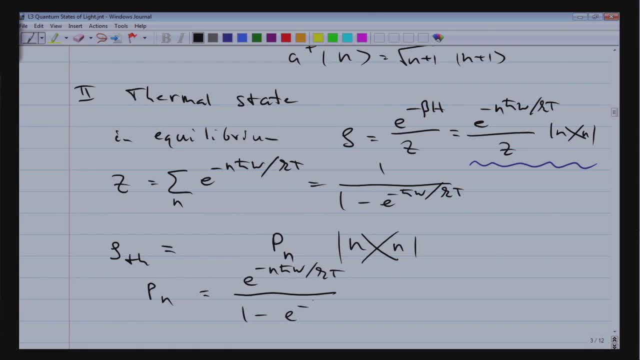 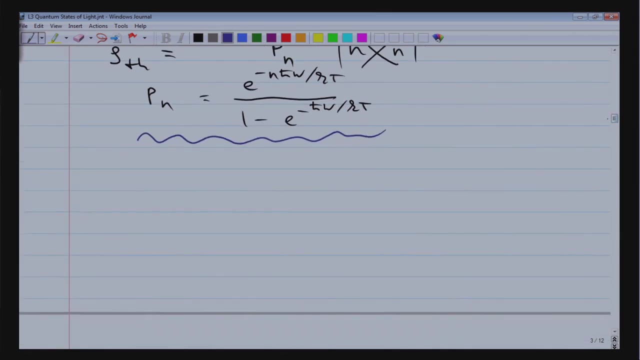 And this is the expression e to the minus h bar omega. This result takes care of many situations, actually almost all situations you find in every day's life, unless you switch on a laser pointer. So this describes an resistive filament. It describes the light generated by gas discharges. 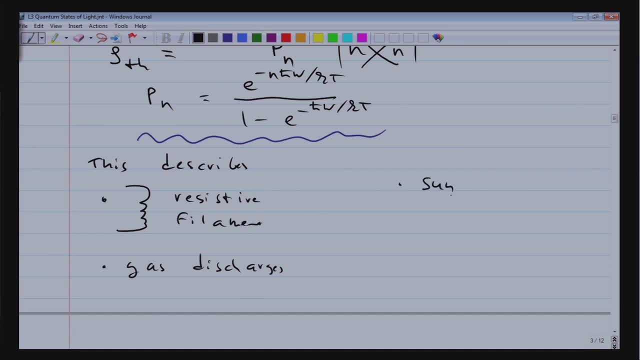 It describes the light of the sun And this kind of thermal light because it has the maxi- I mean light in thermal equilibrium. thermal equilibrium is maximizing the entropy under the given boundary condition. It's also called chaotic light. It's just another name for thermal light. 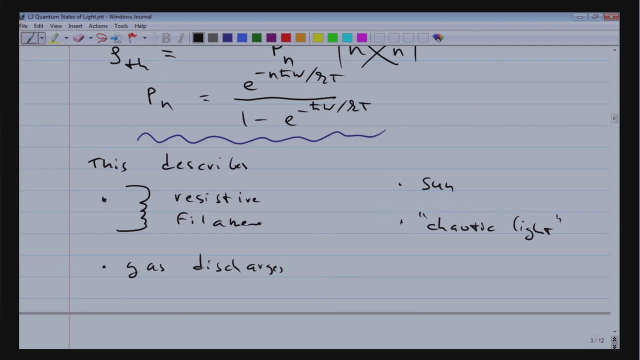 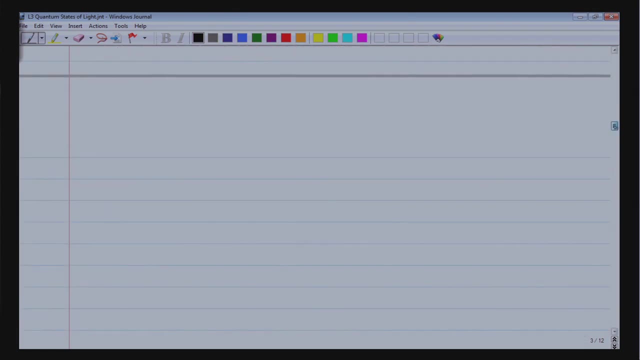 So well, you should now lean back and take the attitude. if I know the statistical operator of an ensemble, I know everything about it. I know that every quantity on the interested in can be calculated. So, just as an example, we know what is the probability. 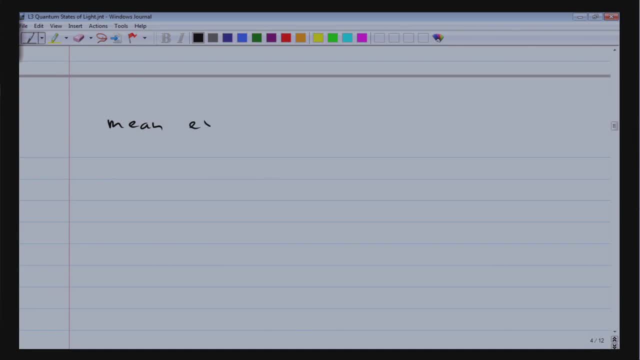 to find n photons. But now we want to ask: what is the energy density, or what is the mean excitation number, what is the average of n? So? So for that we have to take the number operator: a, dagger a. 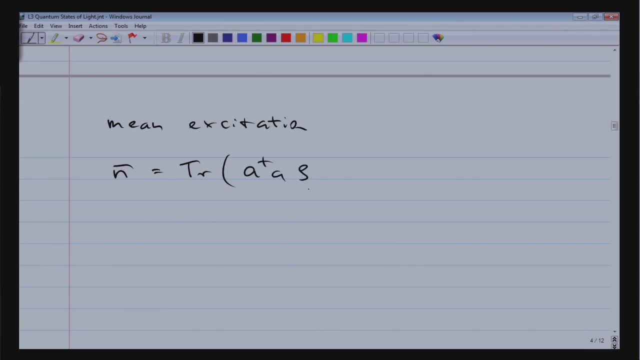 and perform the trace with the product of the statistical operator, And this is of course nothing else. Then we look for the probability to find n photons, And this probability is weighted with n, And what we get is a very simple result. 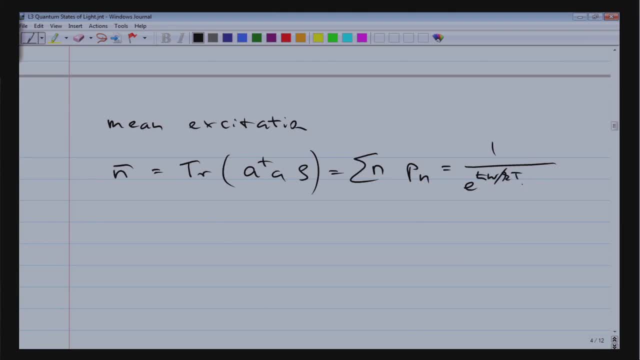 It's the Bose-Einstein distribution law with a chemical potential of 0,, which is the familiar distribution. We can now use the quantity n to rewrite our previous expression for the probability to find n photons in thermal equilibrium. It is n bar to the power n divided. 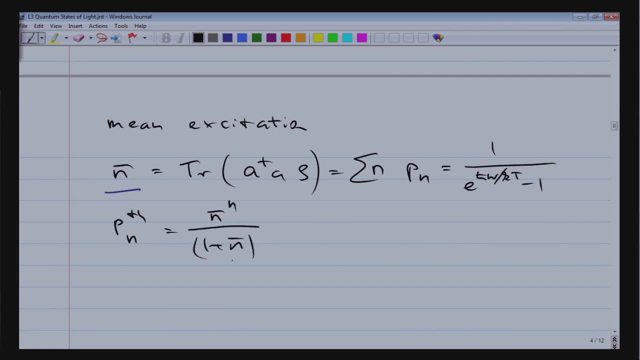 by 1 over n bar times, n plus 1.. So all of this should be very familiar to you And I'm not doing the final step. but I could immediately get Planck's law now All I have to use it. sum up now: 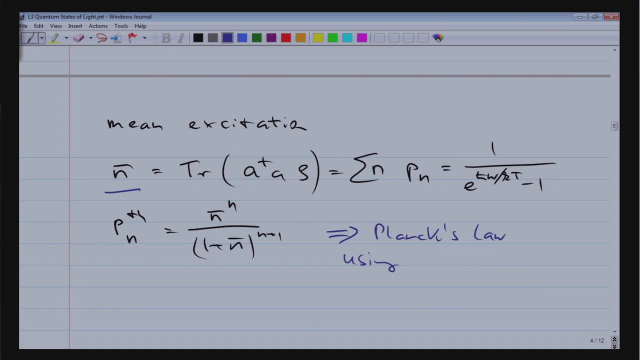 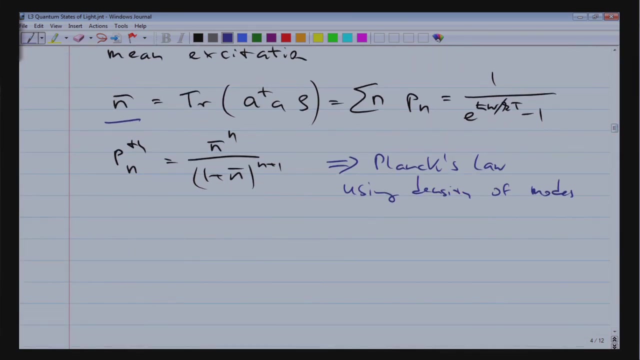 This is a single mode of light, single monochromatic light. All I have to do- I used to get Planck's law- is to sum over all modes using the density of modes. Any question, We will not be talking a lot in this course. 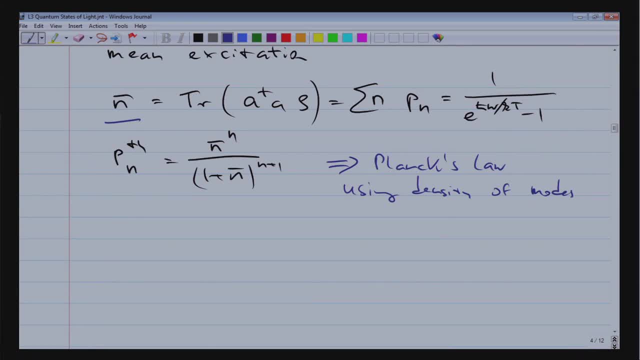 about chaotic and thermal light, Because we are mainly interested in the purer form, how atom interacts with light, And this will be when light is in a more specific state, not in a thermal ensemble, in a more specific state, which are number states or coherent states. 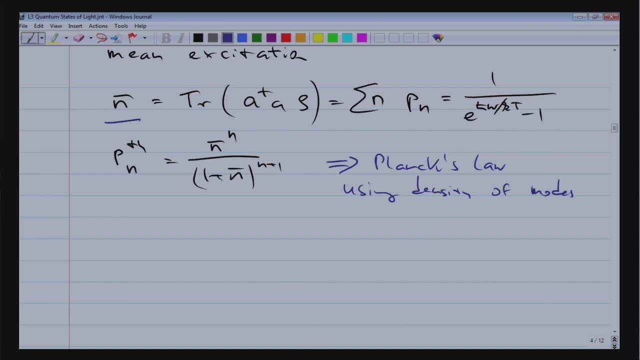 But nevertheless, I feel if I don't tell you a little bit about ordinary light, you will not be able to appreciate quantum light. So I want to use this example now of a thermal distribution of light and write down for you in the next 90 seconds. 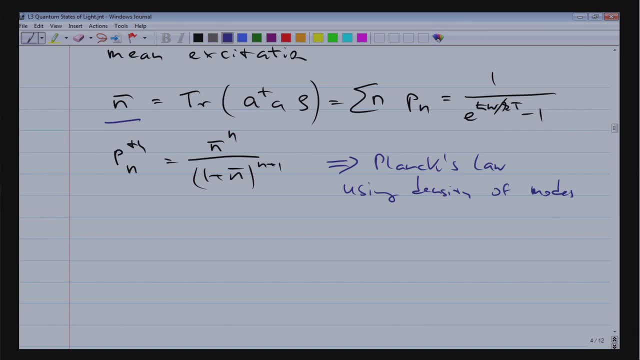 expressions for the fluctuations. So you should know a little bit about what is the statistic of thermal light. If you find n photons in a black cavity and you look again, is the variance in the standard deviation of the photon number square root n? is it Poissonian or is it much larger? 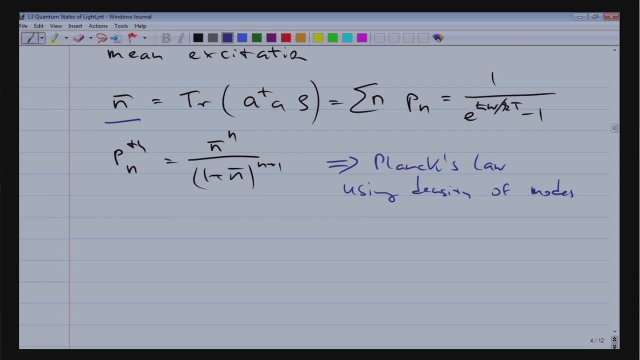 So you should know about that, Because it will then make a difference when we talk about the purer states of light, coherence, even states and number states, quies states and all that. OK, So we want to look now at fluctuations. 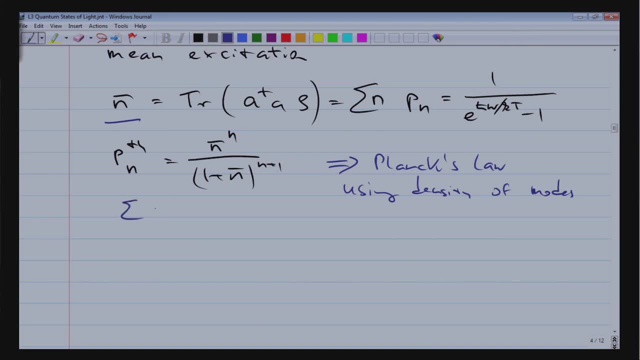 Let me just first mention that we have normalized correctly the probabilities, Just one second. What we are interested now is What are the fluctuations? So we want to know the variance, We want to know what is delta n squared, And delta n squared is of course n square average. 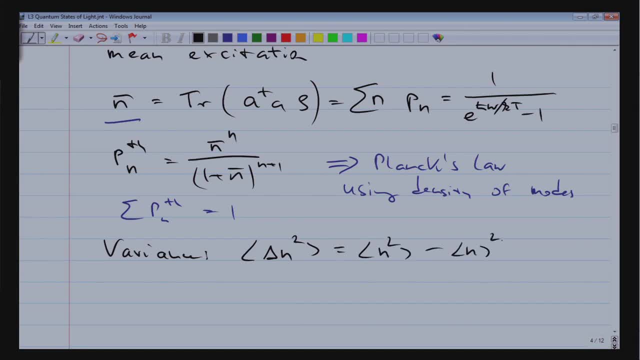 minus n average squared, And we want to find out what is that for thermal light, for chaotic light? What we need now is we need an expression. We have already an expression up there for n average, And now we need an expression for n square average. 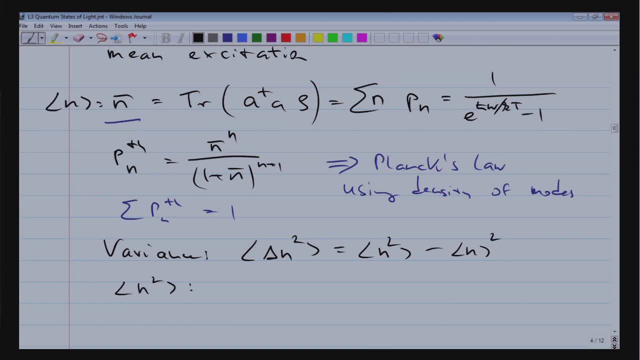 We can get that as follows: If We take the probability, multiply it with n, n minus 1, sum over. Sorry, I have a brain cramp. This equation is in my notes, But I don't Maybe step back. 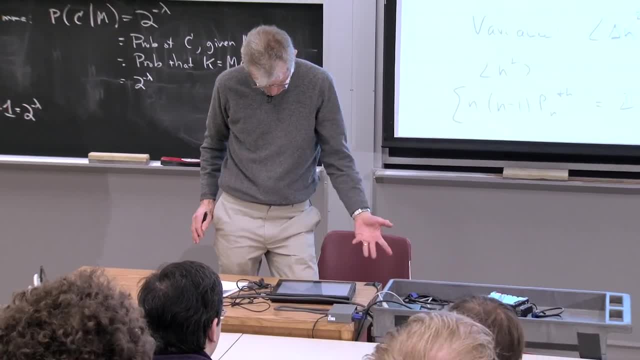 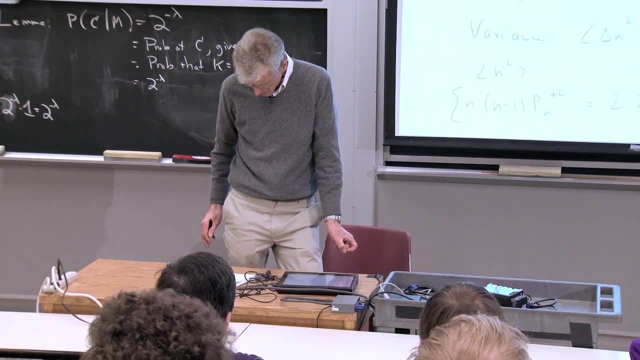 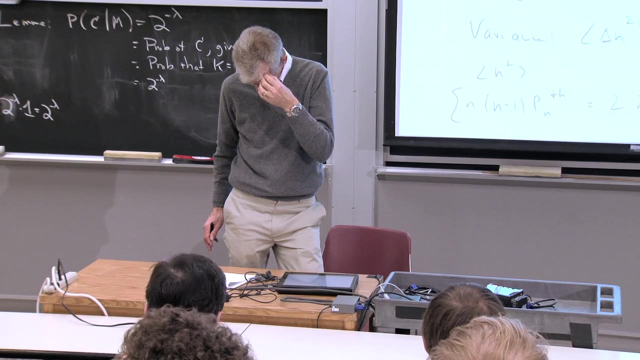 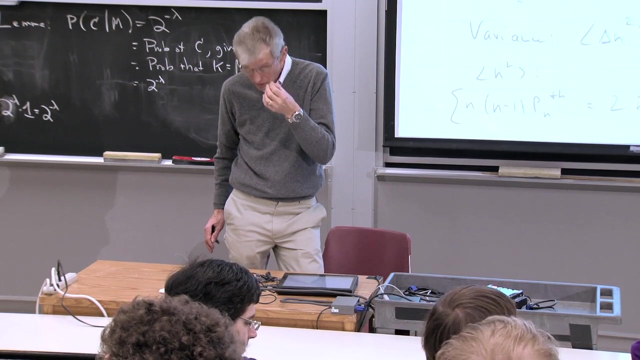 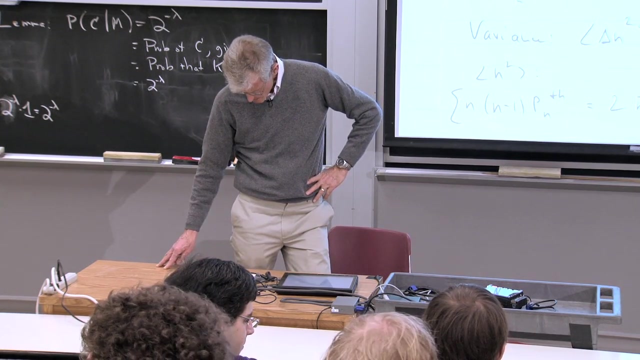 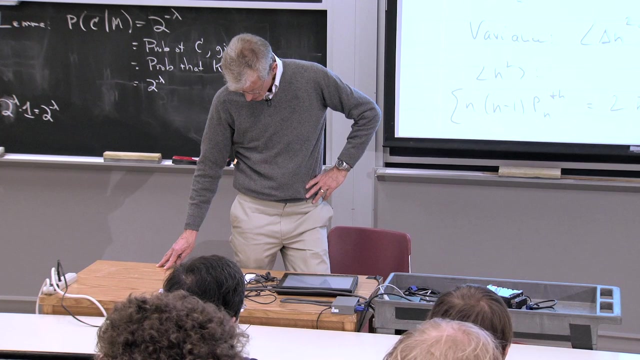 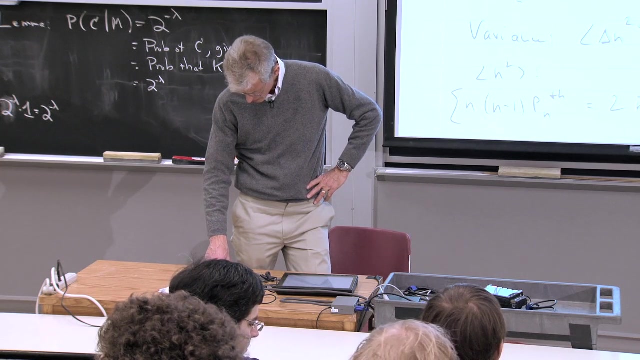 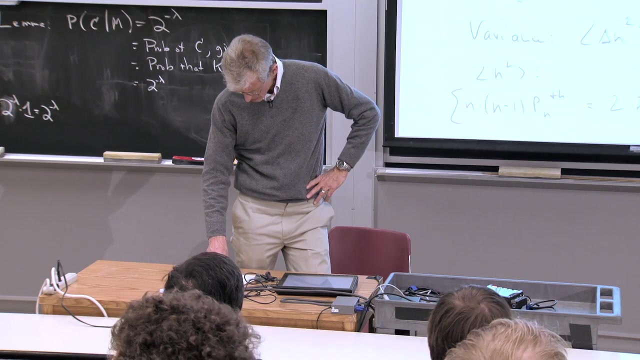 I don't see where it comes from, But from this expression, of course we have now an expression for n average squared, The sum over it. Just a second. Just a second In thermal n average squared Anyway. 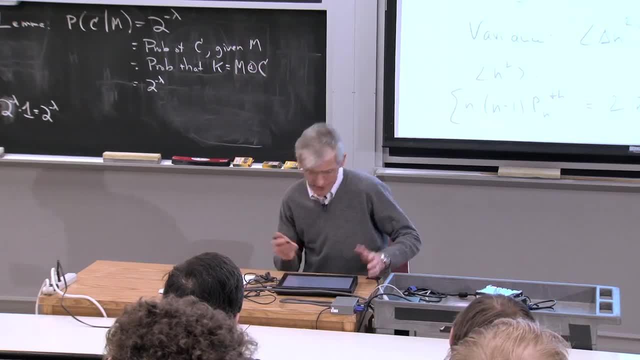 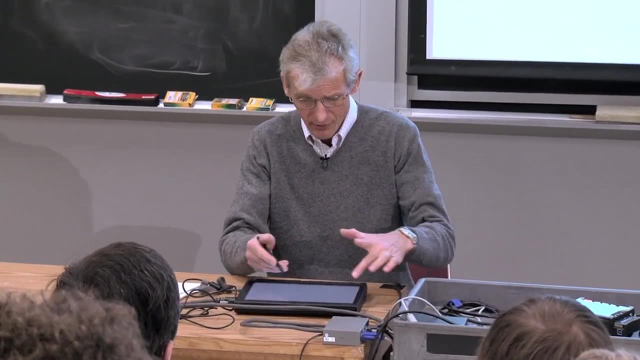 I don't want to waste class time. It made sense to me when I wrote the notes. I just can't reproduce the argument, So this should be obvious. It's not obvious to me right now, But let's just take it and run with it. 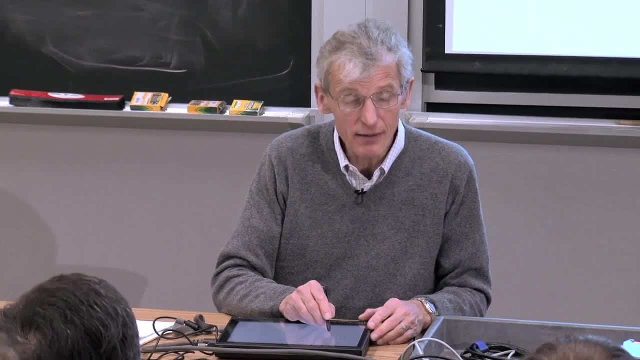 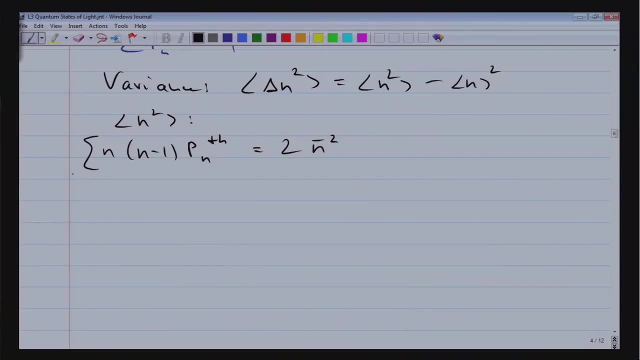 The left-hand side has n square minus n multiplied with the probability. So let me just take a note. I will show you where it comes from on Monday. But assuming that it's true- and I know it is true- that actually contains n square average minus n squared. 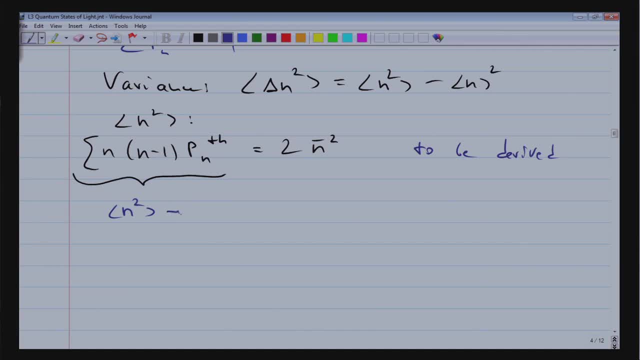 n average is 2n average squared. So therefore we have now our expression for the average of n square, which is 2n average squared plus n average. 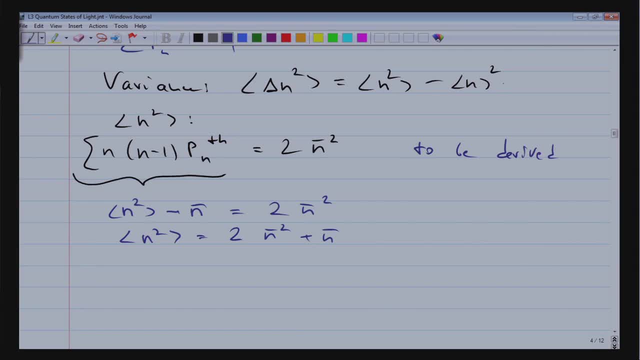 Therefore, for thermal light, for chaotic light, the variance delta n square is an average square plus an average. So the question is, if this is our variance, the variance of thermal light, of chaotic light, is that? What you should see immediately is: 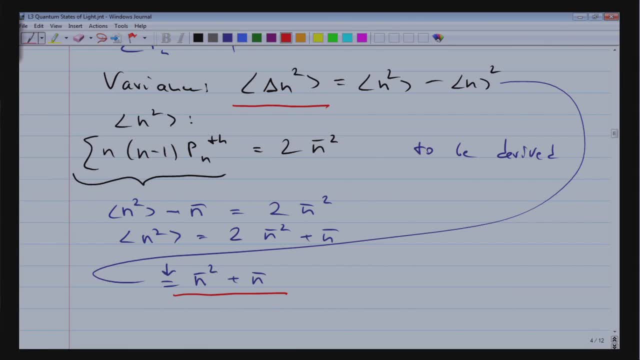 that it is much more fluctuating than Poissonian statistics. If you compare now with thermal light Poissonian statistics, Poissonian statistics would have fluctuations where well the rms fluctuations are square root n The variance is just an average. 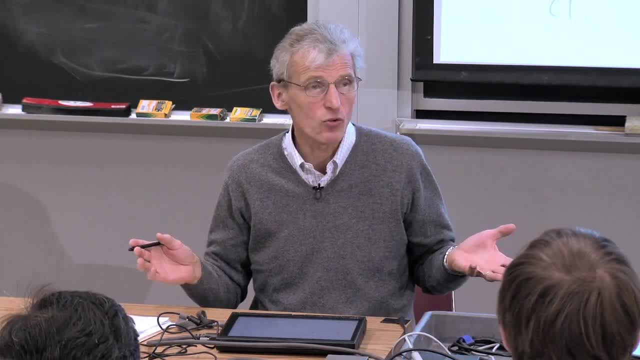 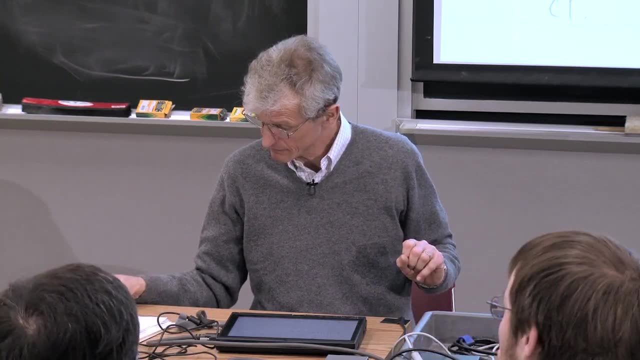 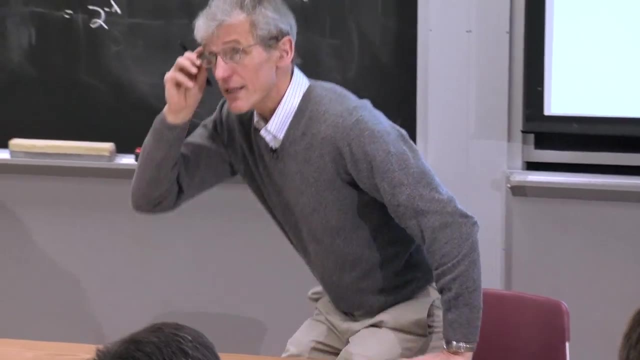 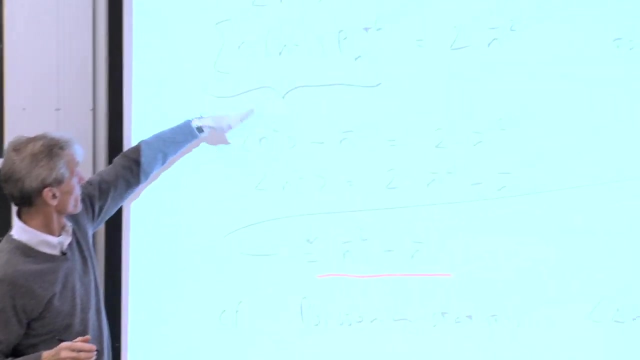 So thermal light is suitable. Super Poissonian has much, much stronger fluctuations in thermal than Poissonian distribution. OK, One question for you, If you look at the distribution of photons- and we have written it down here. Let me just scroll up. 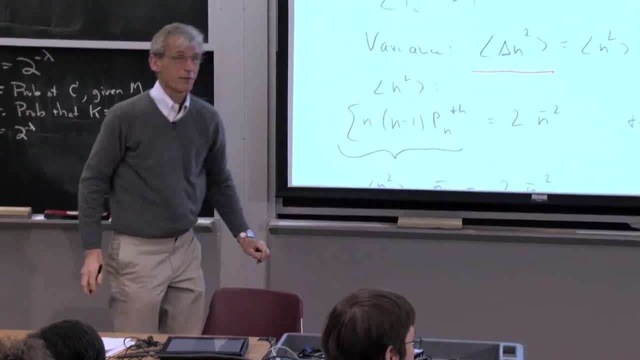 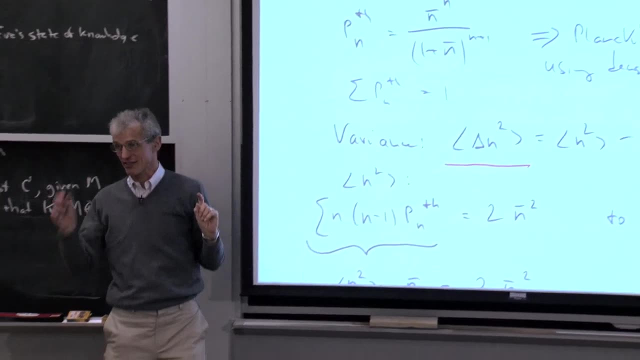 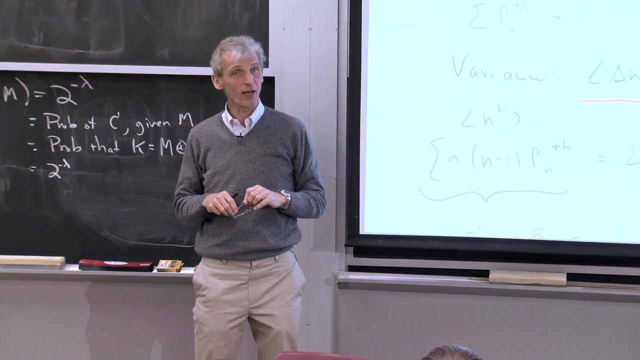 This is the well. You probably don't have an auto-plot function in your brain, but if you plot this function and I'm asking you what is the most probable photon number you will find for light in thermal equilibrium? 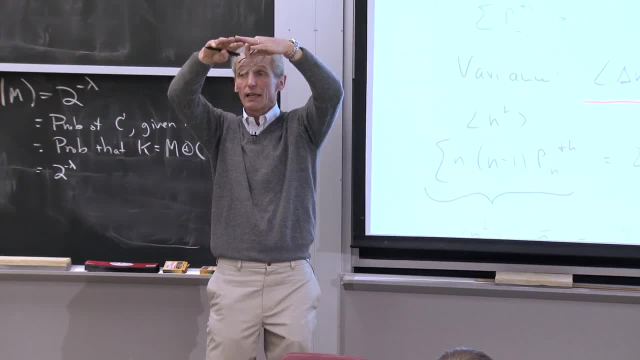 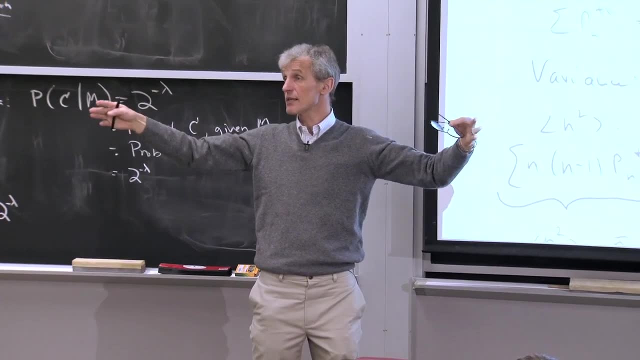 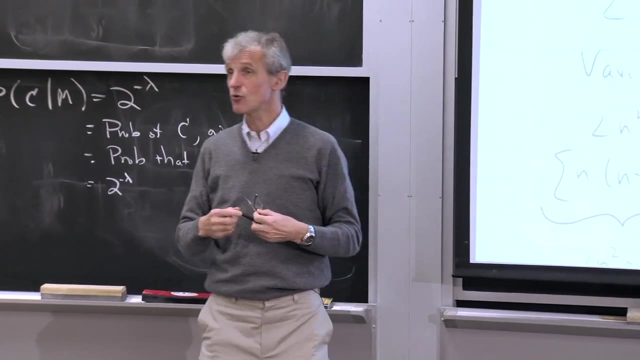 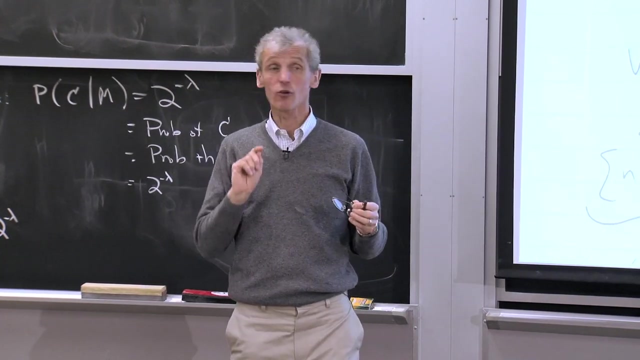 Zero Zero. It is a broad Gaussian centered at zero. So you have a broad Gaussian. The average photon number is related to the width of the Gaussian. But the nature of thermal light is that whenever you look into a black body cavity and ask what is the most probable photon number, 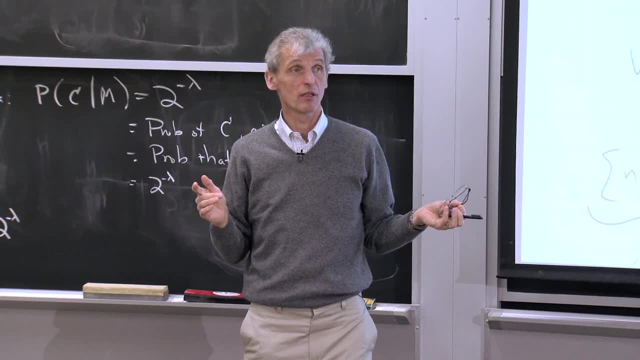 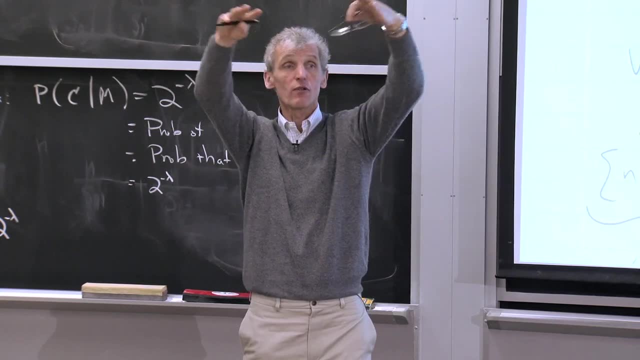 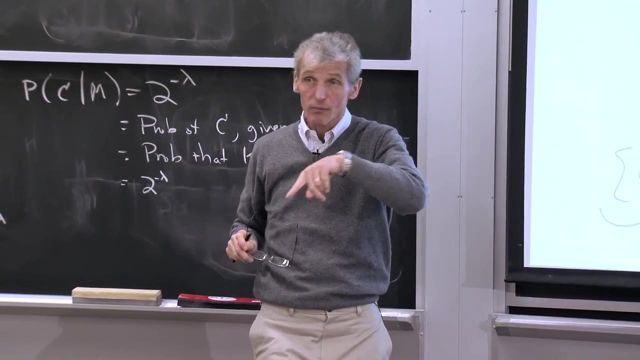 for any mode, it is actually zero. No matter how hot the cavity is and how many photons you have in it. The photon number distribution is always a broad Gaussian, With a maximum at zero. We'll come back to that later, when. 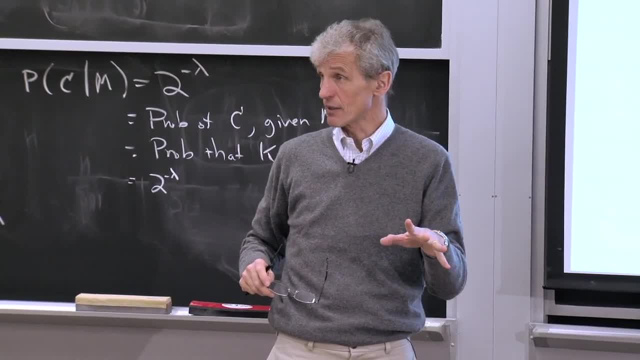 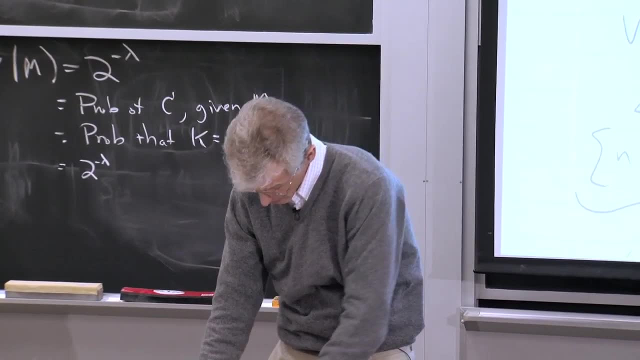 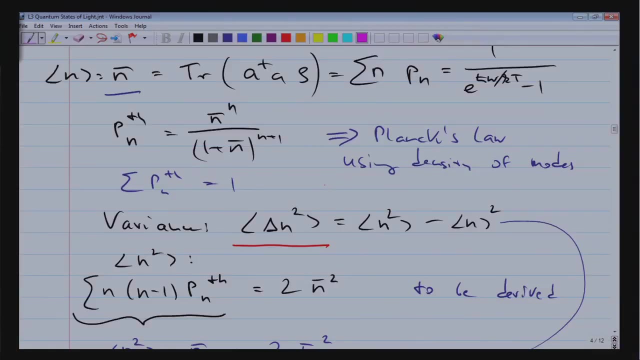 we talk about coherent states, Then you will appreciate the difference. But I will be referring back to the result we have just derived for the photon number distribution. Let me just take a note: The most probably n Is. n equals zero, OK. 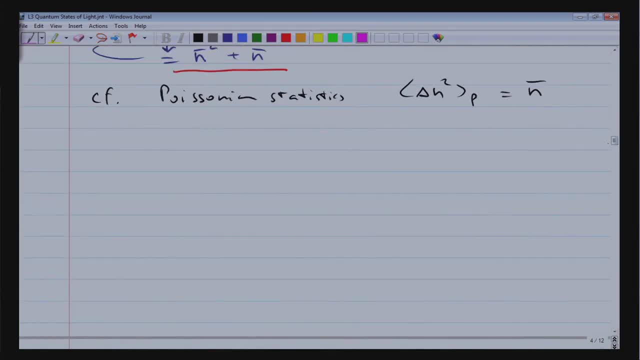 I hope with that- and this is Roman 3, the third subsection- you can really appreciate the properties of coherent states. Coherent states were introduced by Roy Glauber in 1963.. It's actually something you should wonder about. 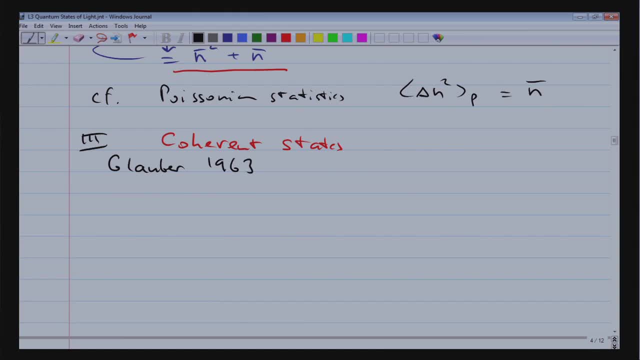 Coherent states seem so natural. We teach it in all courses And when we think about harmonic oscillator we often think in terms coherent states. But they were not immediately used and invented. when quantum mechanics was invented in the 30s, it really took somebody like Roy Glauber. 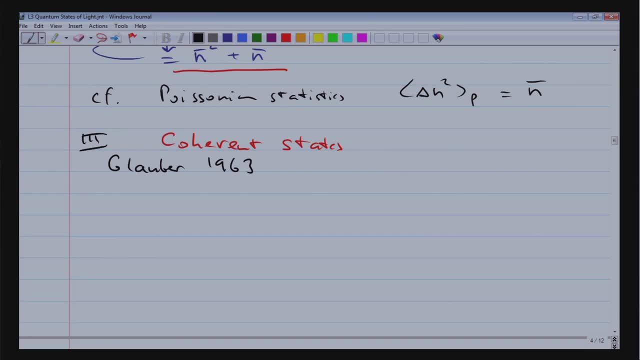 to invent coherent states, And that happened in the 60s. Maybe the reason why people didn't immediately jump at coherent states is because coherent states are not eigenstates of a Hamiltonian. The definition of a coherent state is actually an eigenstate, not of a Hamiltonian. 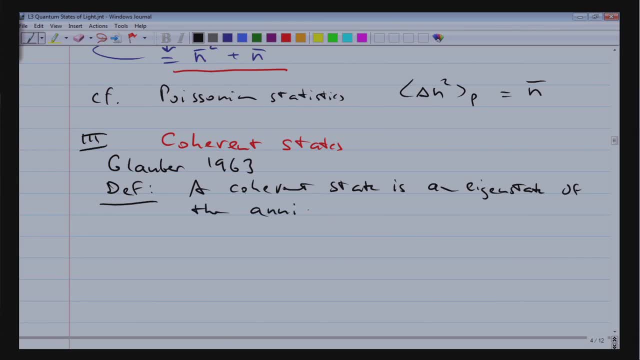 It's an eigenstate of the annihilation operator And of course the annihilation operator is non-Hermitian, So it's a strange operator to look for eigenstates. But this is what defines the coherent state, namely that A acting on a coherent state. 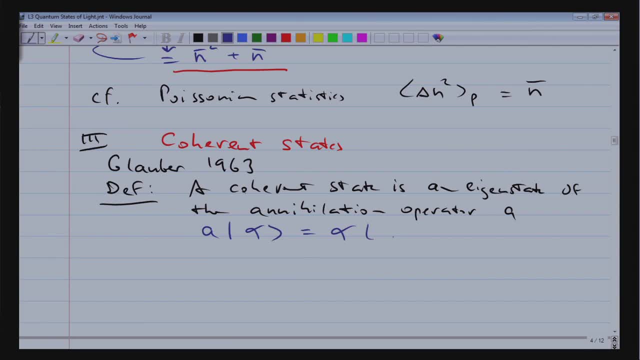 alpha equals alpha times alpha. I'm using here the standard notation that alpha is both the label for the coherent state written down here and is also the eigenvalue of the coherent state when acted upon with the annihilation operator. We normalize those. 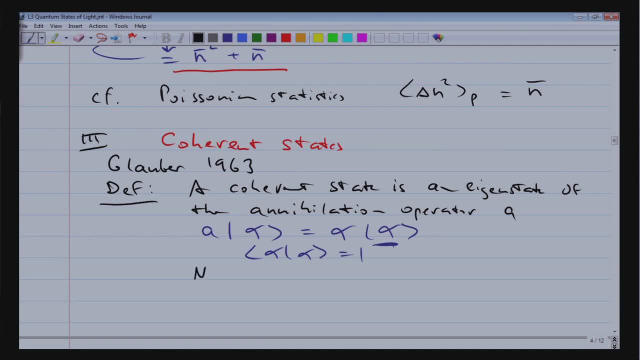 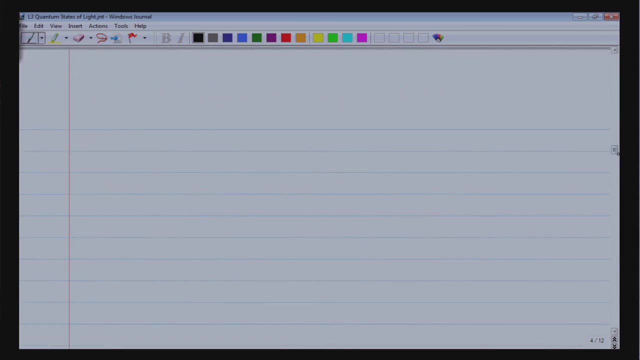 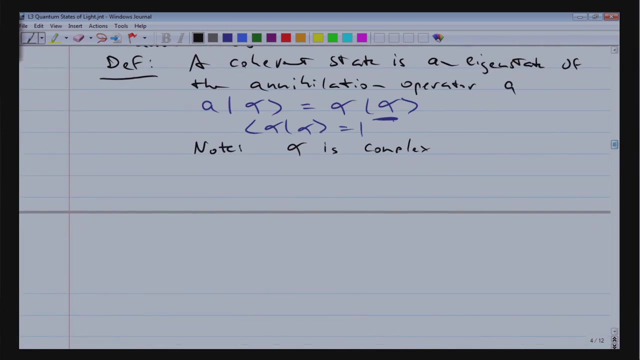 We normalize those states. And since we're talking about eigenvalues of a non-Hermitian operator, alpha can be any complex number, OK. so now we have introduced a second set of basis functions for light. Remember we had the basis functions. 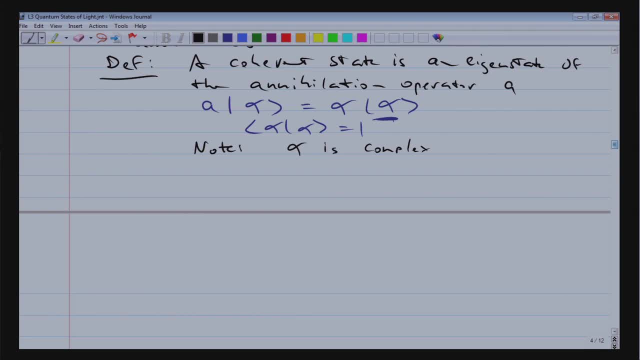 n, the eigenfunctions of the harmonic oscillator, And now we have defined a new set of eigenfunctions, the coherent state alphas. Of course, the next obvious question is: how are the two representations connected? So what we want to do now is we want to figure out. 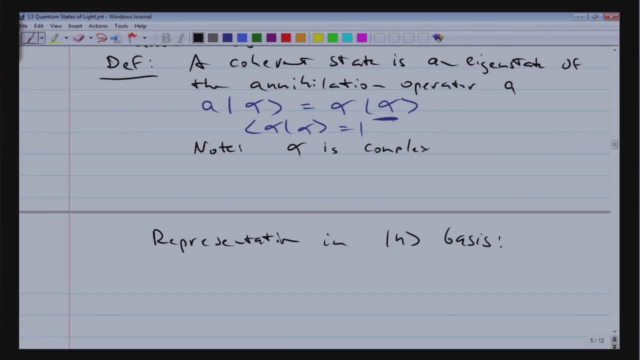 how do we write a coherent state alpha in the n basis, in the basis, OK, OK, The basis of eigenfunctions of the harmonic oscillator. So we want to write this is just want to expand the coherent state into eigenfunctions n. 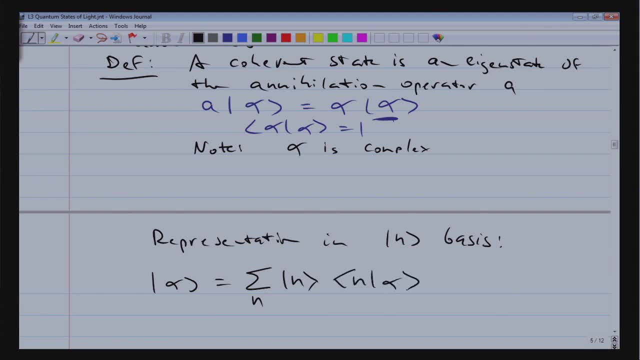 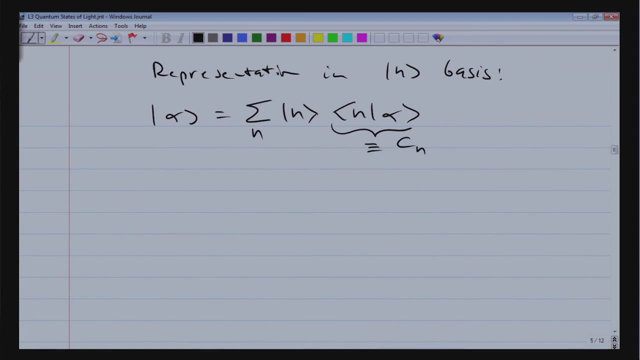 So the coefficients we want to calculate are those matrix elements which I define as cn. So what we have to use is, in order to find this representation, we have to use the fact that alpha is an eigenstate of the annihilation operator. 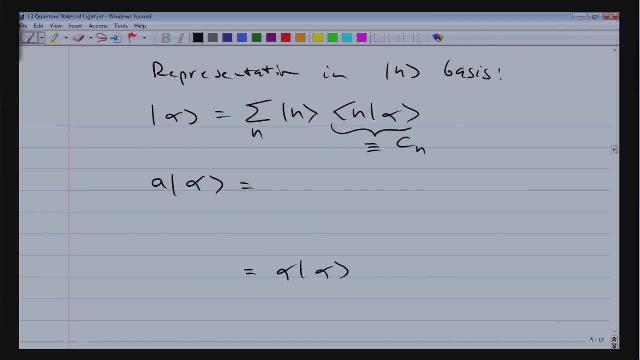 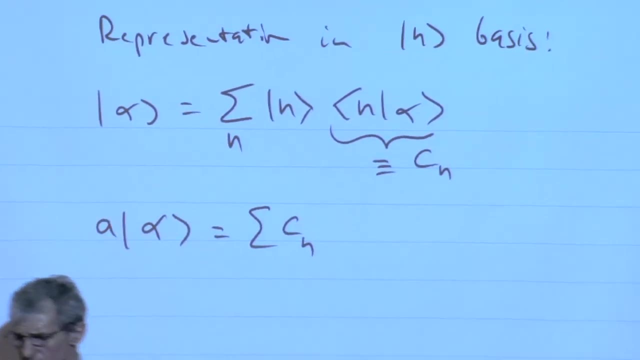 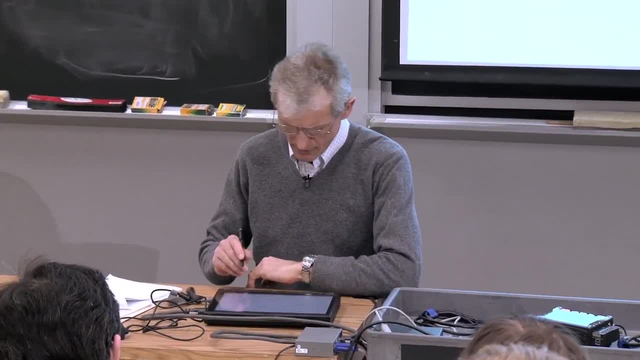 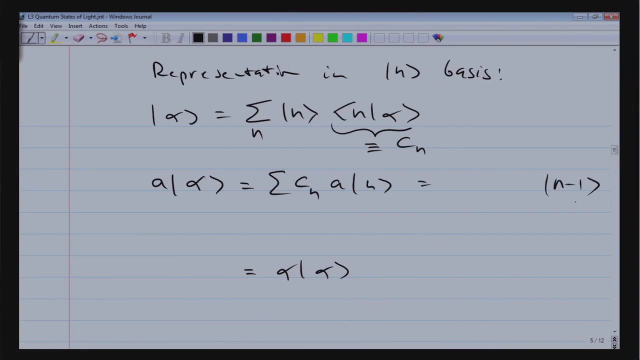 And the annihilation operator, of course, does what it is supposed to do: It lowers the photon number by 1. And we get the matrix element square root n, And then, by just changing the summation index by 1, we can write it as n times cn plus 1 times the square root. 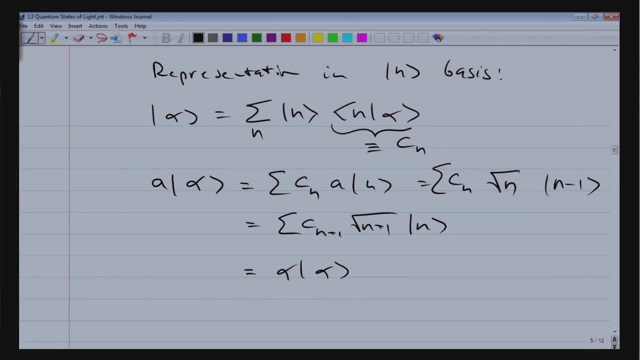 of n plus 1.. So this is when the annihilation operator acts on the sum. And now I continue with a lower line, which is alpha cn times n. So what I've found now is I've found two ways to write the same state, namely a acting on alpha. 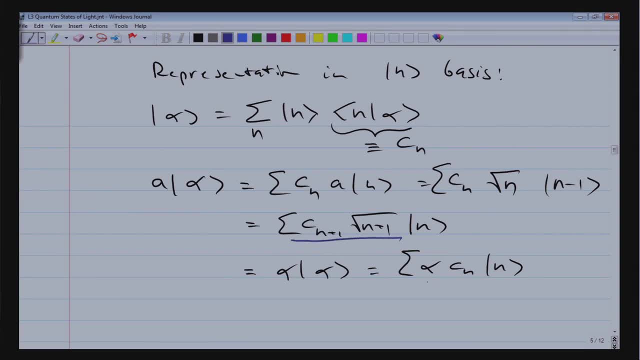 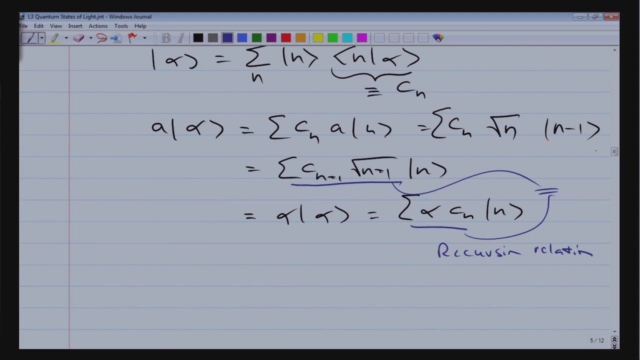 And therefore those coefficients have to be the same. And what I just indicated in blue is a recursion relation which expresses cn plus 1 by cn. So every time you go from cn to cn plus 1, you multiply with the square root of n plus 1.. 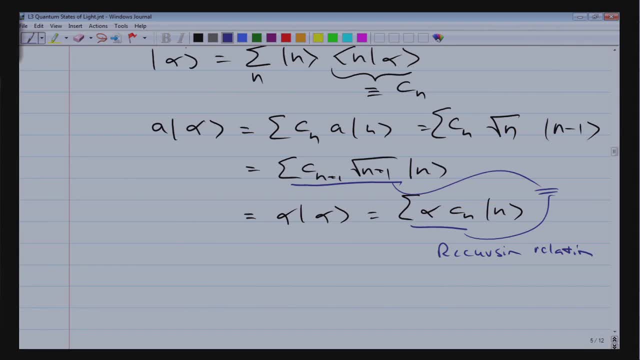 So if you stare at it for a moment, you find that cn is related to c3.. And c3 is 0.. Yes, cn plus 1 by alpha n over n factorial. OK, OK, OK, OK, OK, OK. 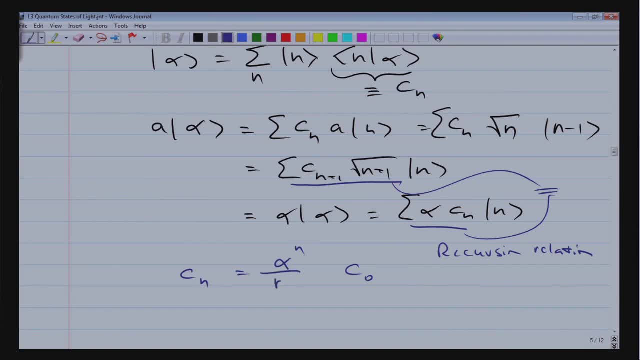 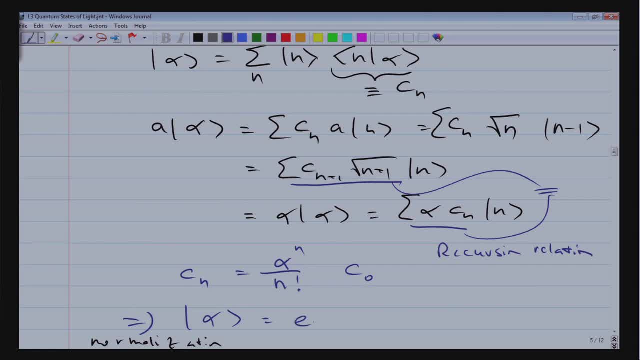 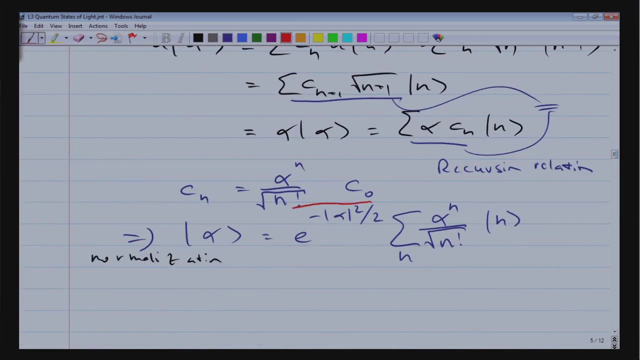 And then we get as a final result the normalized representation of the coherent state in terms of number states. Excuse me, I think the square root is missing here, because it appears here times n OK, so what we have found here is now. 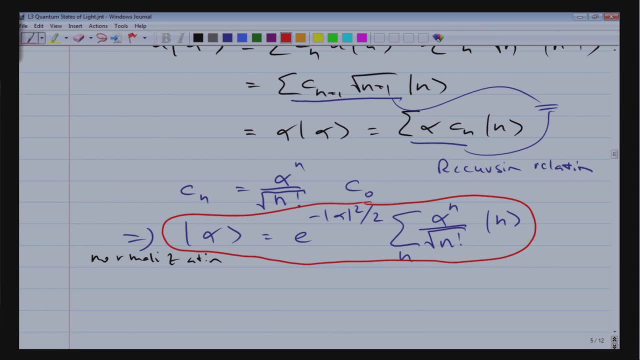 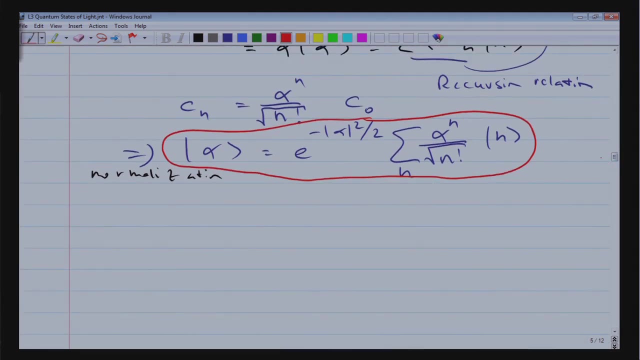 how coherent states are written down in the number state basis. So now we know coherent states and we can ask a number of questions. So what is this? So what did we define and what have we now derived? Let's look at some of the properties. 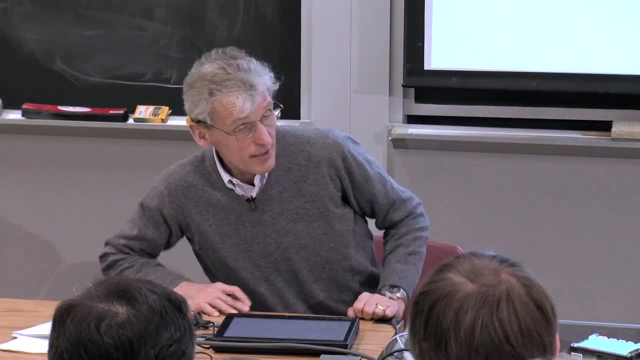 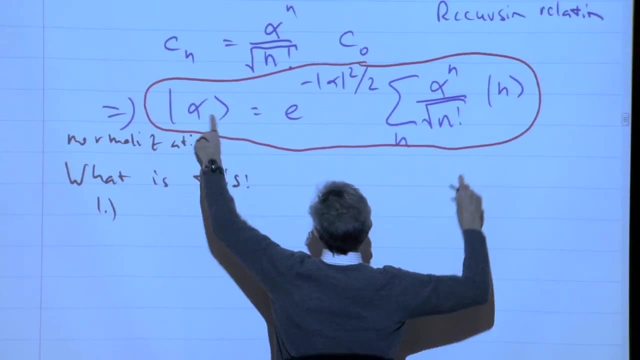 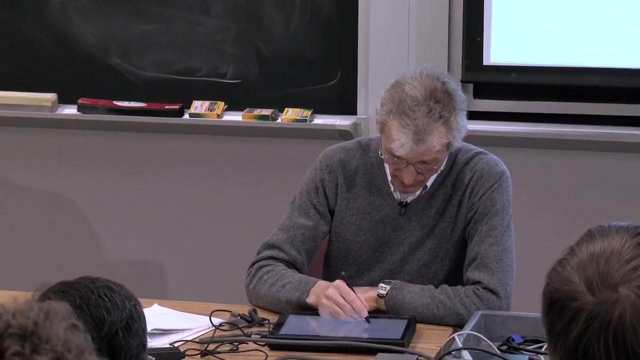 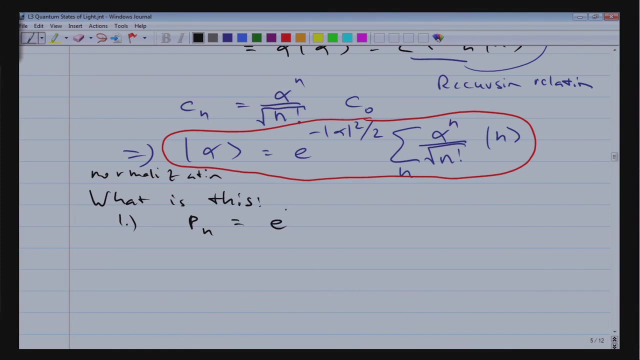 The first one is that if we look at this expression, this is the amplitude that we have n photons in a coherent state. The square of the amplitude is the probability. So the probability to find n photons is, let's say, the square of the amplitude above. 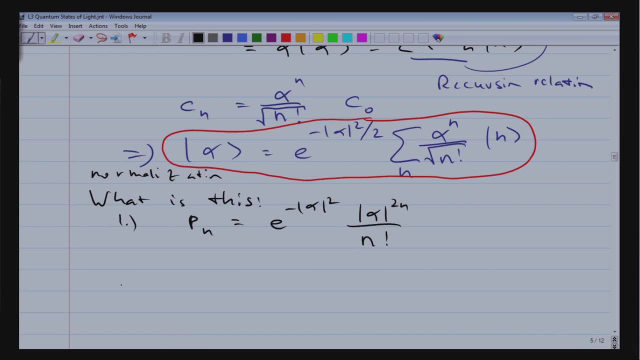 So this is that, And this is now a Poissonian distribution. So it's immediately clear that those coherent states have much, much smaller fluctuations in the photon number than the And the thermal state we discussed before, Because this is Poissonian, whereas the thermal state 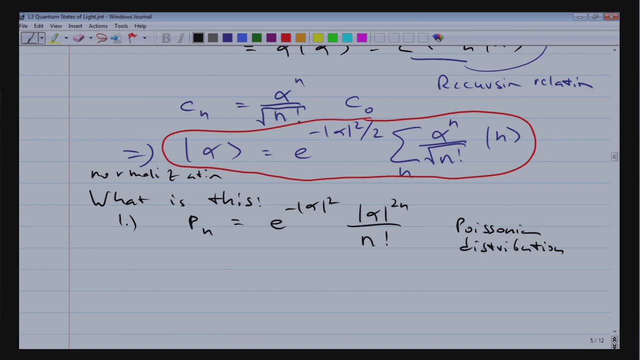 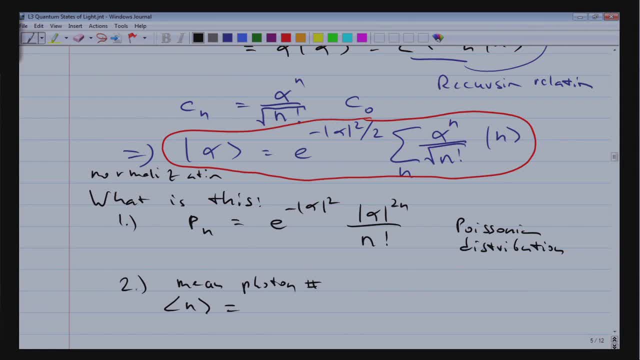 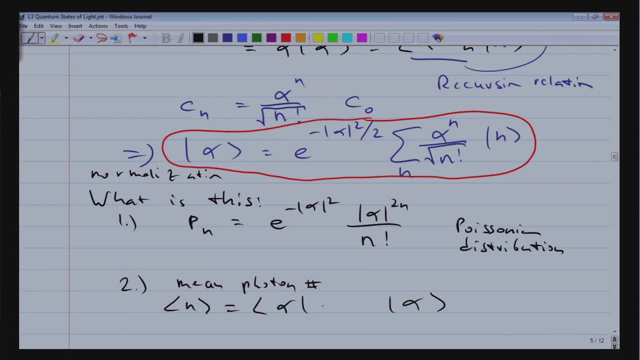 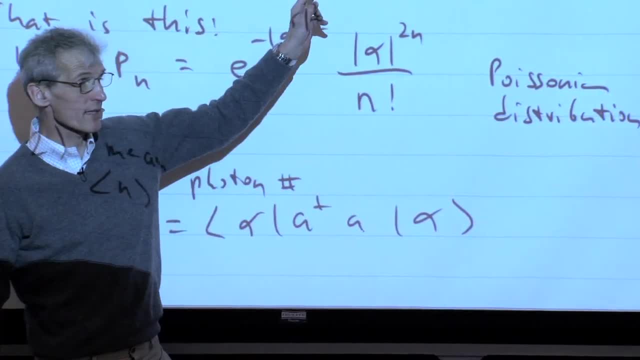 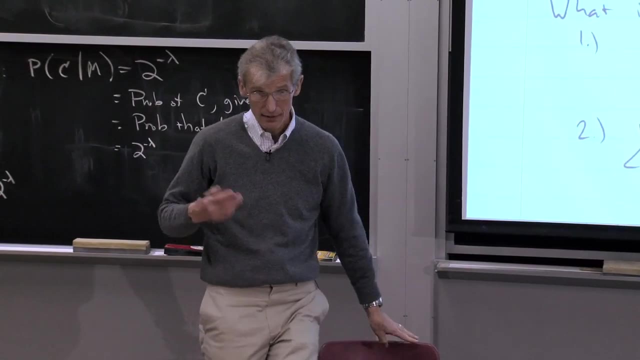 the coherent state And the photon number operator is a dagger a. And now you see, hey, we are lucky, because a acting on alpha is just getting alpha, But a dagger acting on alpha on the left-hand side gives us alpha star, the complex conjugate. 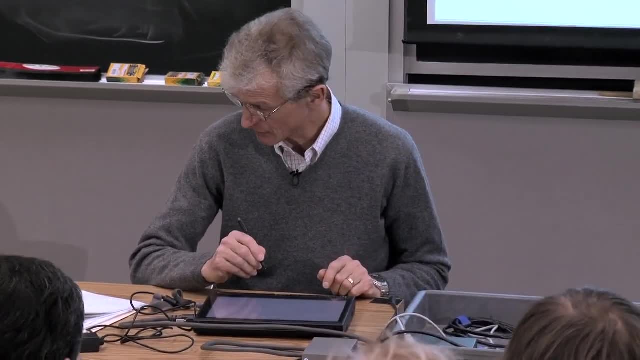 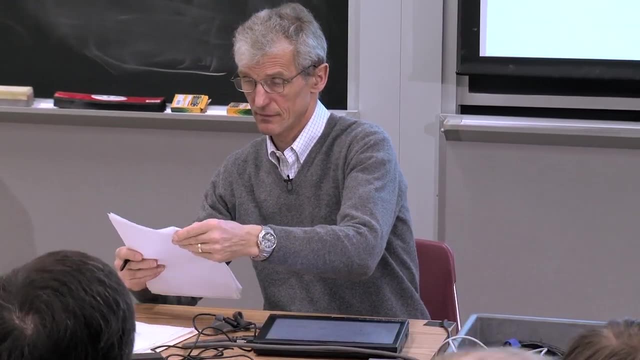 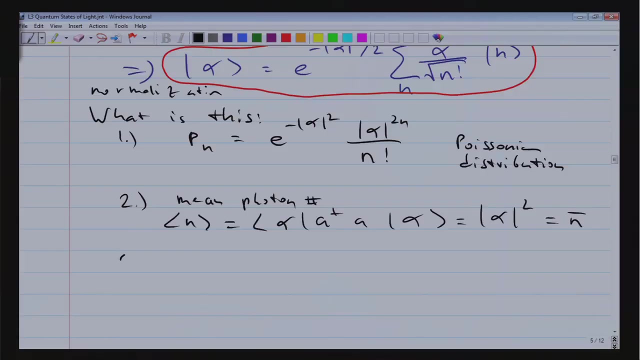 So what we obtain here is simply the absolute value of alpha squared, And this is our expression for the average photon number. I have already mentioned that the variance must be n because it's a Poissonian distribution, But since it is so nice to have creation annihilation operators, 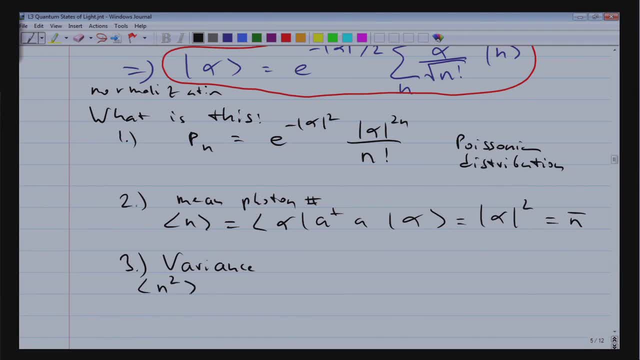 as acting on coherent states. let's just calculate. Let's verify that we know the distribution is Poissonian, But let's verify directly that the variance of the photon number in the coherent state is n is Poissonian. If you need the variance, we need an average. 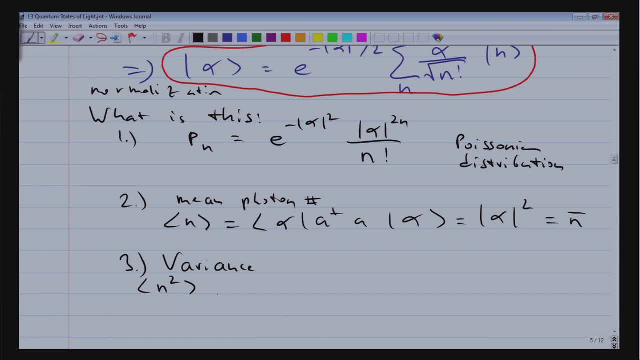 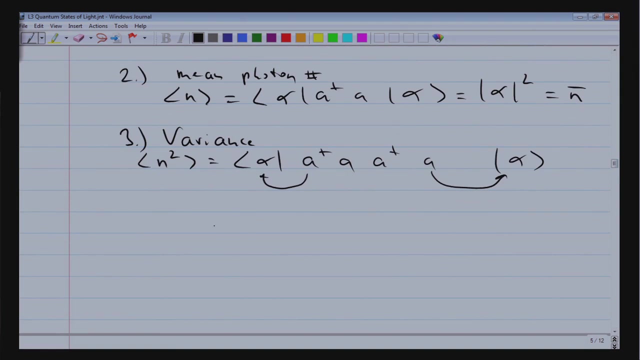 And we need n square average. Let's just calculate n square average. So we need now the operator for n square, which is a dagger a, a dagger a. We know already, if those two operators act on the bra and the ket, that this just. 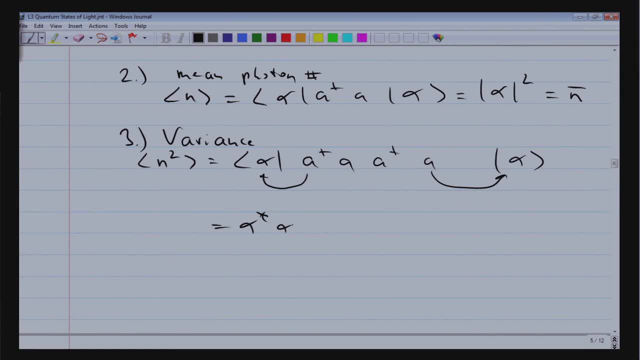 gives us alpha, star alpha, And then we are left with a alpha a, a dagger. Now a dagger acts on alpha. We don't know what a dagger is acting on alpha. We know that alpha is an eigenstate of a, but not of a dagger. 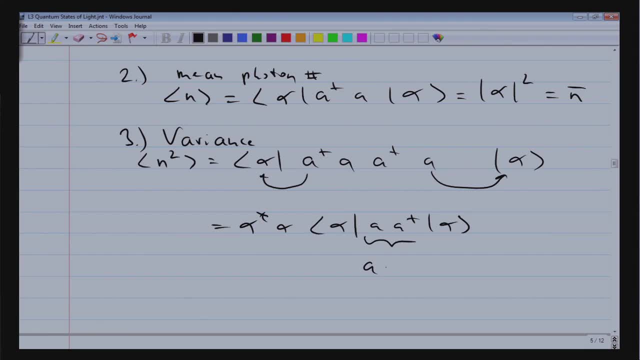 So therefore, we want to change the order of a and a dagger Use the commutator, And then, of course, a dagger can act here, a can act here, a can act here, And we just get another factor of alpha. 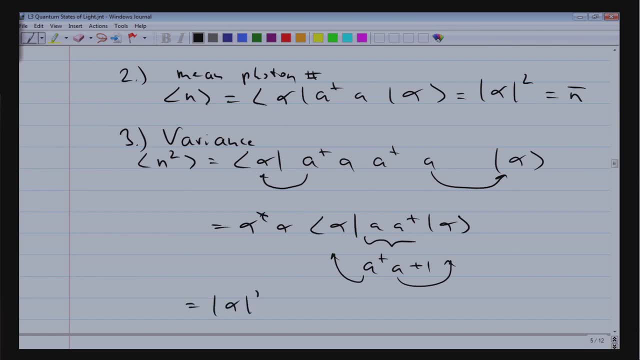 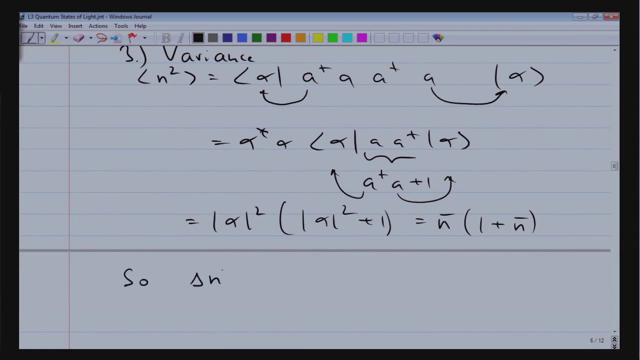 So therefore, in a very straightforward way, we find now that n square is alpha square times alpha square plus 1.. And using the result for the mean photon number, this is nothing else than n bar 1 plus n bar. So if we now put it together, we want to know the variance. 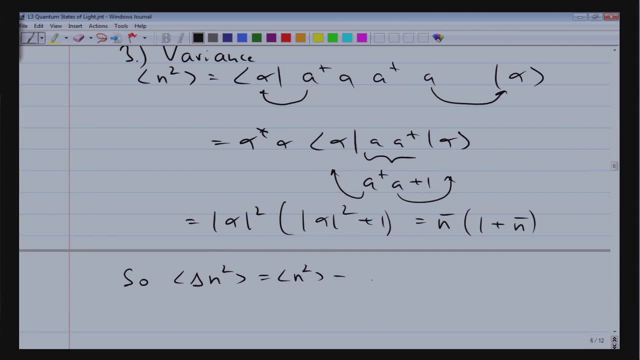 The variance is n square average, which we've just calculated, minus n average squared. And hooray, we find n bar And we verify again that the fluctuations are Poissonian. What else can we ask? We've asked about the statistics, the fluctuation, 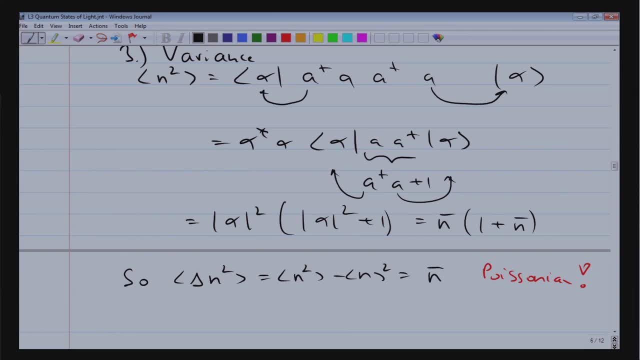 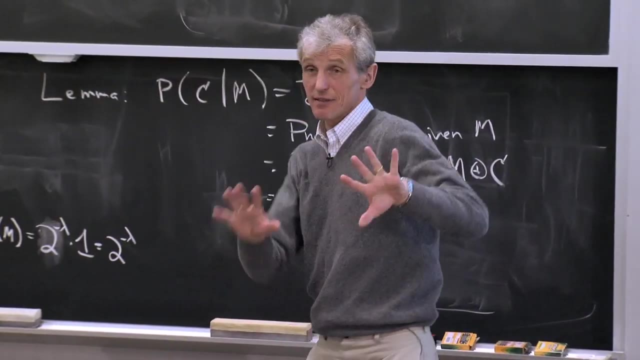 We've asked about the probability to find photons. Well, what else do we want to know about light Electric field? Oh, that's something I forgot to ask. I want to come back to that later, but just sort of to connect it. 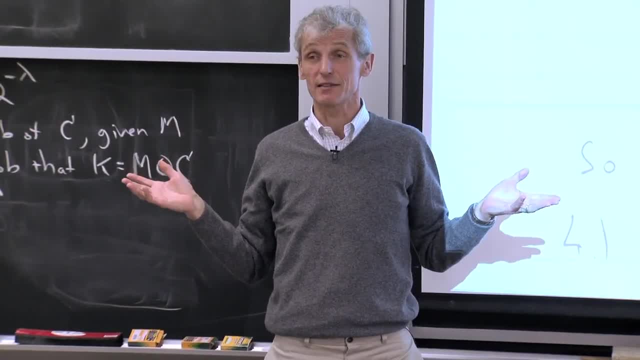 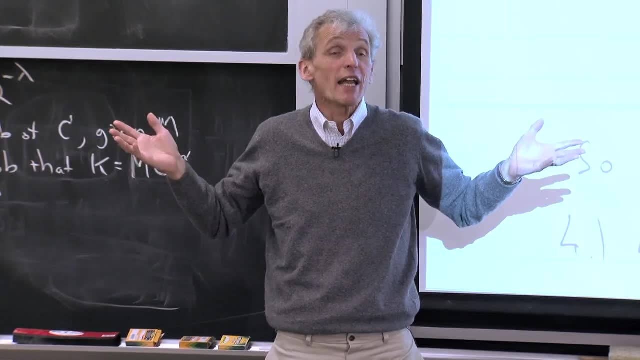 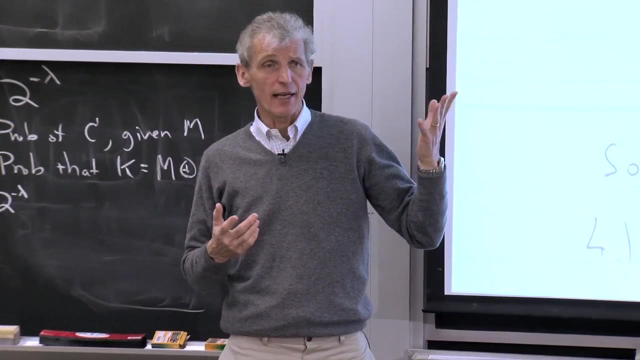 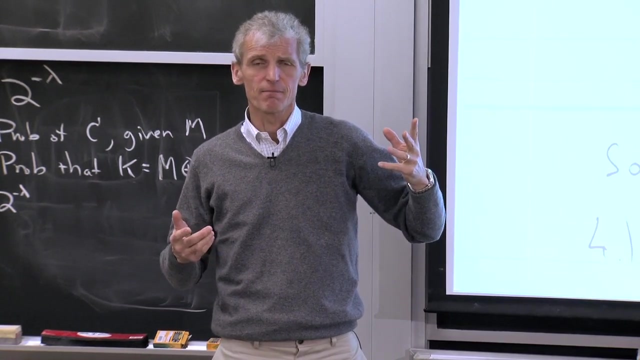 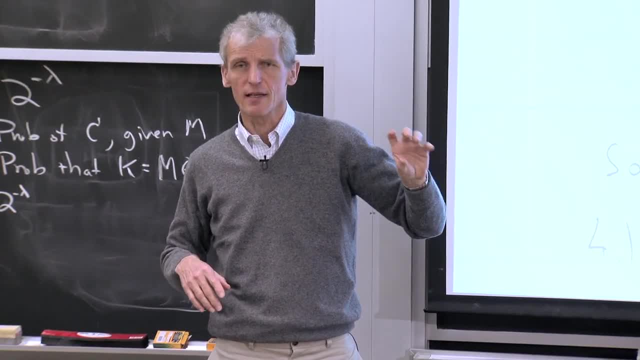 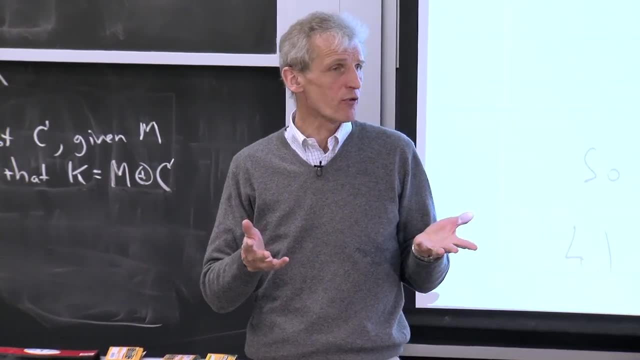 I see it- I see it loosely- that the photon has a phase. The phase will define whether it's positive or negative, But all different phases of the photon field, all different. What I mean now is coherent states which have different phases. 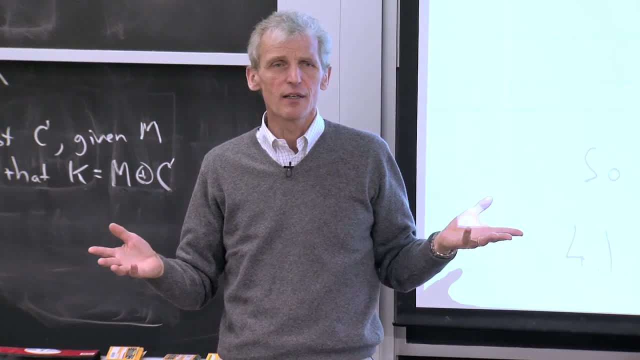 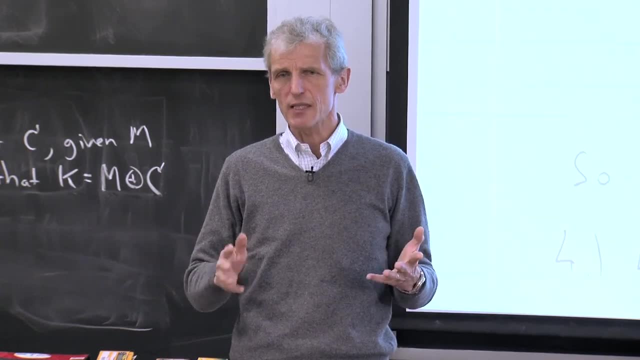 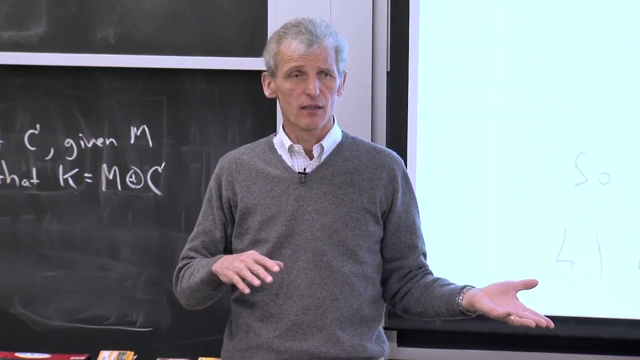 They are all degenerate. So in a thermal ensemble there is no thermal ensemble. The states are only populated due to their energy, They are populated by Boltzmann factors And therefore there is no distinction. There is no distinction what the phase of the state are. 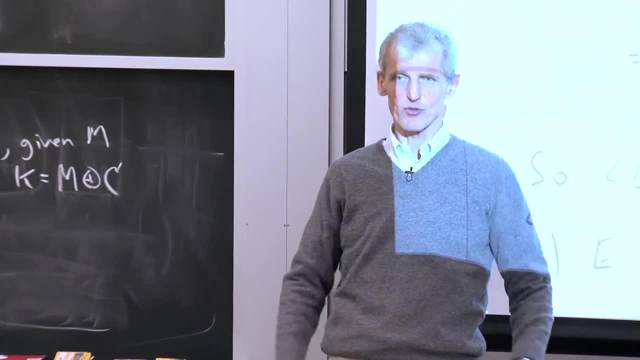 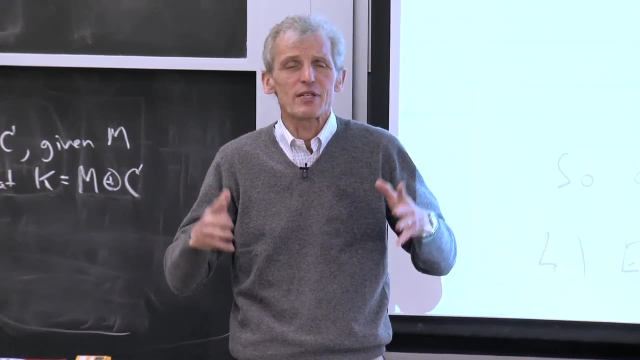 So therefore, we haven't defined yet what the phase of a photon is. Therefore I'm a little bit guarded with my language. But in other words, whatever the state with the phase is in the thermal ensemble, you have all phases simultaneously. 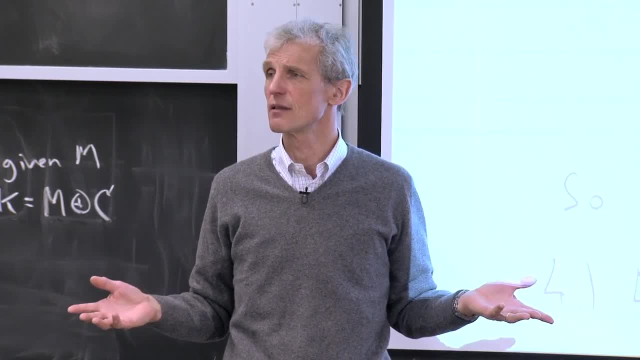 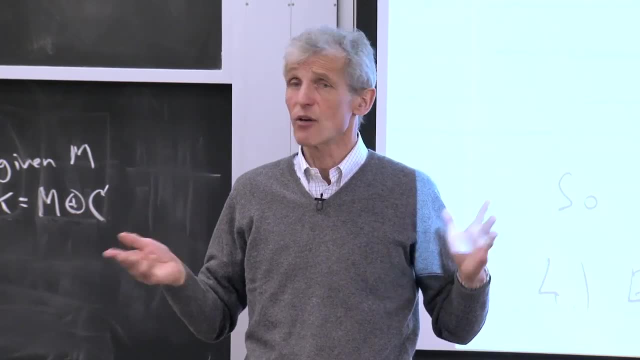 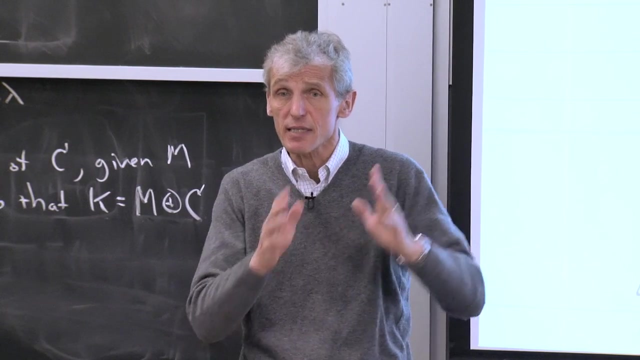 And therefore you never have an expectation value of E. But of course we had an average number of photons And that means we have an expectation value of E squared, because the expectation value of E squared is the expectation value of the energy. 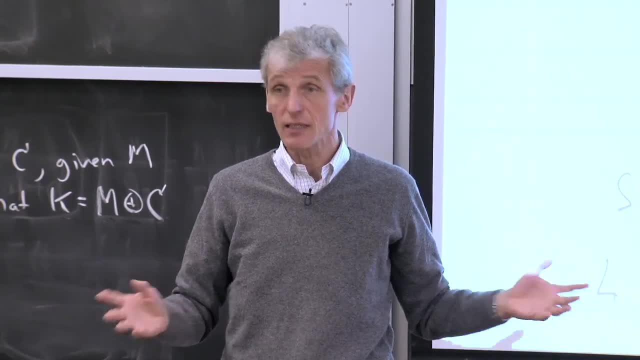 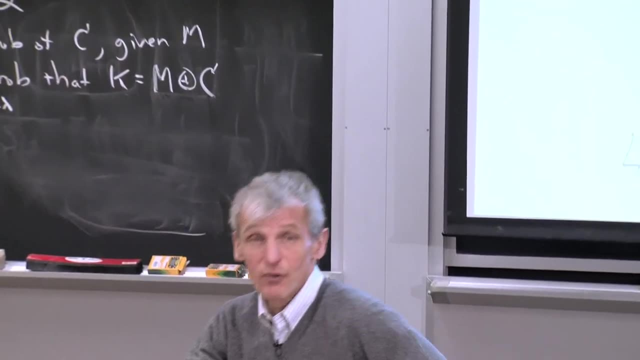 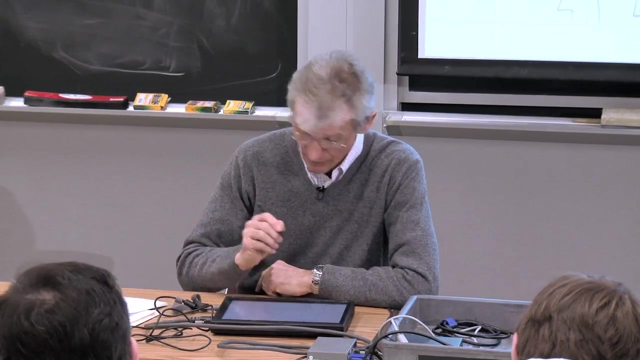 The state has energy but it doesn't have an expectation value for the electric field. OK, So maybe with that motivation we want to figure out now: does this coherent state which we have constructed, does that have now an expectation value for the electric field? 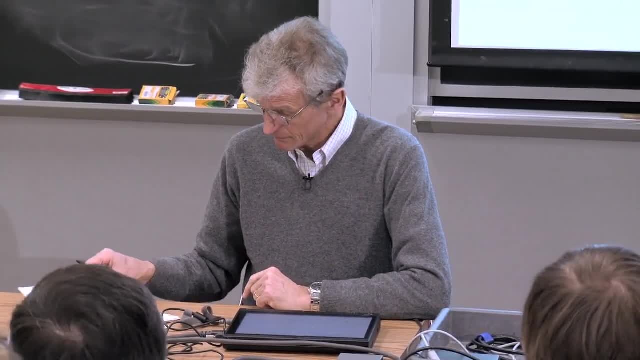 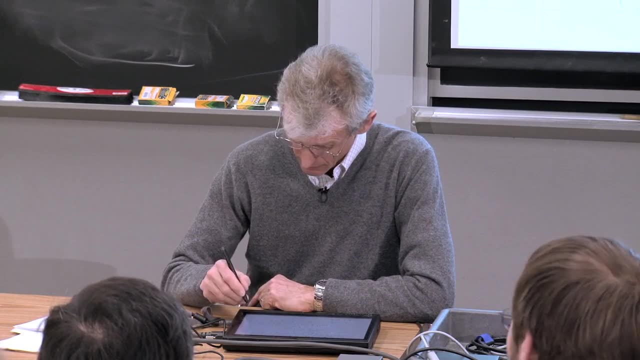 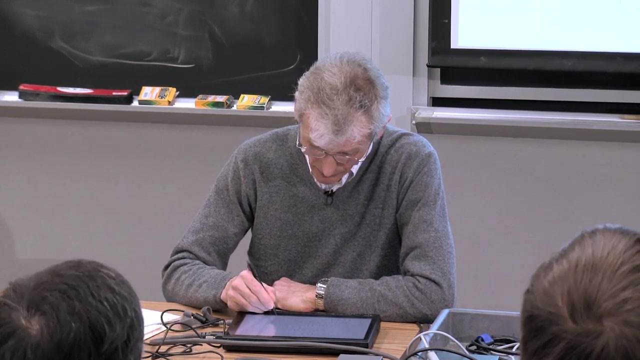 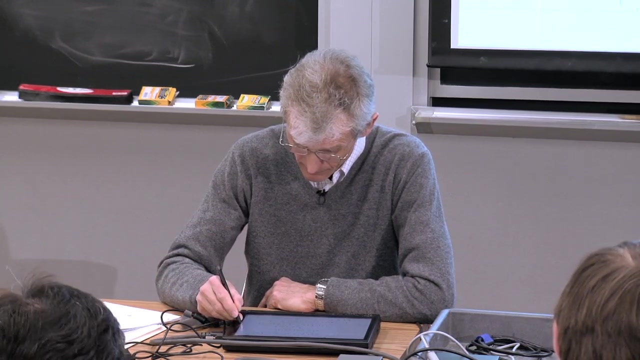 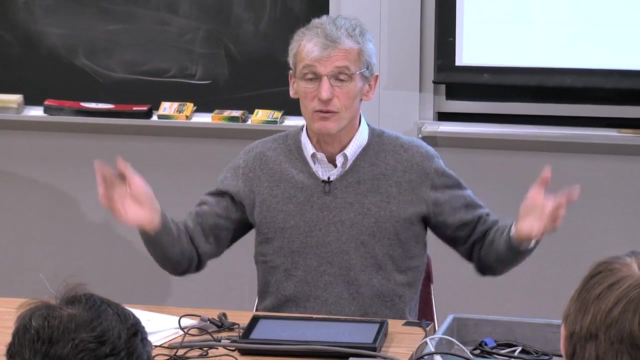 So there is one thing we of course know about this electric field: Whenever we have an electric field, it needs an amplitude and a phase, And what I just mentioned to you is that in a thermal ensemble, we were just looking at the partition function and such. 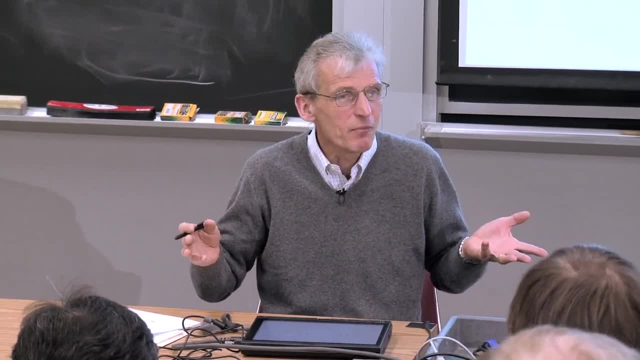 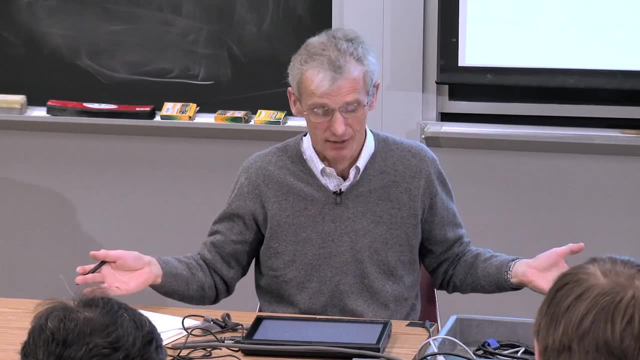 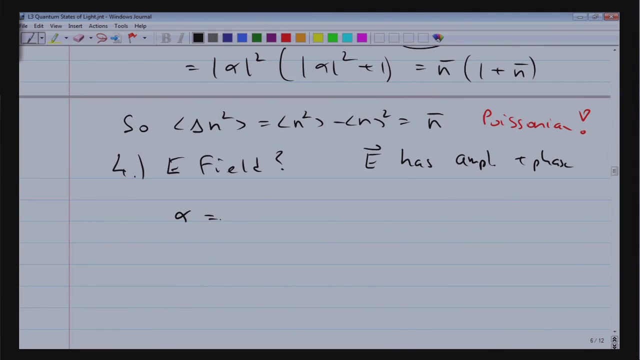 We didn't even mention a phase. There was not any complex number in any of the equations we wrote down about thermal light. No complex number, no phase means no electric field. But this is different now for the coherent state, because I mentioned that alpha in general can be complex. 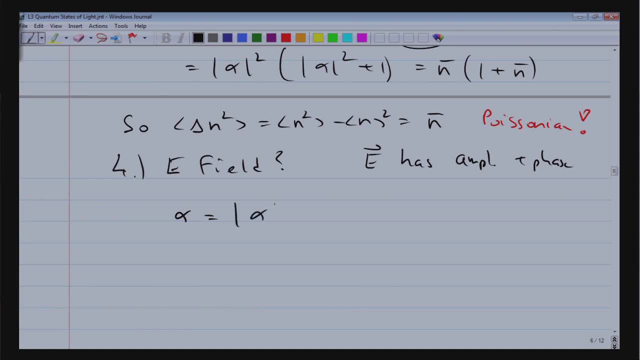 The annihilation operator can have complex eigenvalues. So, therefore, in the coherent state, because it is characterized by a complex number, we have now the possibility to include a phase, And what I want to show you in the next few minutes is that, yes, indeed, the coherent state. 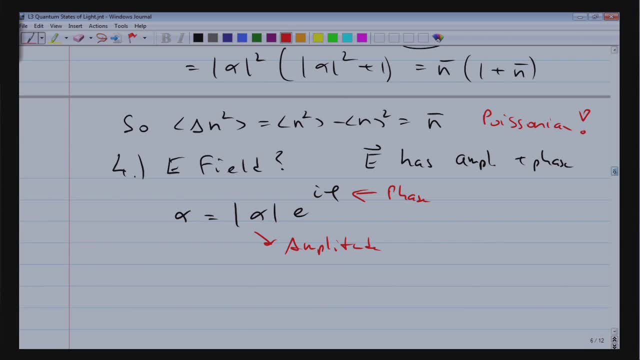 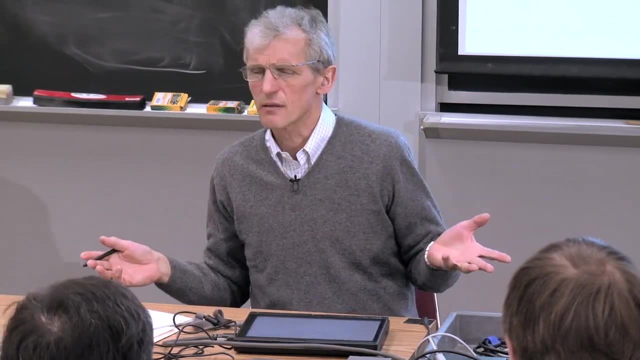 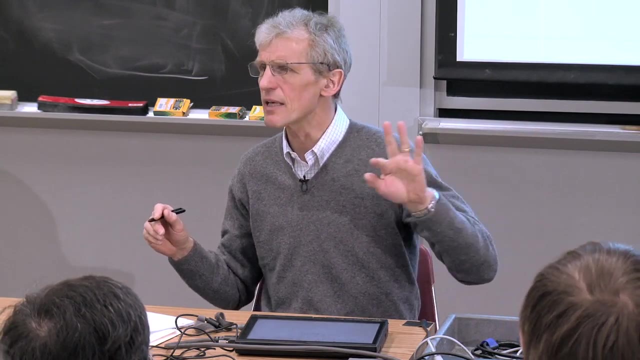 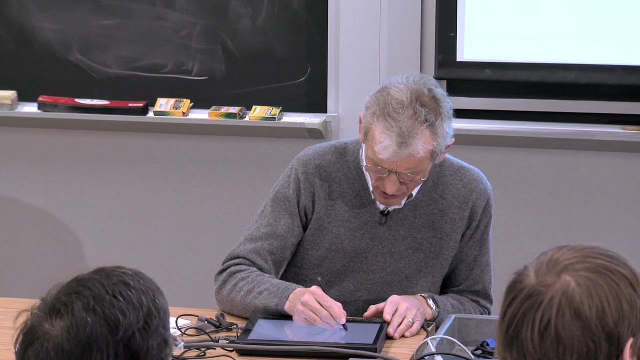 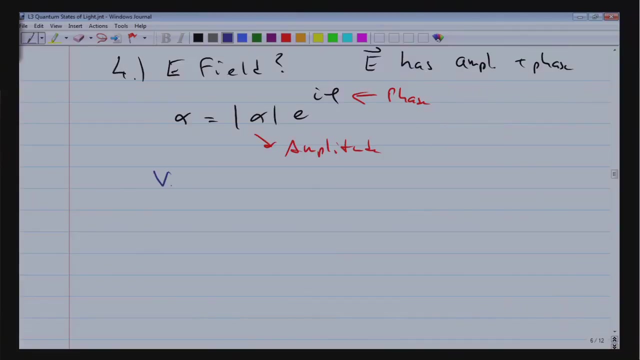 has an expectation value of the electric field. Instead of simply using the equation for the electric field operator- remember, electric field operator was a minus a dagger- I want to introduce something else which will turn out to be very, very useful And one of the application of this concept. 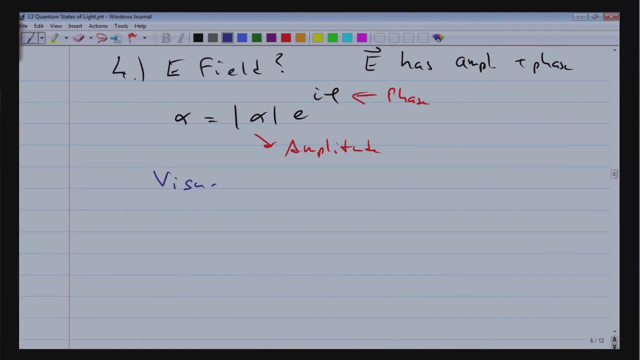 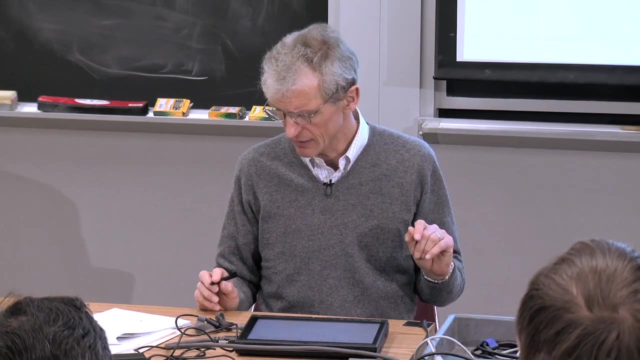 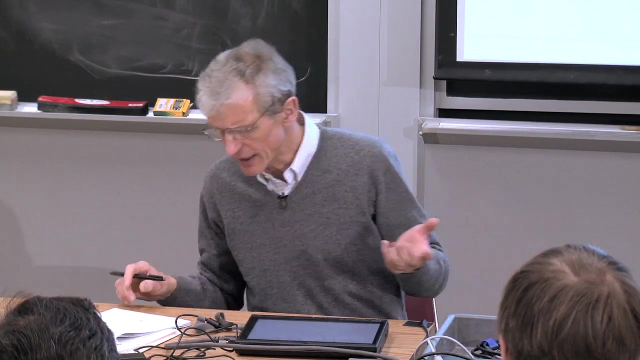 is to show you what the electric field is. This is sort of a visual representation, OK, A visual representation of the states of the electromagnetic field. So I want to sort of give you, in a two-dimensional diagram, a visual representation of thermal states, coherent states. 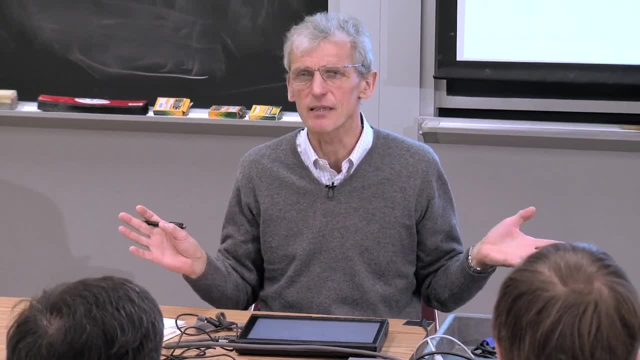 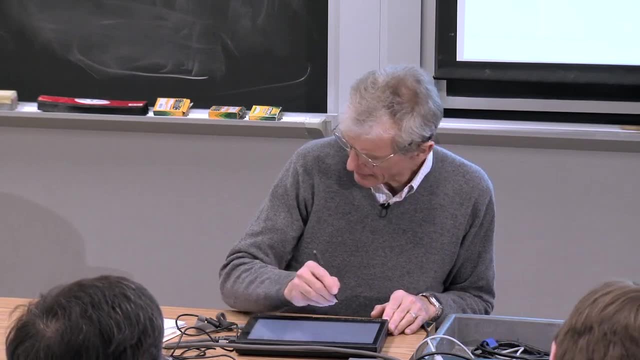 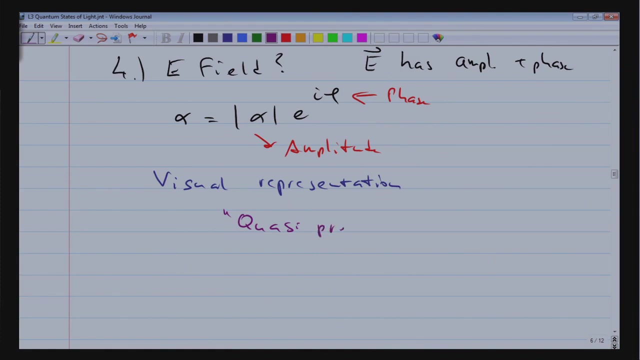 number states, And this visual representation will make it immediately obvious what the electric field is. OK, So this visual representation will represent what are called quasi-probabilities. So I have to define for you now those quasi-probabilities. So I denote the quasi-probabilities. 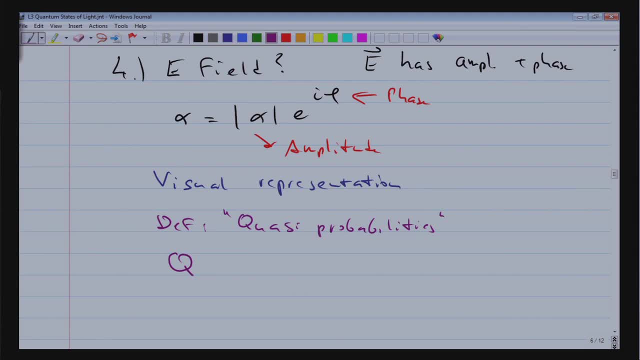 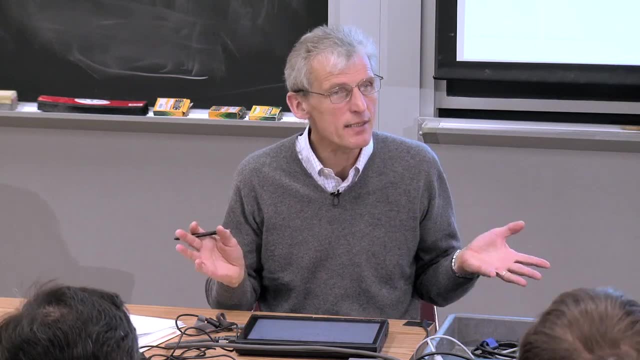 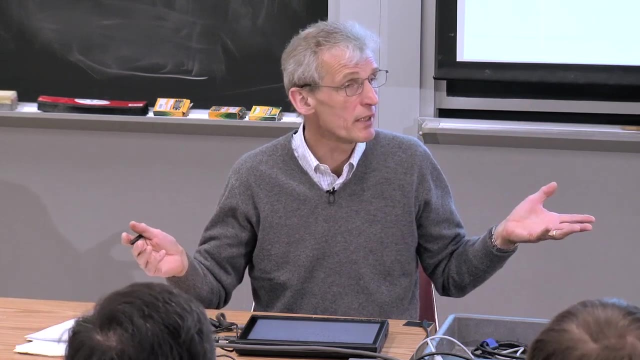 OK, OK, The quasi-probability by Q, And I want to know what is the quasi-probability Q for any statistical operator which describes a light. It could be the operator for thermal light. It could be a statistical operator. It also includes, of course, pure states. 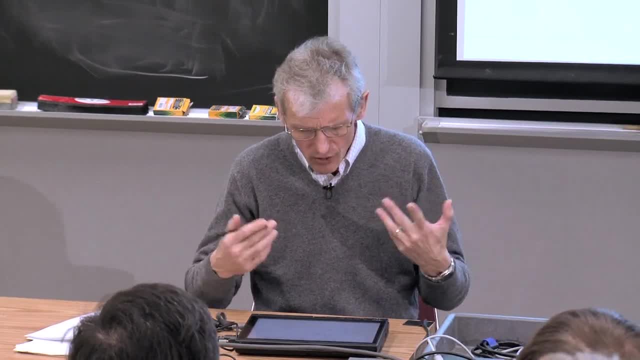 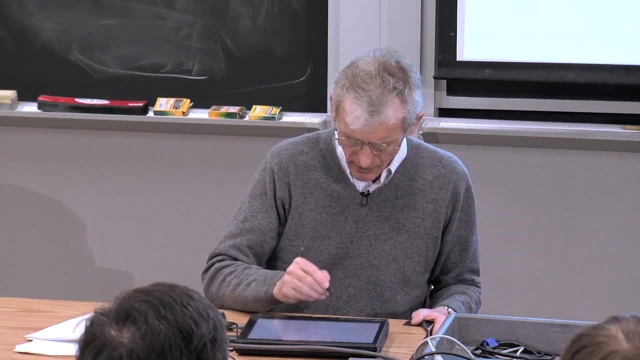 And the pure state could be a coherent state. So this is a way to define now quasi-probabilities for any statistical operator which is describing light. It's describing the light And the quasi-probabilities well, the probability for what? 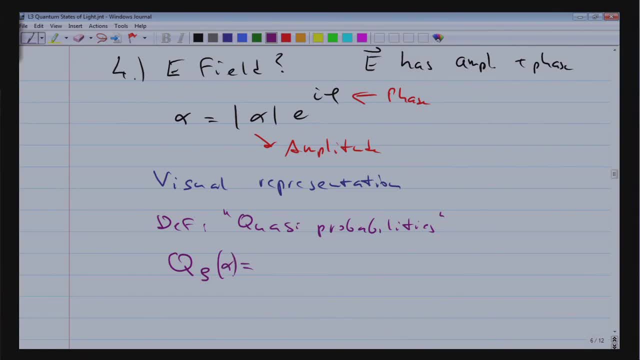 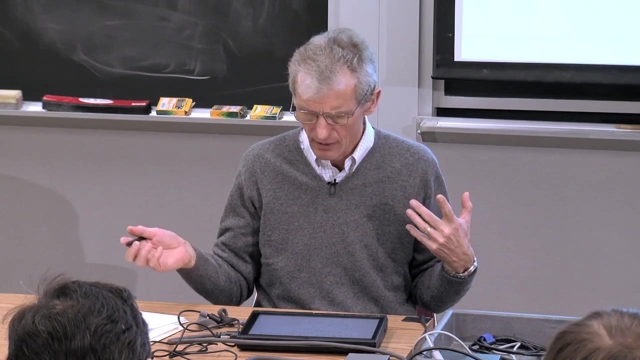 Well, the probabilities for alpha, And alpha is related to the coherent state. So in other words we say a statistical operator has a quasi-probability with a coherent state alpha- by simply calculating this diagonal matrix element. And that's the definition of the statistical operator. 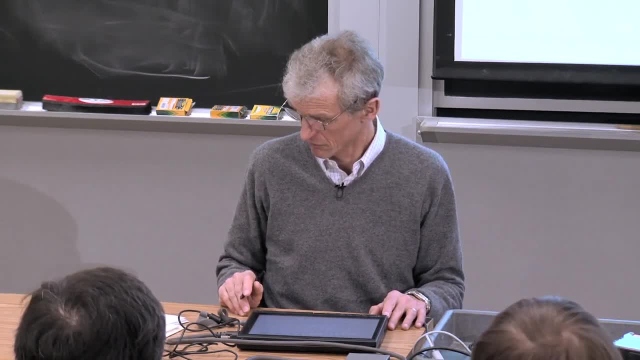 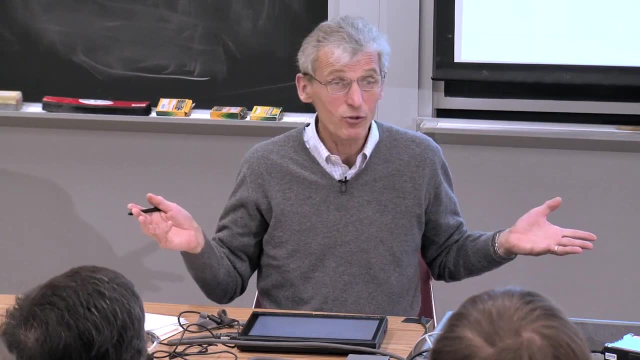 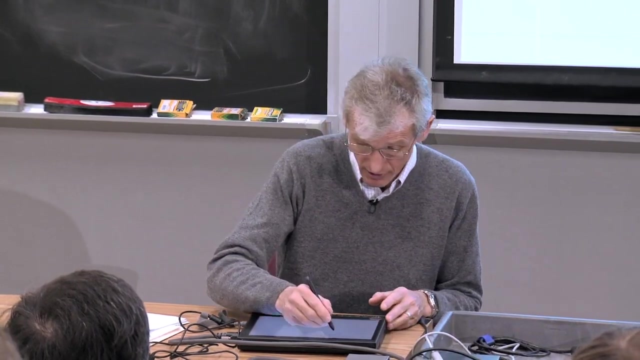 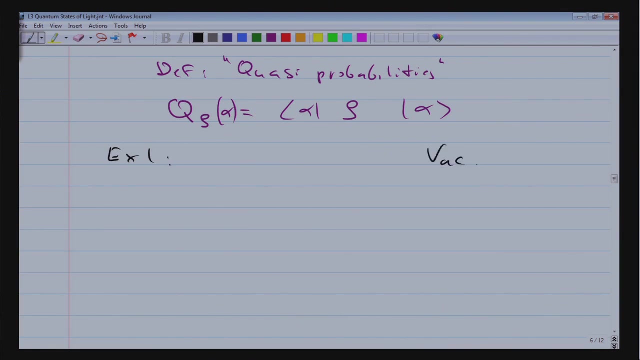 with alpha. Well, that's an abstract definition, but it's exact. What we should now do is I want to show you some examples And then you will actually see that it's actually a wonderful definition. So my first example is: let's look. 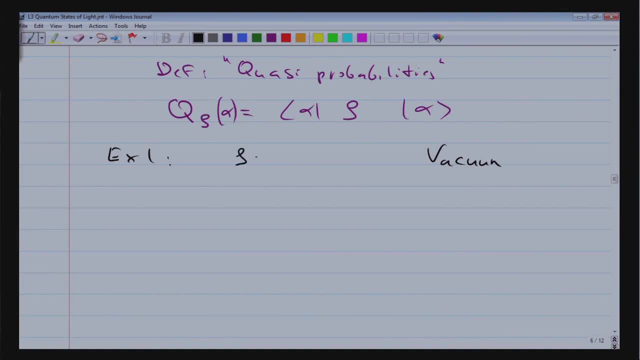 at the quasi-probability for the vacuum state. So if the statistical operator is simply the ground state of the harmonic oscillator, no photon, no, nothing, just empty vacuum. So the quasi-probability for well, the statistical operator is now a pure state. 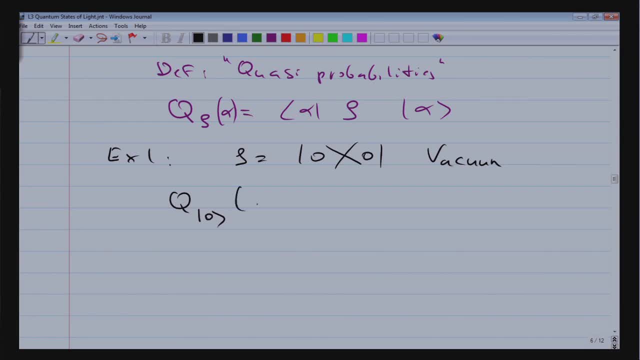 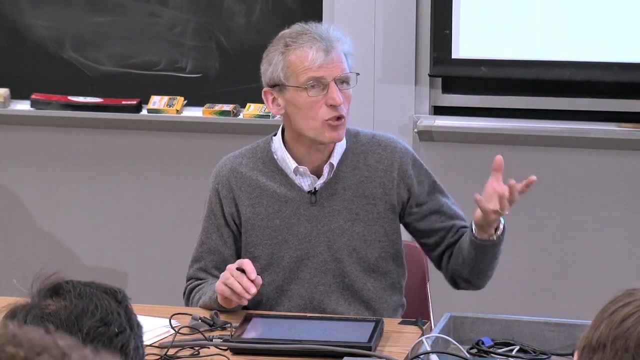 So I can say what is the quasi-probability of the vacuum state to be in state alpha? Well, Following the definition Above, It's nothing else than the matrix element, the overlap between the vacuum and the coherent state alpha I've given you above the representation. 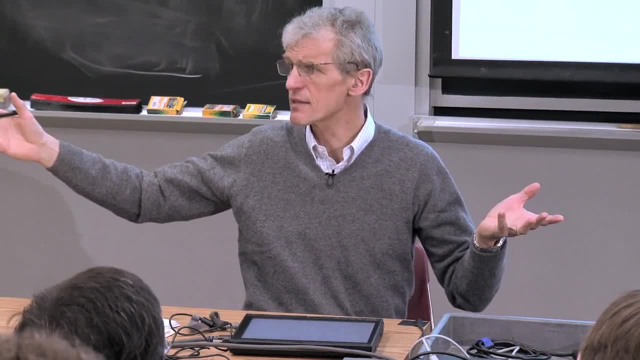 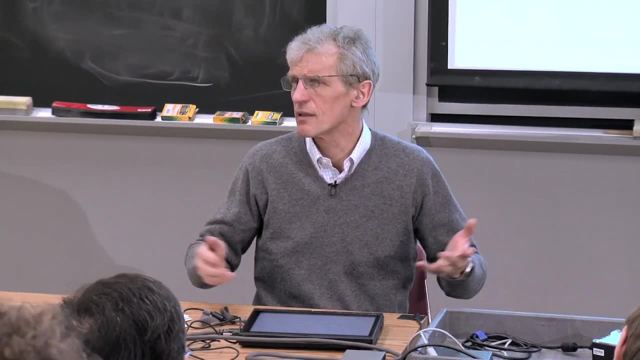 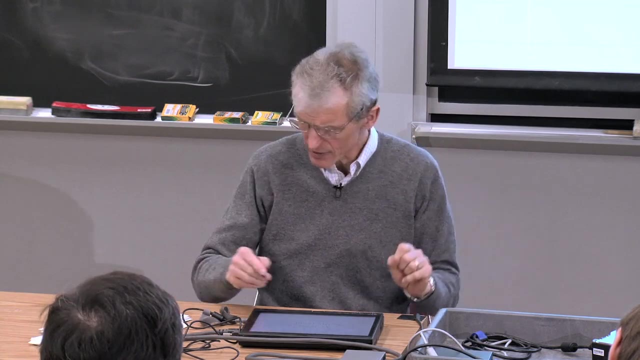 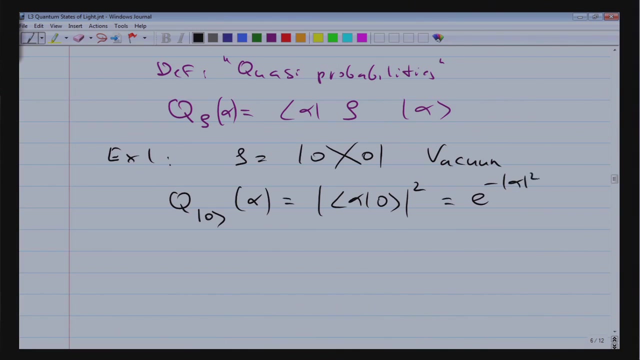 of the coherent state alpha in terms of number states, And all you have to do is look now upstairs. what is the amplitude that this representation includes a vacuum state. So it's just read off The amplitude C0 from the state above, And this was simply e to the minus alpha squared. 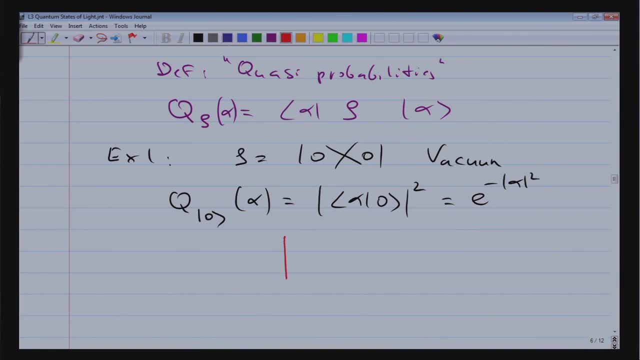 So, therefore, if I those quasi-probabilities can be plotted in a two-dimensional plane because it's a function of alpha, so if I use the real part of alpha, The imaginary part of alpha, Now I can plot the quasi-probability Q. 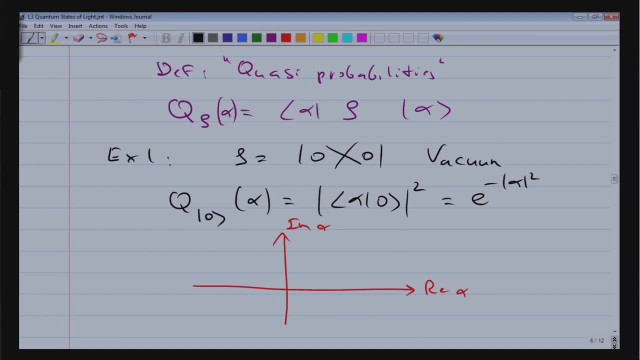 And since it's hard for me to do a 3D plot on the tablet, I just sort of shade the region. Sort of black means the amplitude is large And now sort of here it means the amplitude falls off. So what I'm plotting here is a Gaussian. 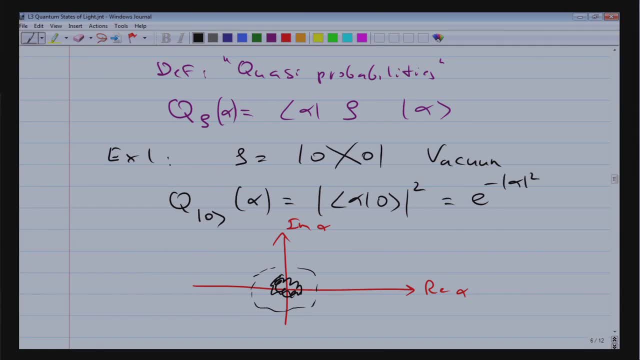 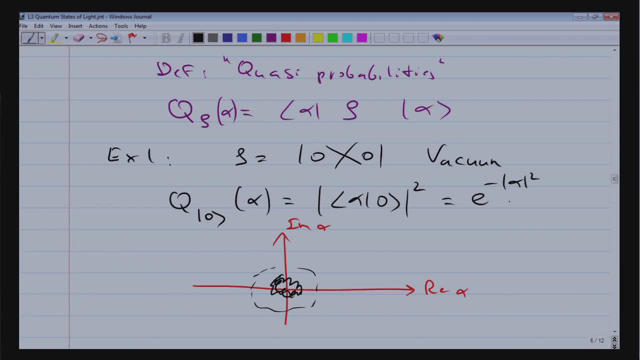 I think in the standard deviation of the Gaussian you have a factor of 2.. Anyway, it's on the order of it's a Gaussian with only order of unity. I think it's 1 over square root, 2, or whatever the definition of the standard deviation is. 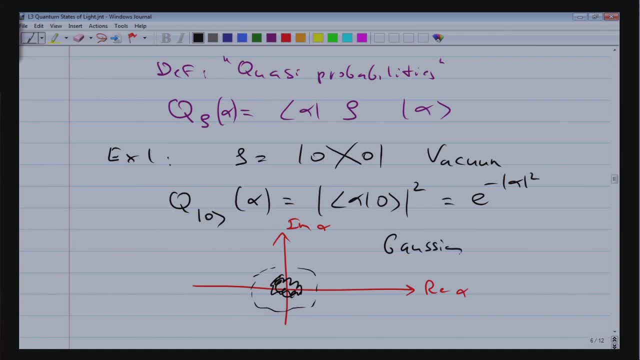 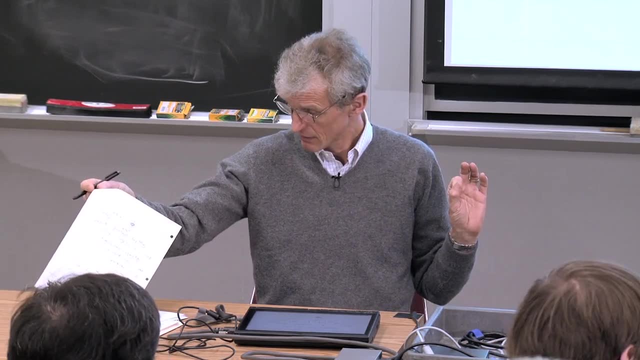 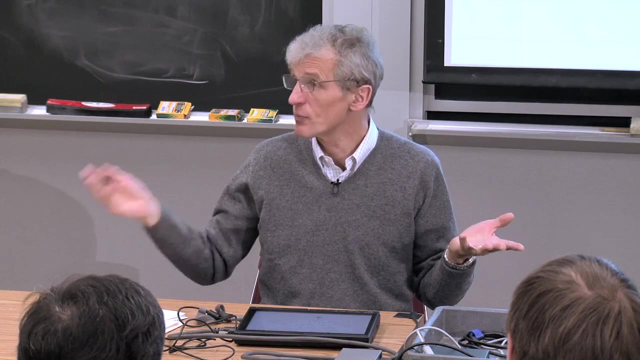 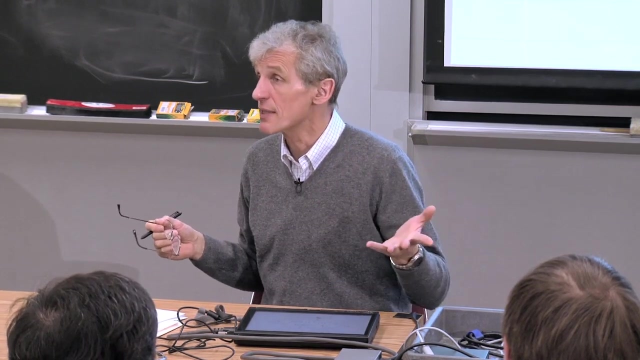 So here we have a Gaussian, Any questions? So for pure state, we are simply asking what is the amplitude of the pure state to overlap, to be in a coherent state, And what we are plotting is nothing else than the probability that this state is a coherent state. 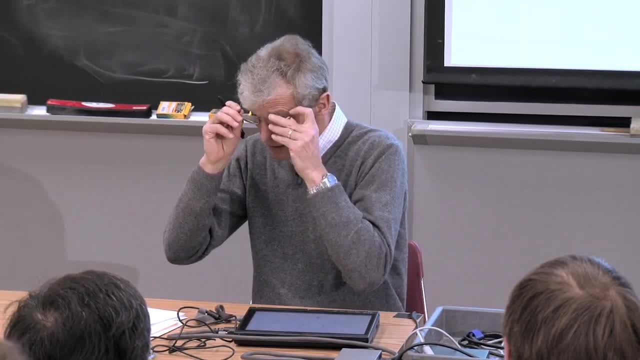 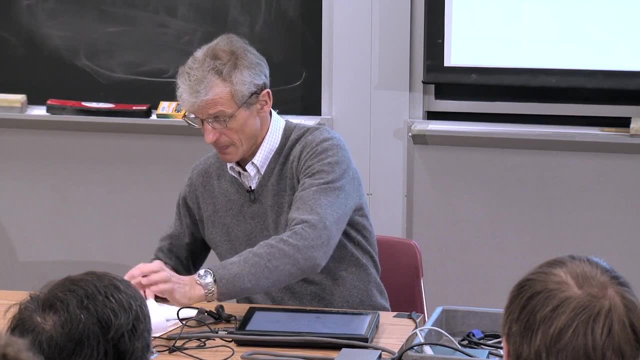 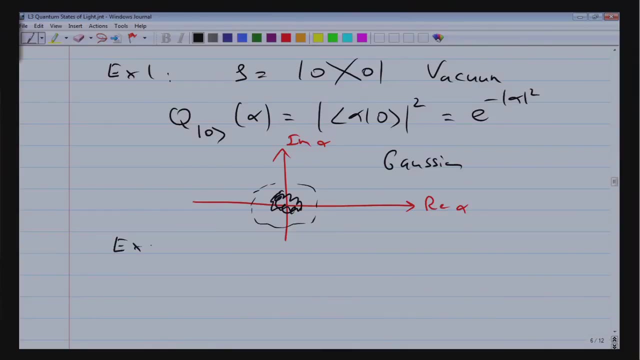 with value alpha. Good question. The next example- and we've already prepared for that- is the thermal state. Example number two is the thermal state. So we want to know what is the quasi-probability for the thermal state? It's a function of alpha. 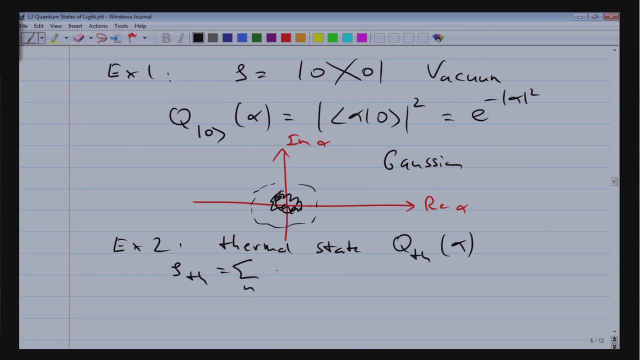 The statistical operator for the thermal states, we had derived it above, was the probability to find n photons, And in the number representation the statistical operator is diagonal, And then the quasi-probabilities are nothing else following the definition above. Then those probabilities times the matrix element. 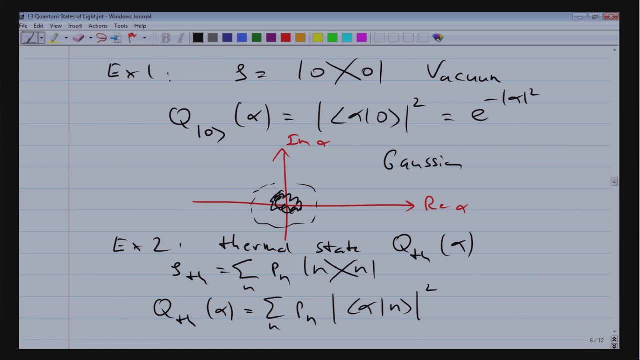 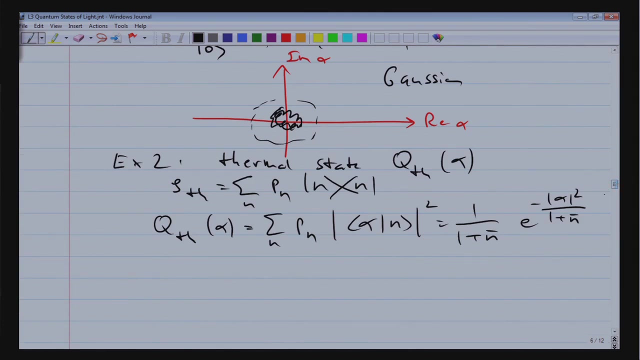 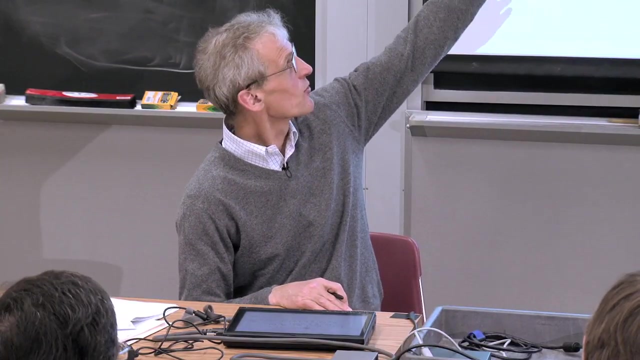 the overlap between alpha and n, And if you look up what we had derived for the probability Pn, you find a very simple result. What we obtain is again a Gaussian. It is also centered at the origin. So therefore, since I didn't label my axis, 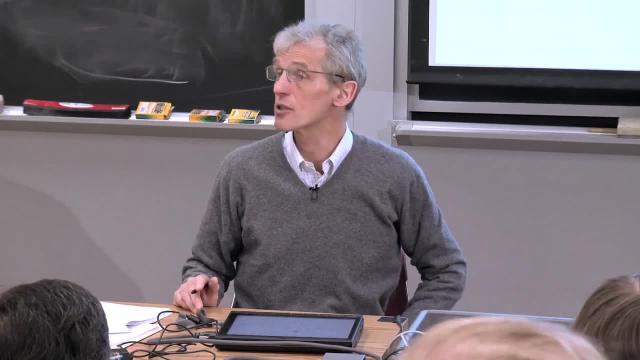 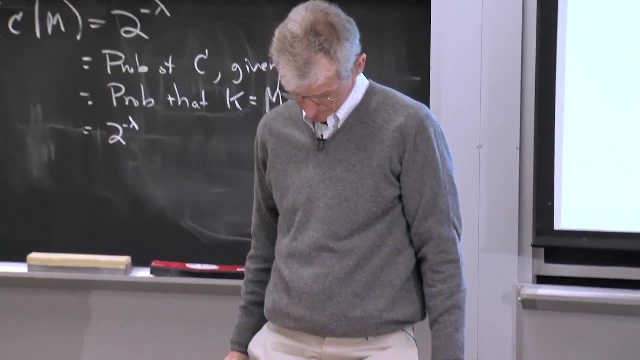 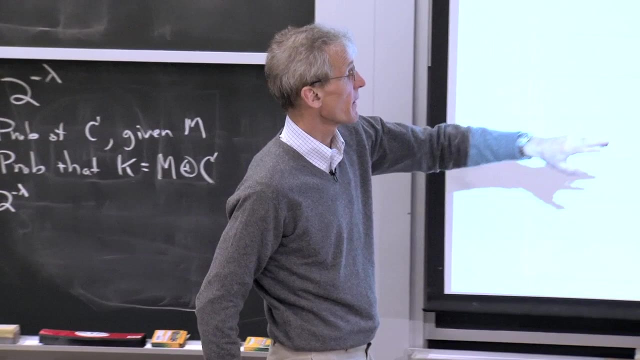 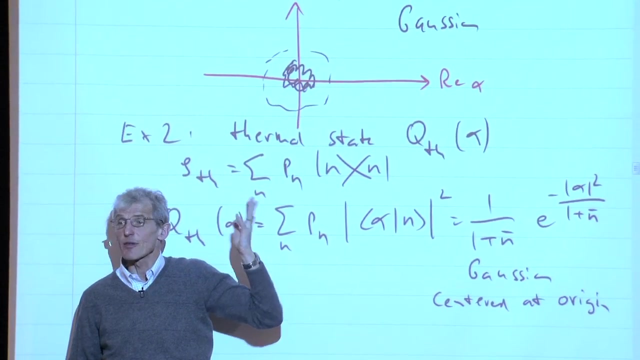 it looks exactly as the vacuum state. It's just that the Gaussian is much, much broader, And I will come to that. but an intuitive reading of this Gaussian is: well, this Gaussian has a peak at the origin, At the origin. this is where alpha equals 0.. 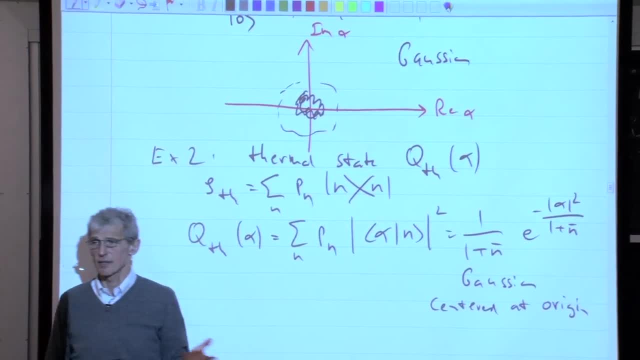 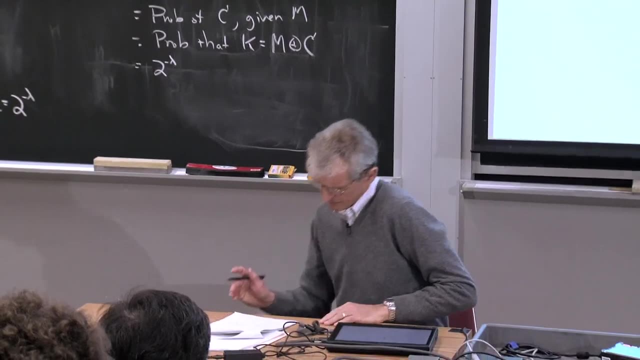 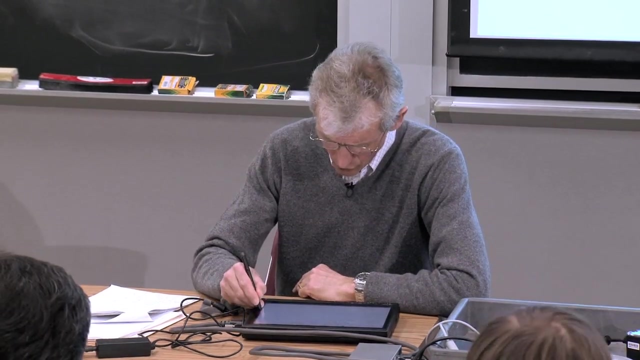 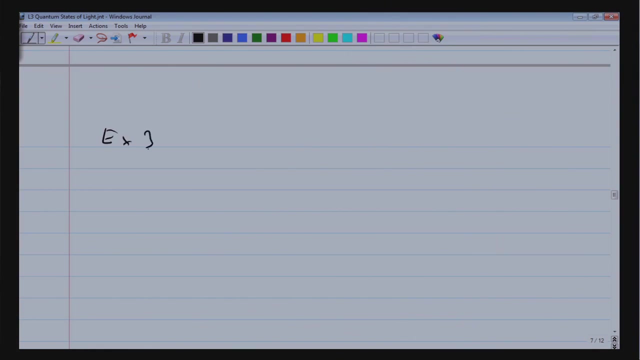 And this is directly related to the question I asked you before- that the photon number probability is peaked at n equals 0. But I hope this will become clear. It will become even clearer when we move on to the third example, which is now. 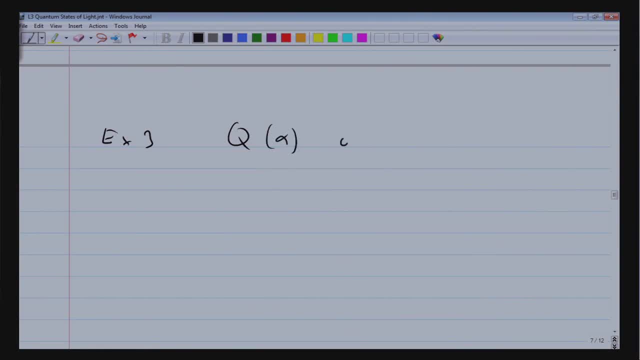 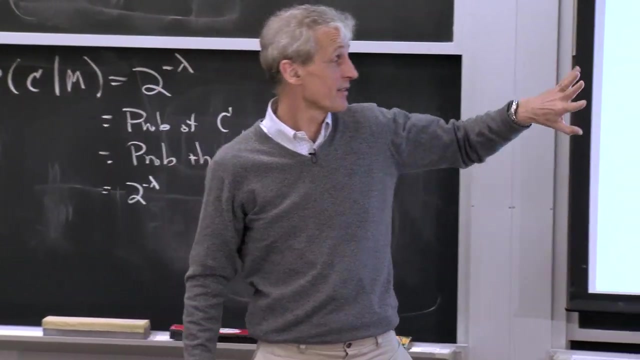 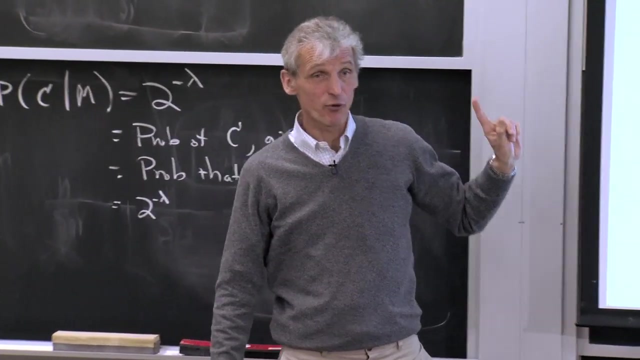 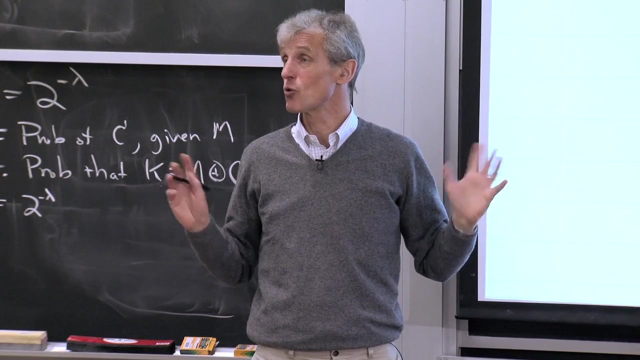 Q of alpha of a coherent state. OK, Maybe, just before I even discuss the quasi-probability of a coherent state, I have to address one thing up front: What would you expect the quasi-probability of a coherent state to be? 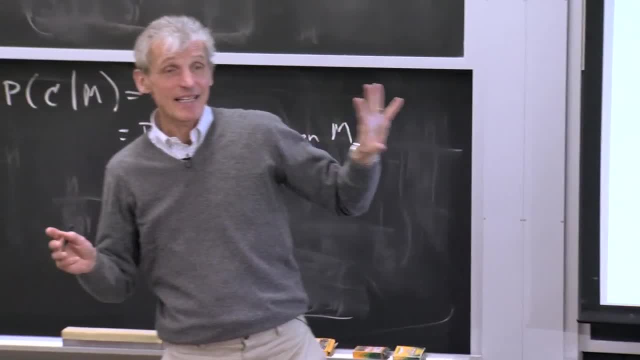 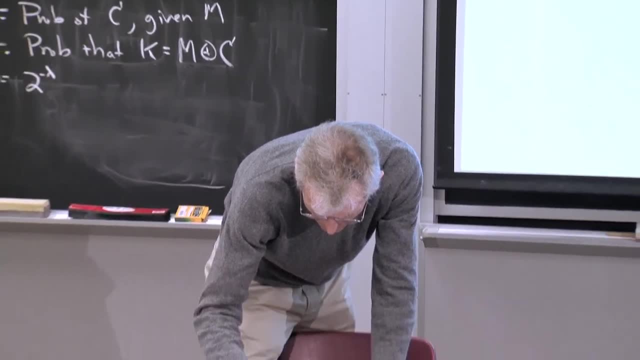 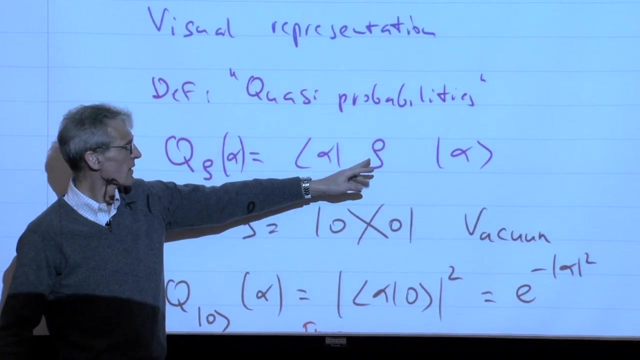 Pretty good. but I said before the quasi-probability. let me just show you how it was defined. Here was my definition of the quasi-probability And you can say: the quasi-probability is the diagonal matrix element of the statistical operator. 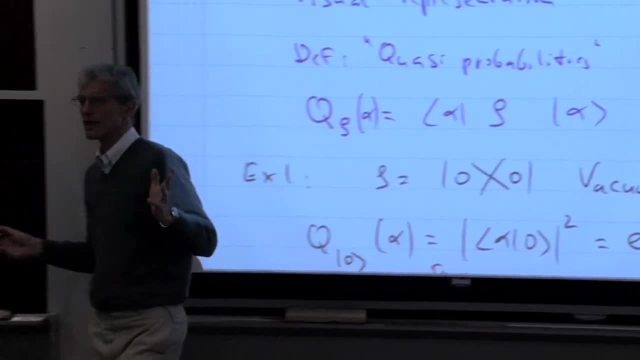 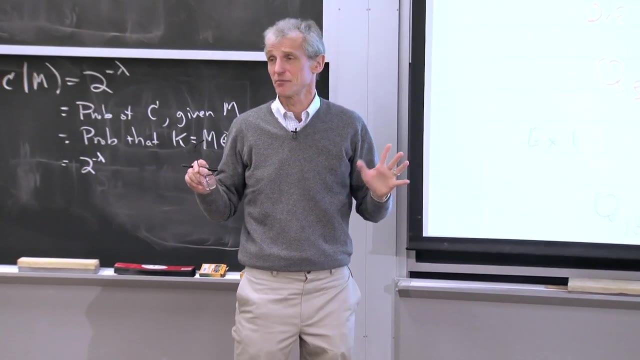 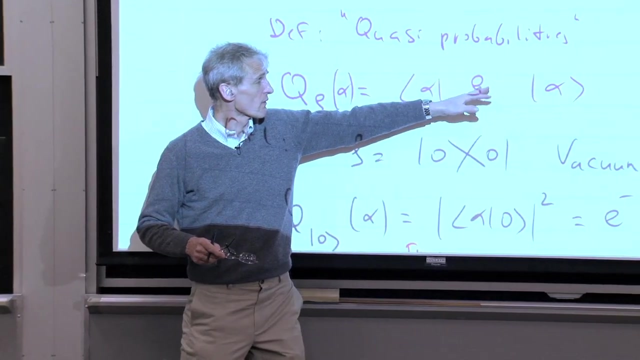 with a coherent state. But if our statistical operator is a coherent state, what would you expect this probability to be, just naively 1. 1. 1 or a delta function? I mean, it's sort of we ask if we. 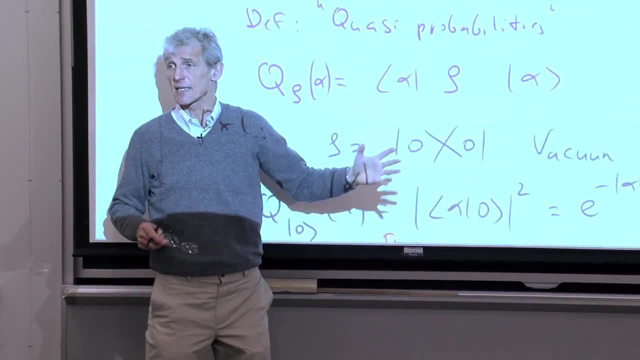 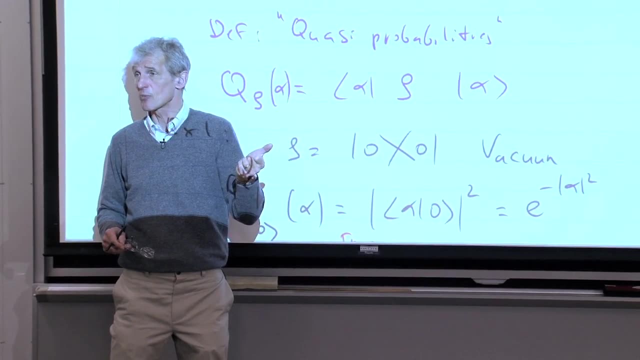 expand this statistical operator in coherent states, what do we get? But if this operator is a coherent state, let's say it's a coherent state, beta you would expect. well then we only get something non-vanishing if alpha equals beta. 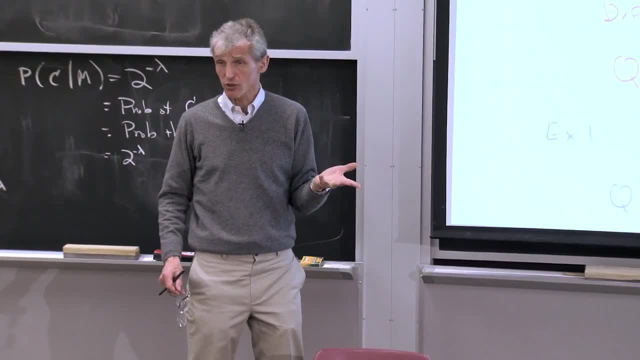 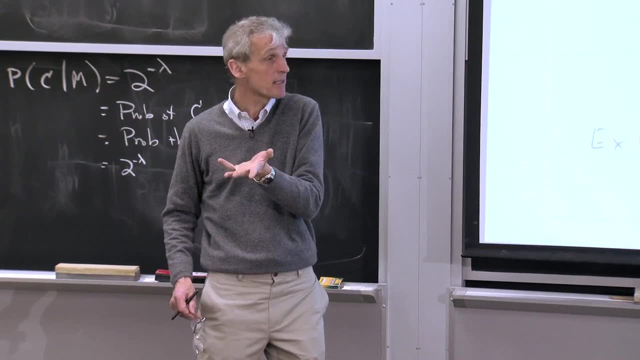 So you would naively expect that what you get is a delta function. The coherent state beta has a quasi-probability Q of alpha, Which is peaked at beta, but it's peaked as a delta function. Now I'm calculating it for you right now. 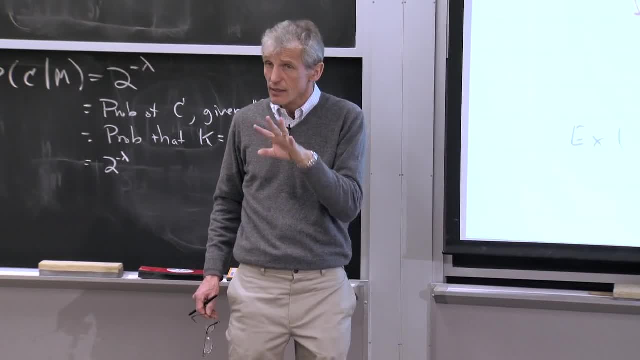 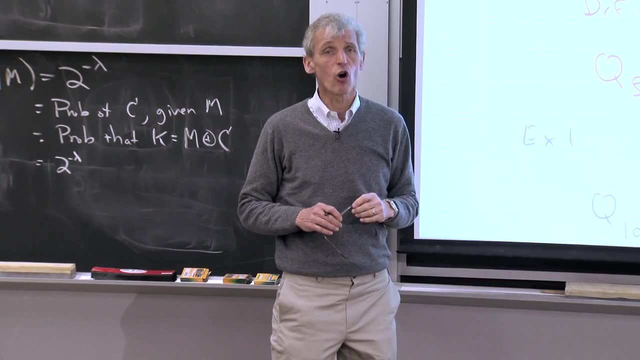 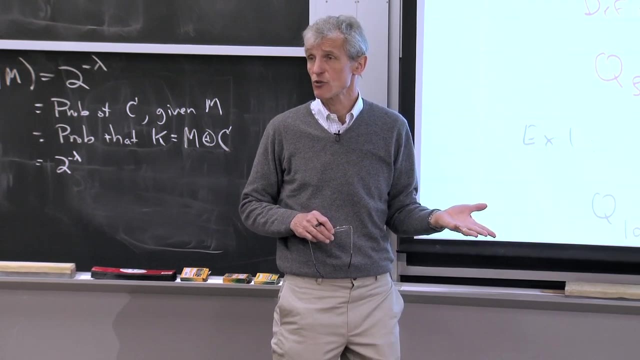 And the result is: this is not the case. The reason is- and I will show that to you- is that the coherent states are not your ordinary basis function. The coherent state forms a basis which is over-complete, So we have sort of more coherent states. 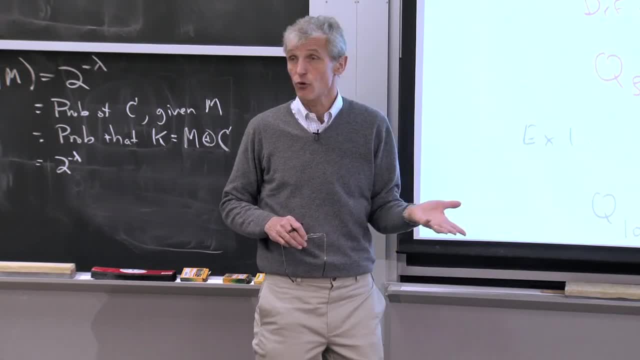 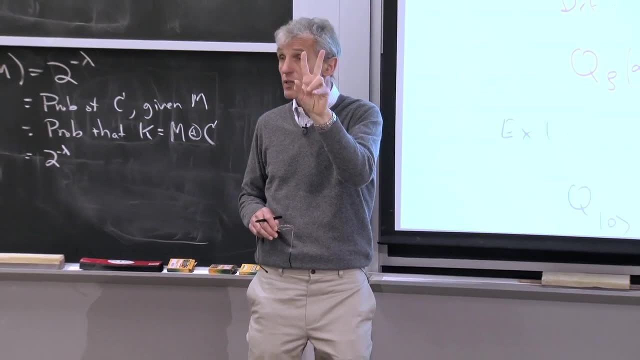 than necessary. There is some redundancy and therefore the coherent state alpha and the coherent state beta, if alpha and beta is only, if there's only a small difference between alpha and beta, they have overlap, Coherent states which differ by only a little bit. 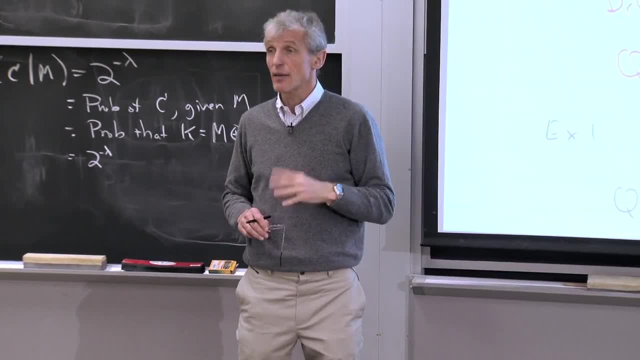 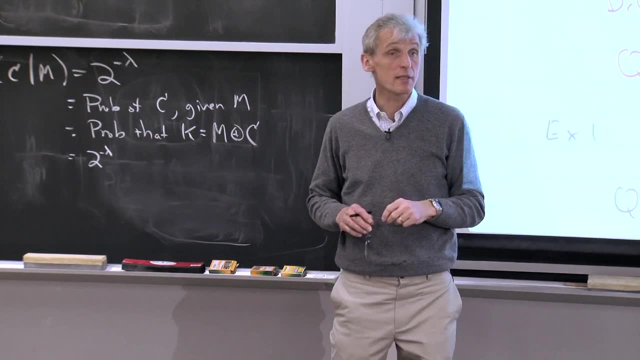 in their eigenvalue. they're not orthogonal, So this is a complication. It's one of the complications we have to deal with when we want to describe coherent states and when we want to describe non-completions. We want to describe laser light. 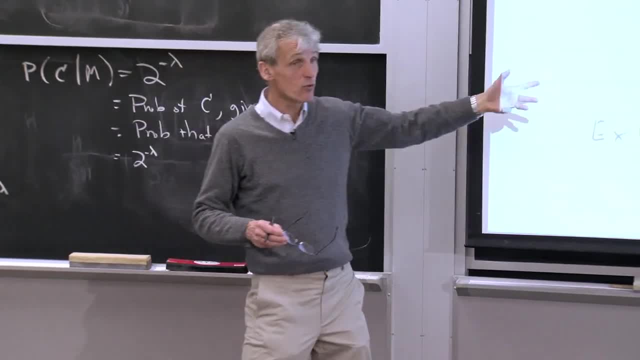 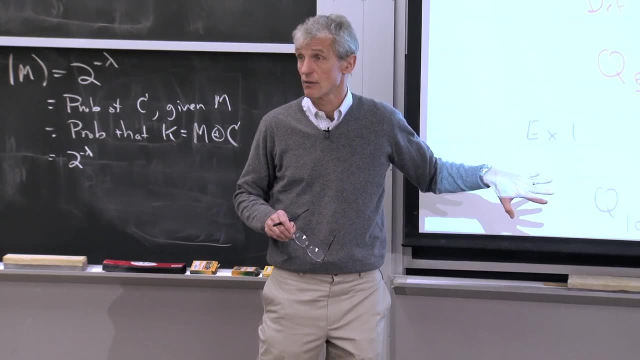 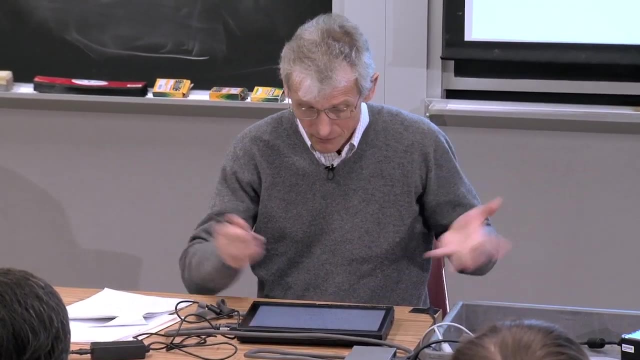 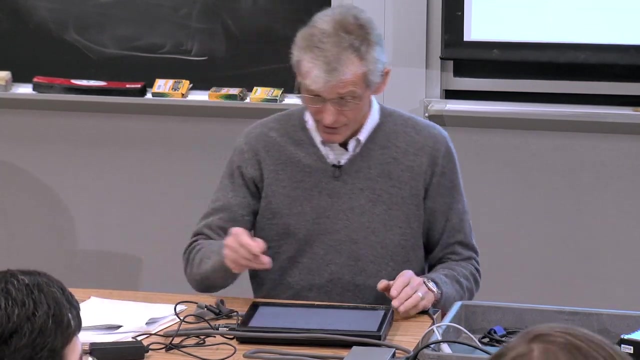 But this is one of the properties. So, therefore, what I'm now discussing with you is: what are the quasi-probabilities of a coherent state? It will not be a delta function, But we should simply follow the definition and everything will fall into place. 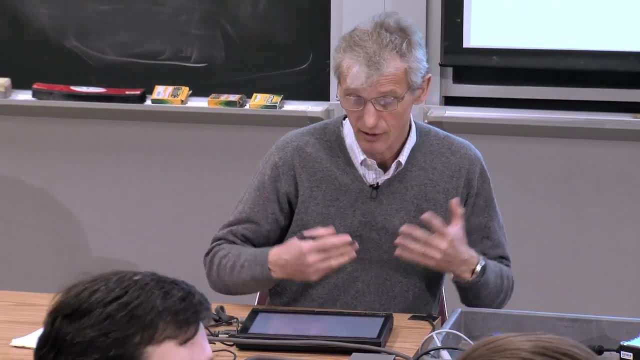 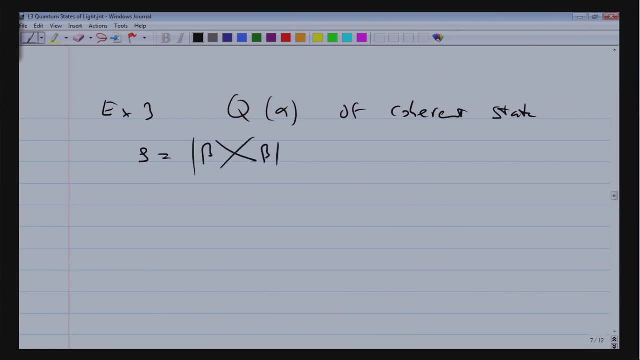 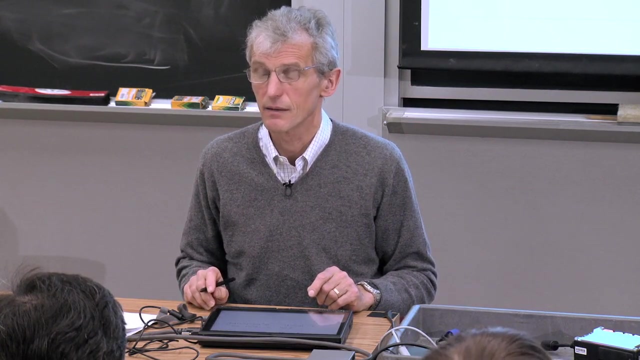 So our statistical operator For a pure coherent state is, of course- this is a statistical operator of a pure state beta And the quasi-probability for the coherent state beta to be in alpha is this matrix element squared And you can calculate it, for instance: 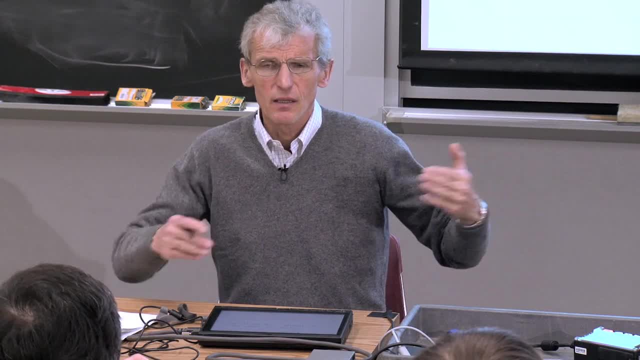 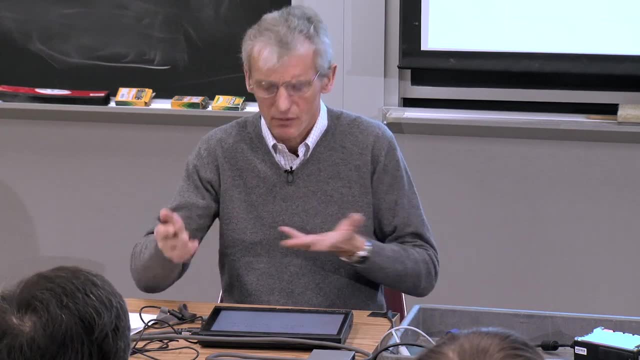 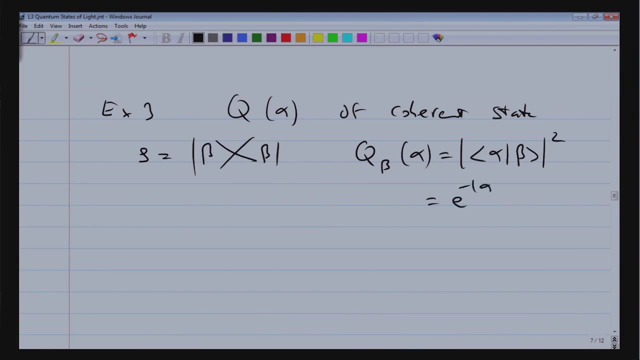 by just putting in now for alpha and beta, the expansion of alpha and beta in number states. So you just have to solve the integral and calculate it And what you find is not a delta function but in decaying exponential. So you can say: as long as alpha and beta you're going to be. 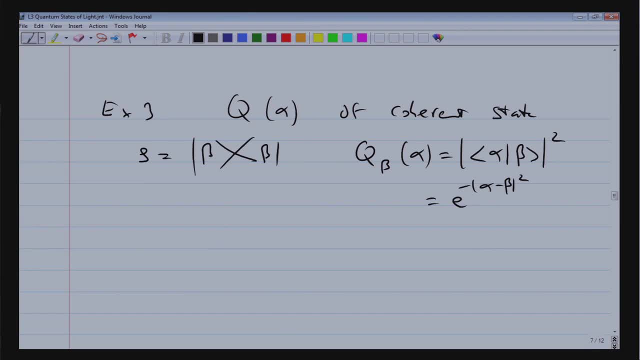 do not differ by more than 1, there is substantial overlap. So, in other words, what we get for this quasi-probability is something which is centered at beta, but it is again a Gaussian. So the important message here is coherent states. 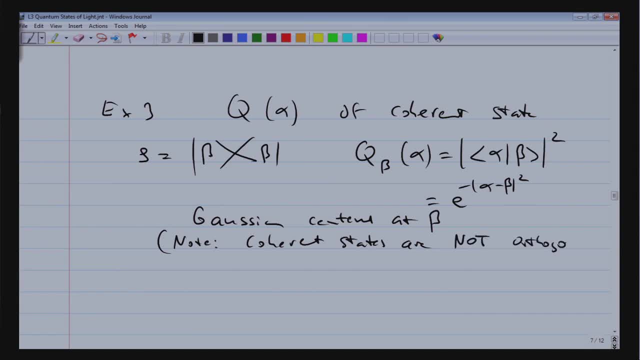 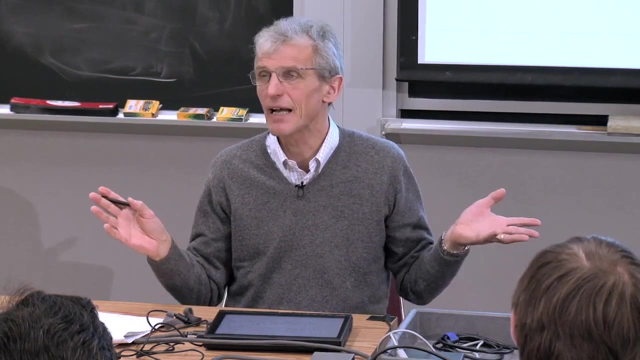 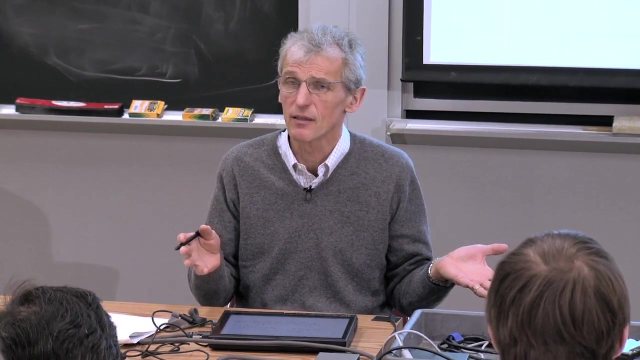 They are not orthogonal to each other. They form an over-complete basis. Maybe, as a side remark, it may come as a surprise to you because you have been trained too much in basis states of Hermitian operators, of energy eigenstates, And those energy eigenstates form. 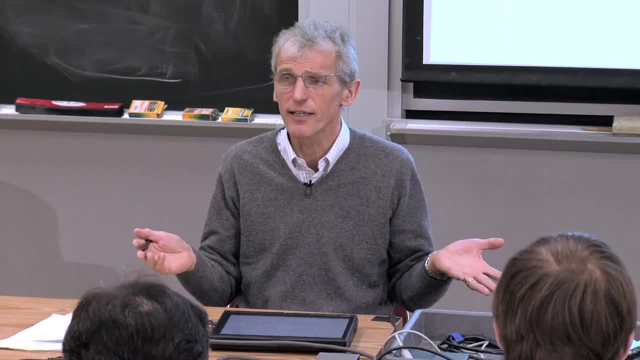 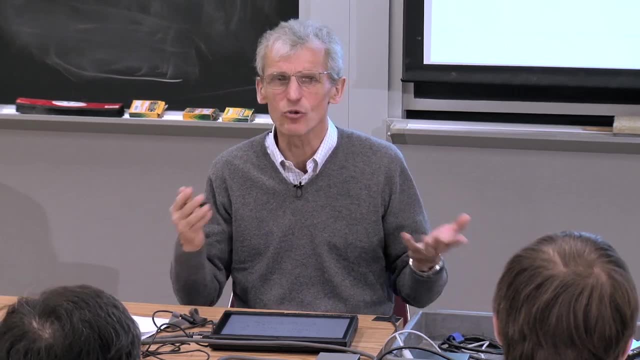 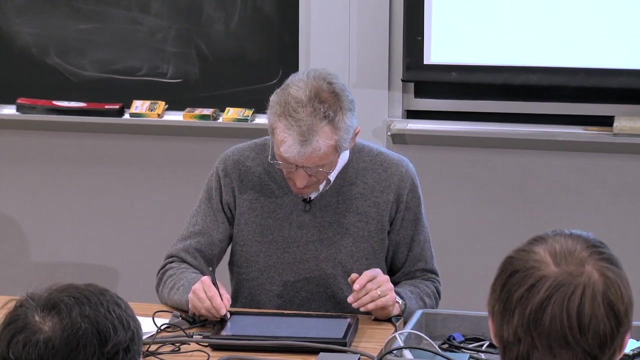 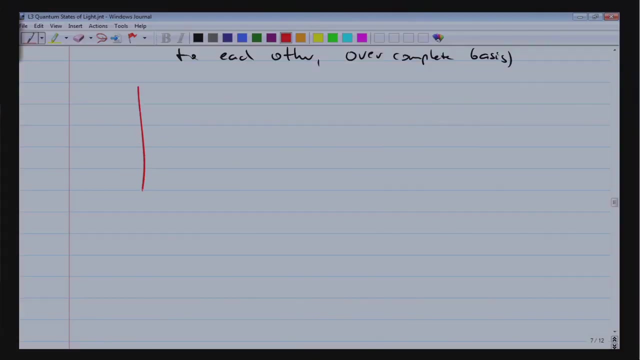 a complete basis. The coherent states are eigenfunctions of a very strange operator, a non-Hermitian annihilation operator. So therefore, the few things you took for granted do not apply here. OK, so we have our nice diagram with a nice diagram. 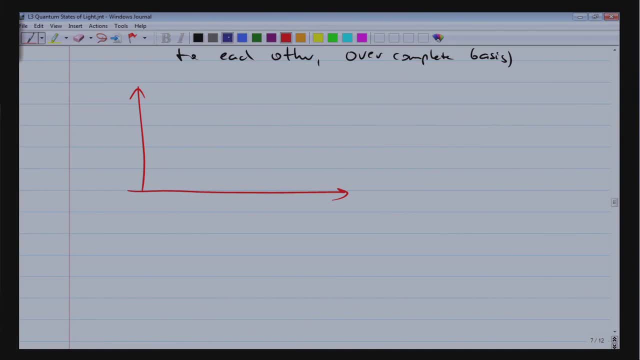 for quasi-probabilities. So now, if we have a nice diagram, we have a nice diagram for quasi-probabilities. So now, if we have a nice diagram, we have a nice diagram for quasi-probabilities. So now, if we have a nice diagram, 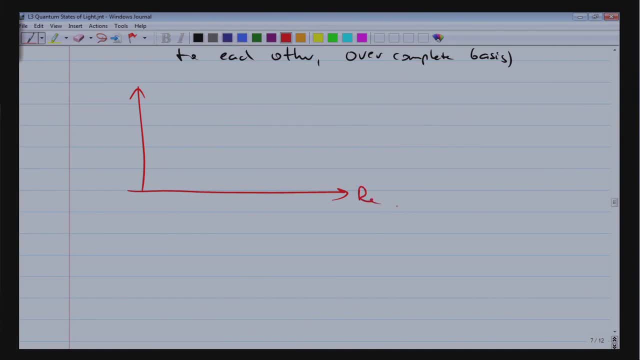 we have a nice diagram for quasi-probabilities. That was the real part of alpha, That was the imaginary part of alpha. So if we take that as a complex plane, and I'm drawing now as a phaser the complex number beta, which 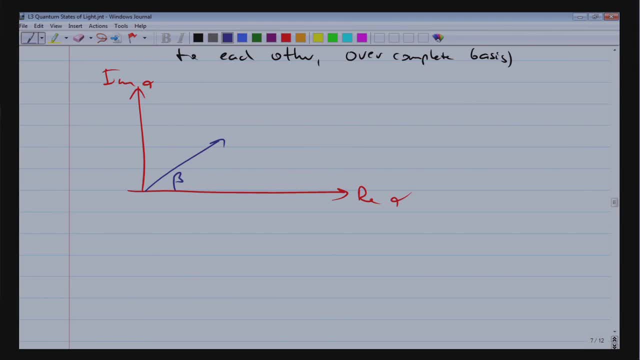 is the eigenvalue of the coherent state beta, then the quasi-probability is centered near beta And it's a decaying Gaussian. I'm not showing it to you here explicitly, but it is simply the vacuum state we discussed before, displaced by beta. 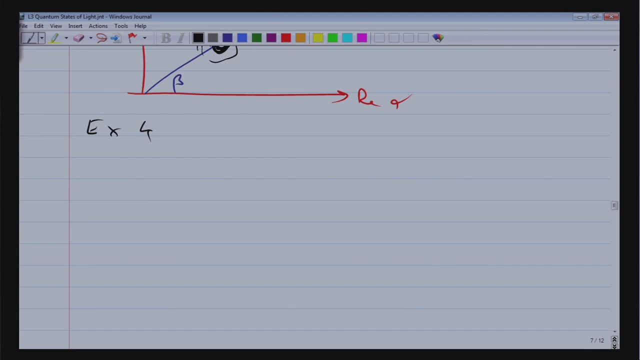 My fourth example, just to show you. so far, I've shown you that everything is Gaussian. Thermal light is a broad Gaussian. Coherent state is a narrow Gaussian. The vacuum state is a narrow Gaussian. Let me just show you something which is non-Gaussian, which 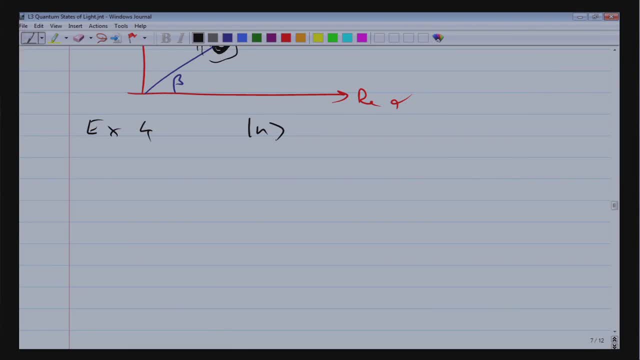 is the number state. If you put into the definition of the quasi-probability the number state and you calculate the quasi-probability as a function of alpha, then you have a Gaussian state. You find that what you get is actually not a Gaussian. 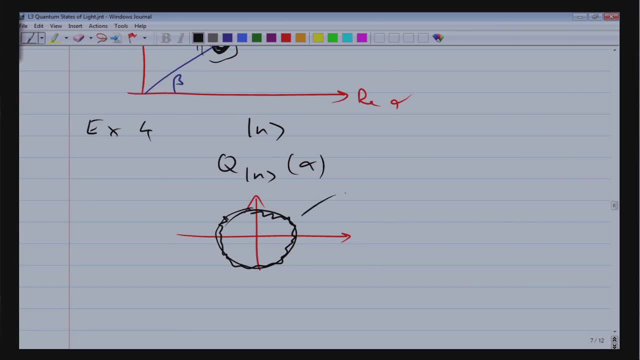 What you get is a ring, a ring with a certain width. So this is the representation of a number state, And the radius of this ring is the number state. That's the Gaussian, That's the Gaussian, That's the Gaussian. This is proportional to the square root. 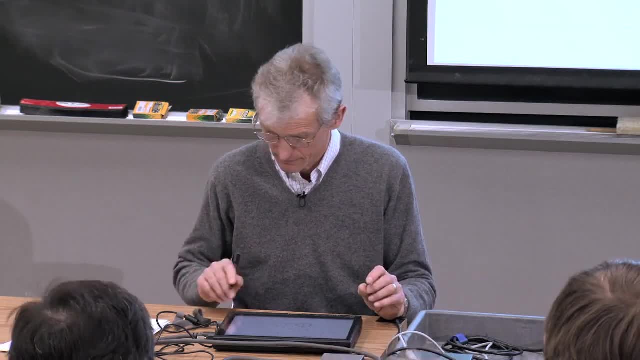 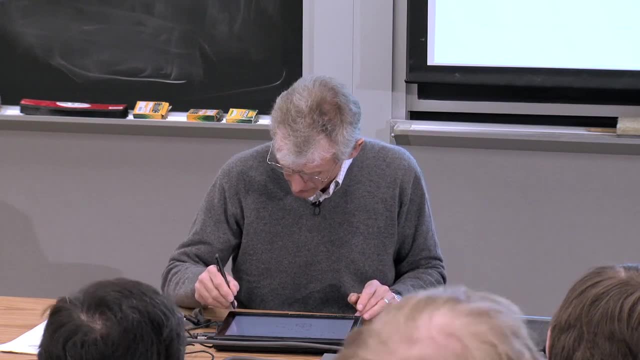 of the number of photons in the number state. We'll come back to photon states in much more detail very soon, but I just wanted to show you that at this point. So quasi-probabilities are not always Gaussian. They really depict something. 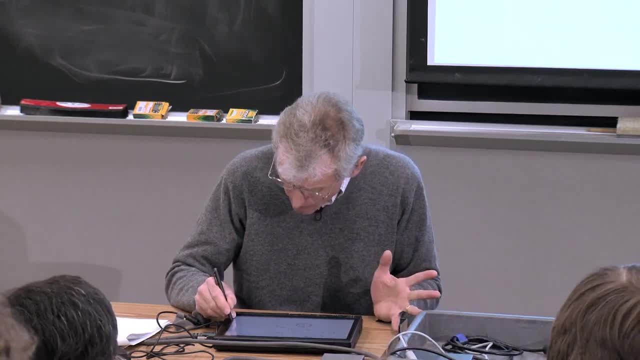 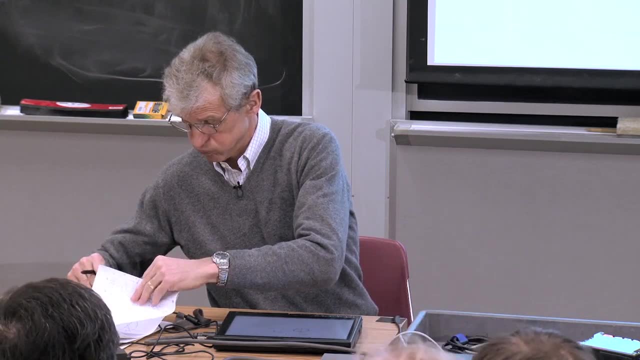 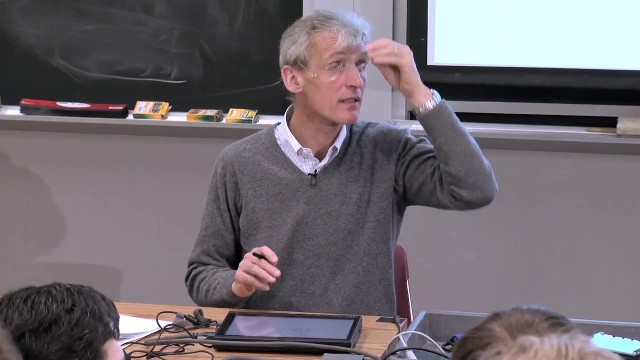 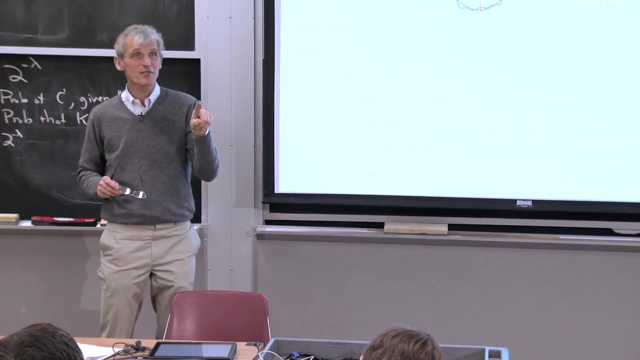 They show us something important about the quantum states of light. OK, Any questions. Yes, Is this a delta function, kind of in the radius, and do we have a little path where we go from 0 to 0? Can you hold the question for three minutes? 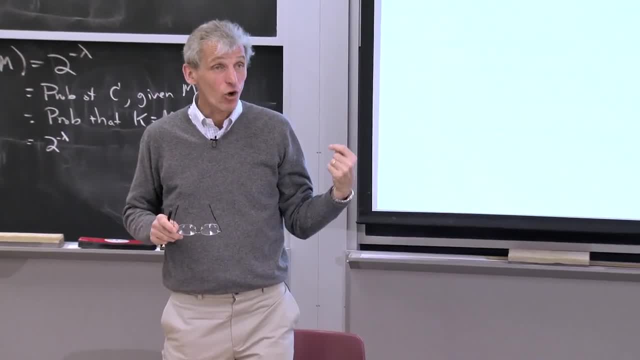 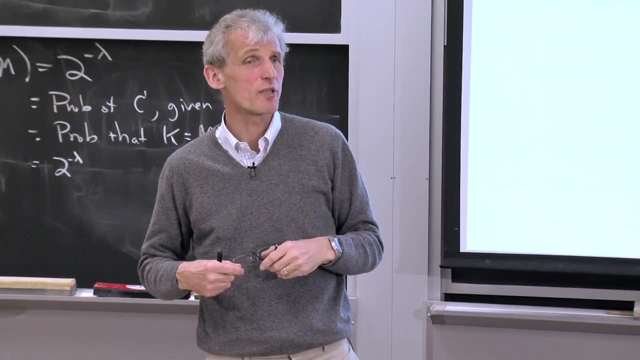 OK? The quick answer is: it's not, but in three minutes I want to tell you that there are three possible definitions of quasi-probabilities: the q function, the w function and the p function. And the p function In one of the functions it's a delta function. 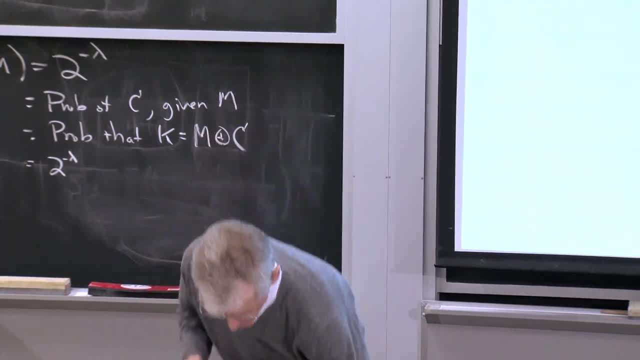 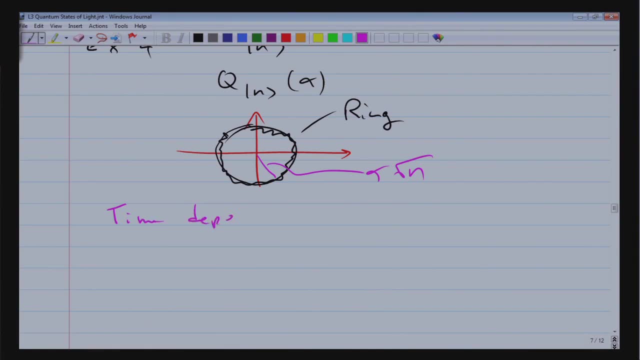 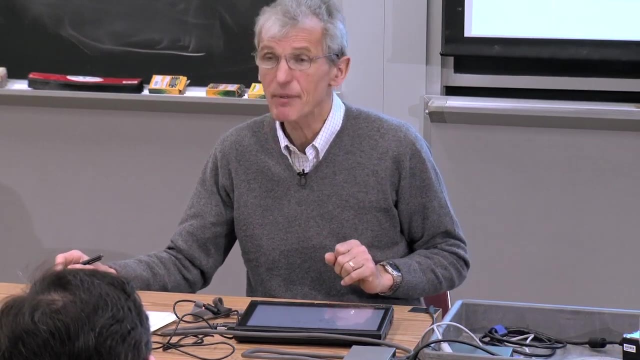 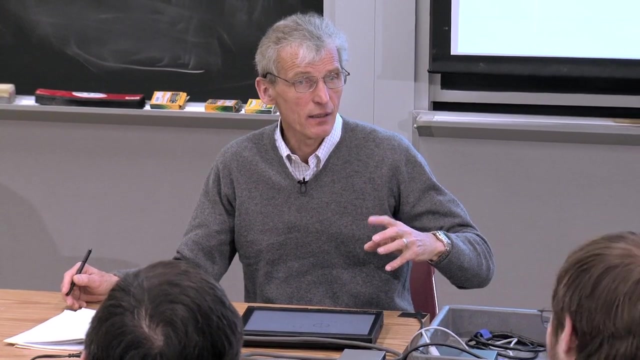 In the q function. it's not, But we'll come to that, But let's for now stick to the q function. The next thing we want to put in is the time dependence. I want to show you that when we have quantum states of light, 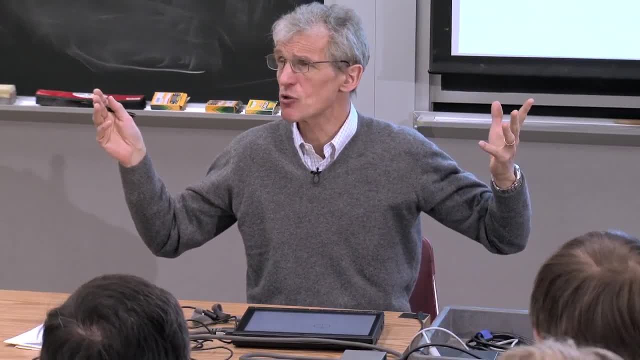 and right now, we've just shown the quasi-probabilities. OK, OK, So we have a quasi-probability distribution at a snapshot, at t equals 0.. What happens as a function of time? What I want to show you is and this: 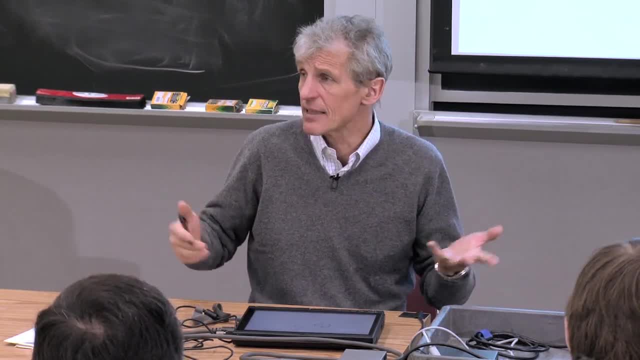 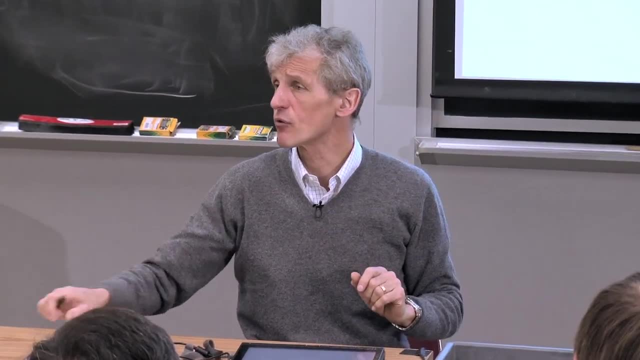 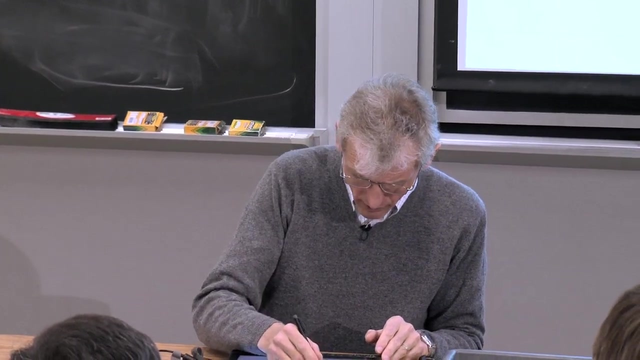 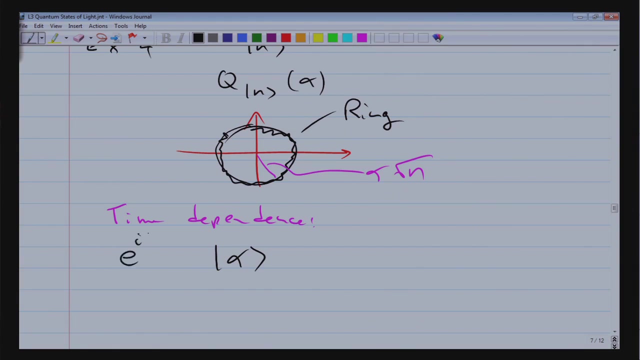 makes those quasi-probabilities also nice and intuitive that, as a function of time, the quasi-probability distribution simply rotates with an angular frequency of omega. So let me show that to you. We know that we have a coherent state And what we want to understand is what. 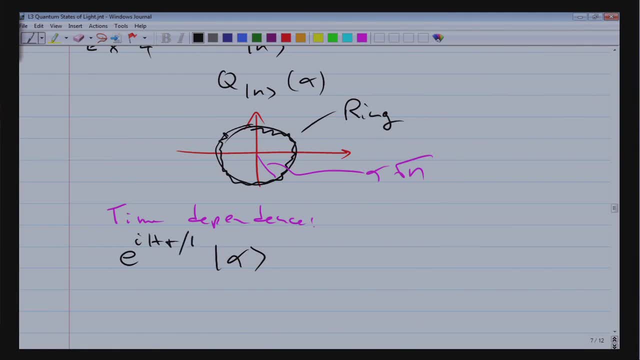 happens when we act on the coherent state with the time propagation operator, which is the Hamiltonian in the exponent. Well, in order to evaluate the left-hand side, we can simply take the expansion of coherent states into in the number basis, because we know. 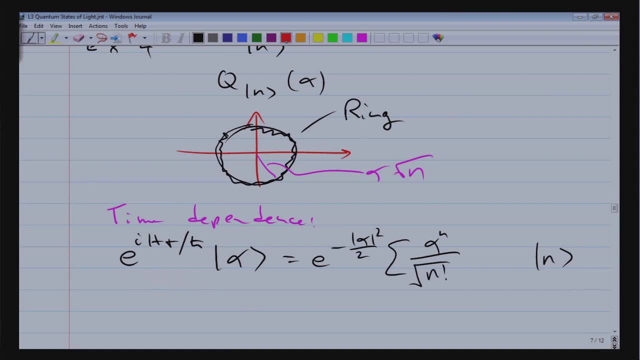 that the time evolution of a number state is simply the energy of the number state, which is given by the energy of the number state which is n times h bar omega. So now, if you look for a second at this expression, you realize that we can absorb the time evolution. 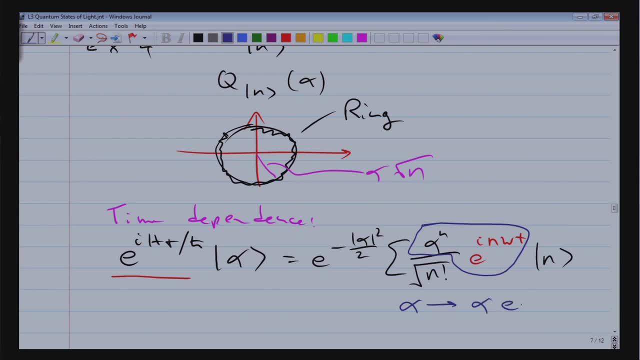 if we redefine alpha to become alpha times e to the i omega t. So in other words, the time evolution of the coherent state alpha preserves the character as a coherent state. It just means we get a new coherent state whose eigenvalue is now alpha times e to the i omega t. 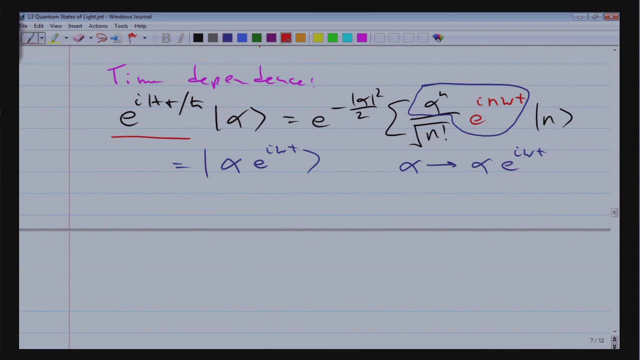 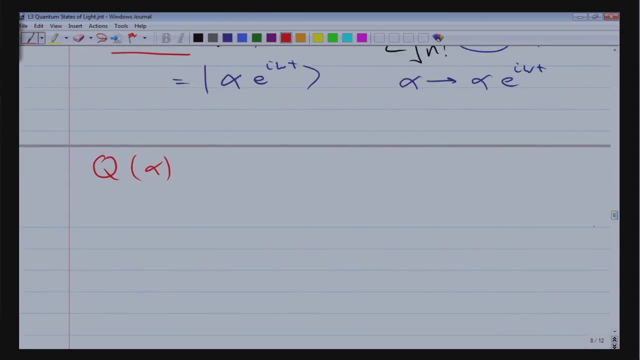 So that means the following: If you want to look, If you want to look at the time evolution in terms of quasi-probabilities, we have our diagram with the real part of alpha, with the imaginary part of alpha, And let's assume we had a coherent state, which happened. 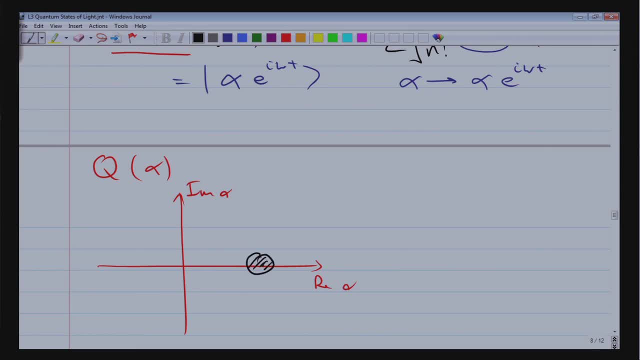 This is sort of now my circle, as you can see, A high contrast representation of a Gaussian. So this is a quasi-probability of the initial state alpha, But as time propagates it just gets multiplied with e to the i, omega, t. 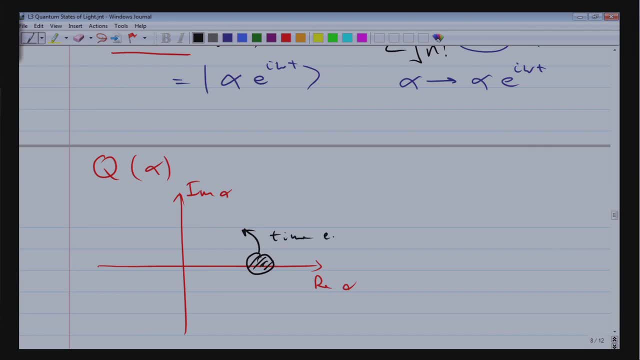 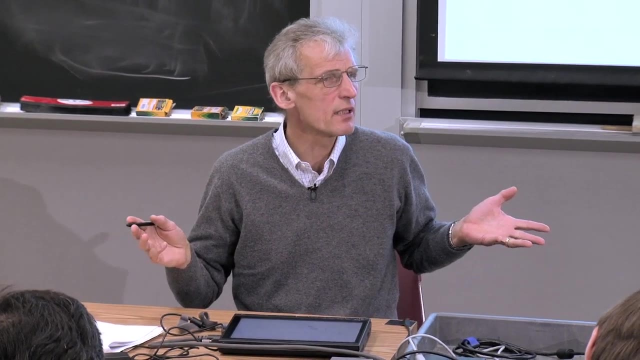 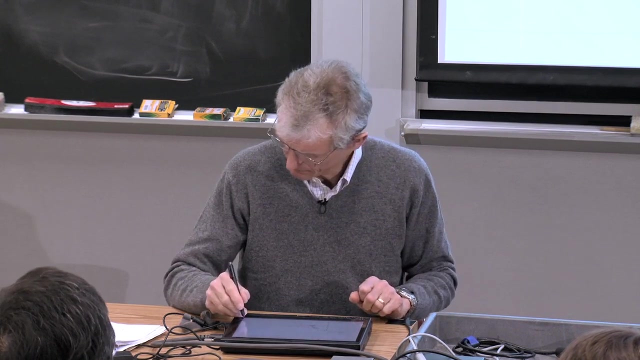 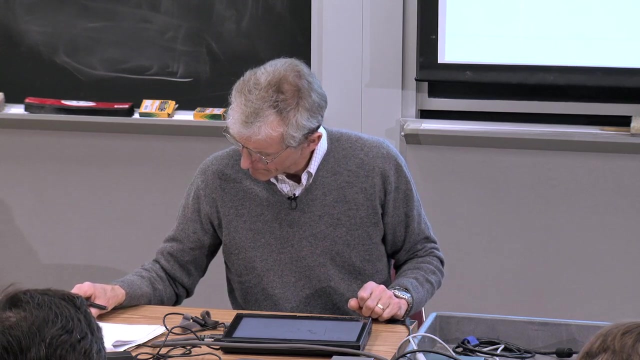 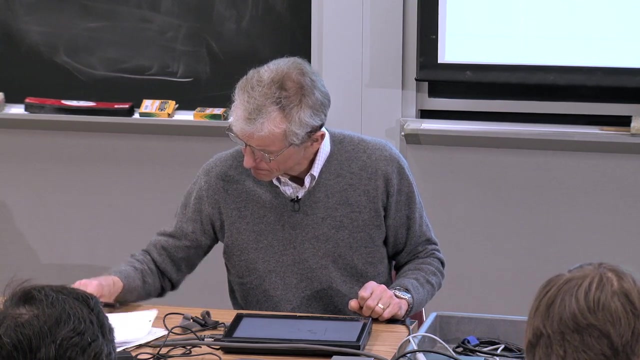 That means if the time evolution is just displacing the state over there and as time goes by, the coherent state is just moving in a circle, And after one full period of omega, we are back where we started Now. let me give you now an intuitive proof. 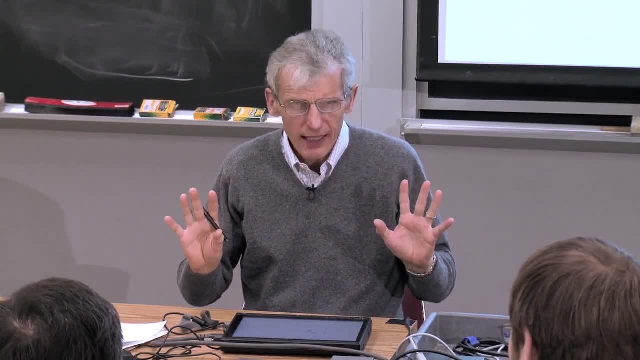 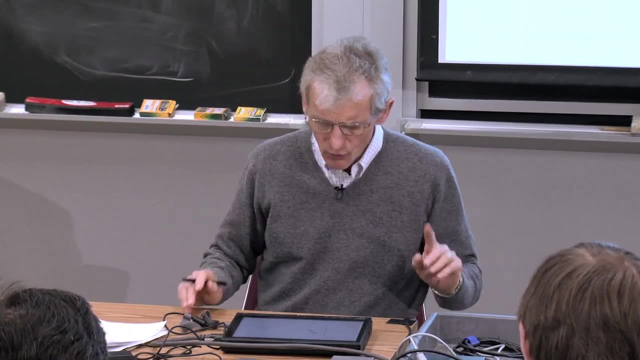 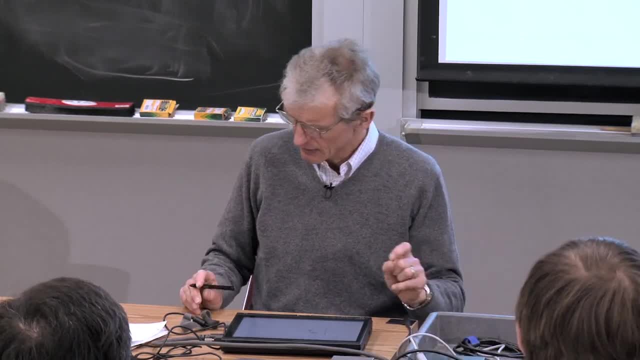 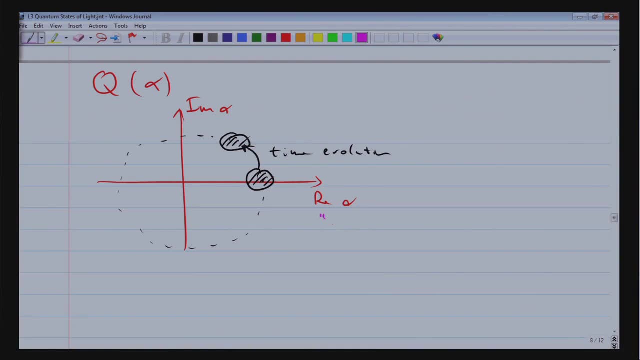 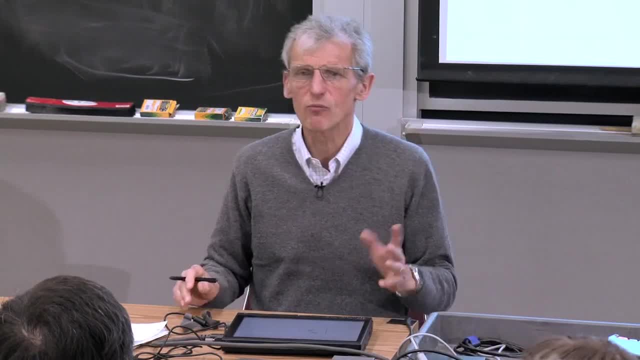 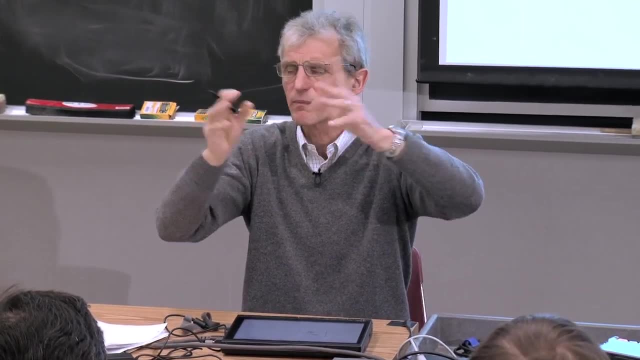 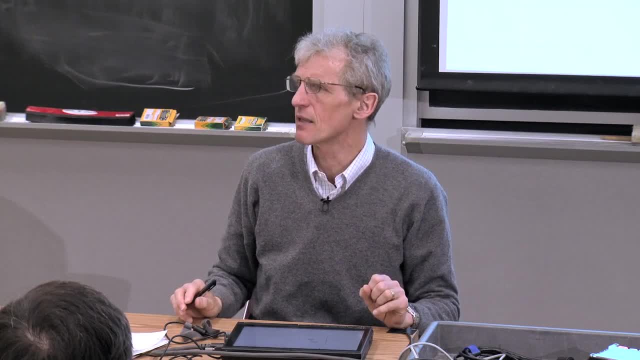 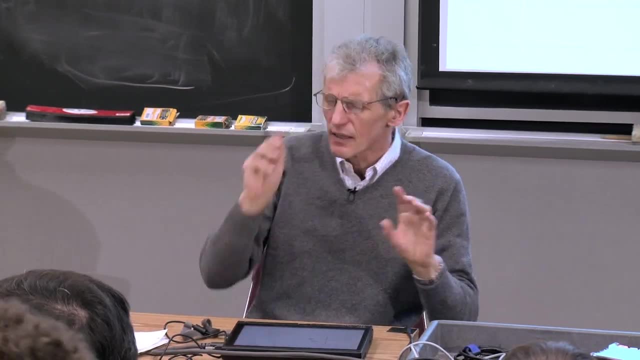 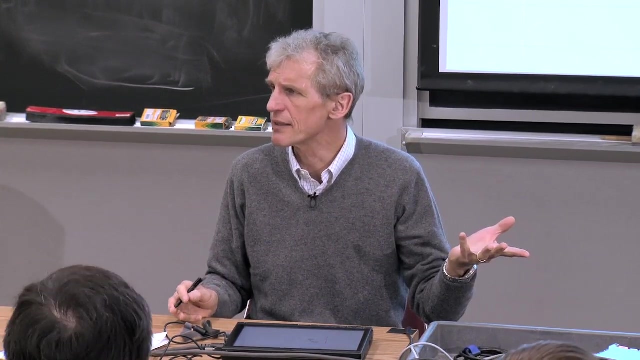 what the system actually does is. it simply rotates on a circle in phase space. The classical phase space is x and p, And I haven't really told you that. I didn't want to get lost in complex definitions. Quasi-probability is a generalization. 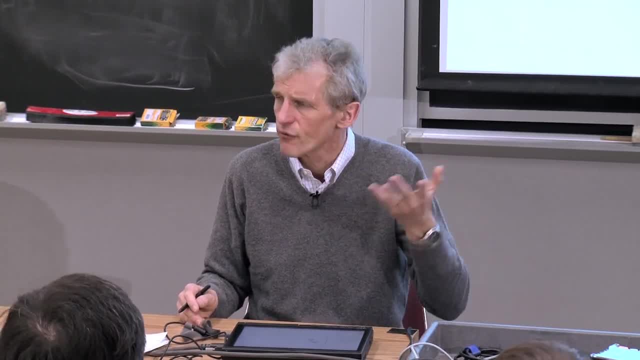 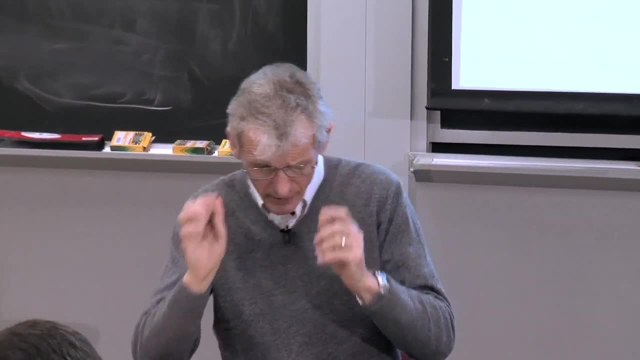 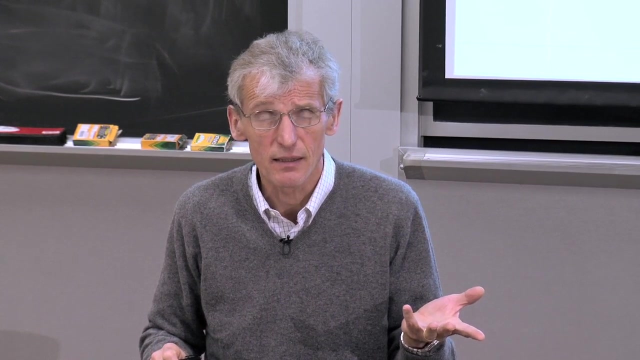 of the classical phase-based function, phase-based function as a function of p and x. So take my word for a second and allow me to identify the real axis with x and the imaginary axis with p. Well then, p is the electric field. 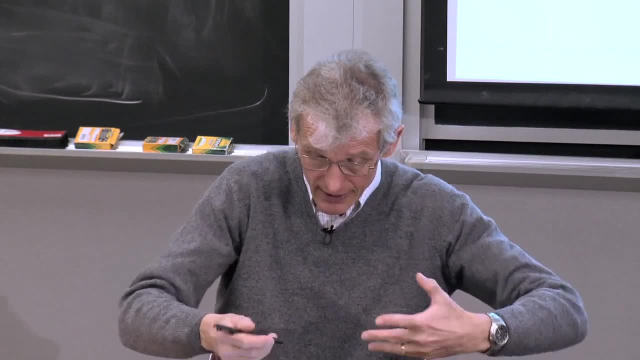 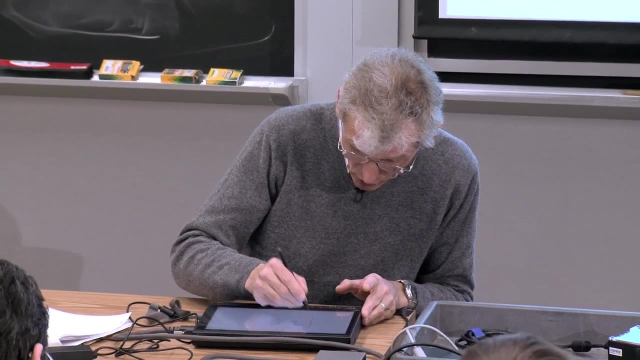 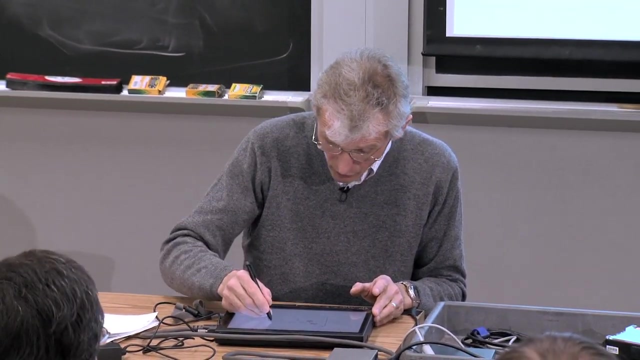 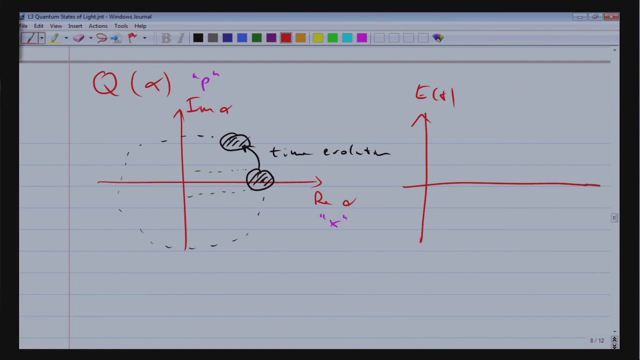 So now, what you should visually take from those pictures is that if you want to know what the electric field is, you just sort of project this fuzzy ball on the imaginary axis. So in other words, when I ask you, what is now the electric field as a function of time, 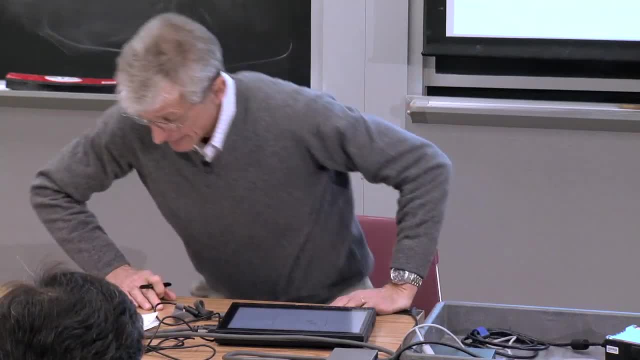 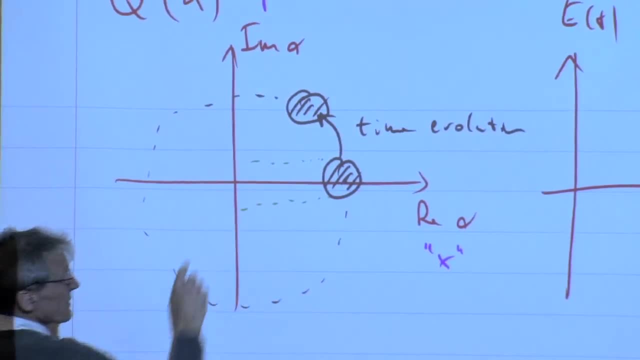 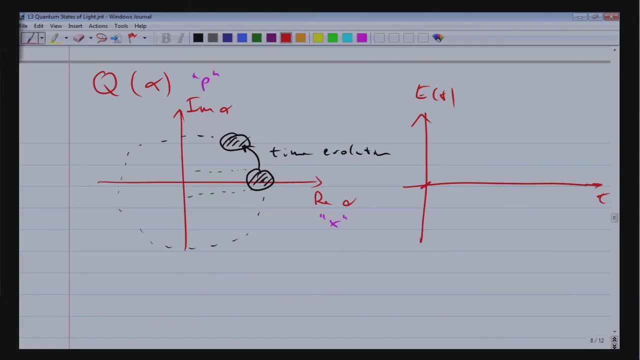 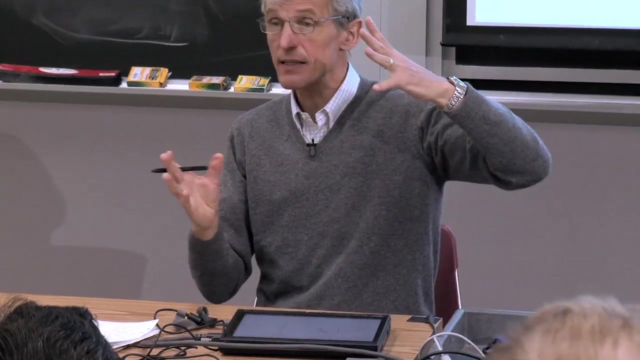 at t equals 0.. I project this onto the p-axis And what I get is something which is centered at 0.. But it has also a certain fuzziness. The fuzziness is given by the size of the disk or by the width of the Gaussian. 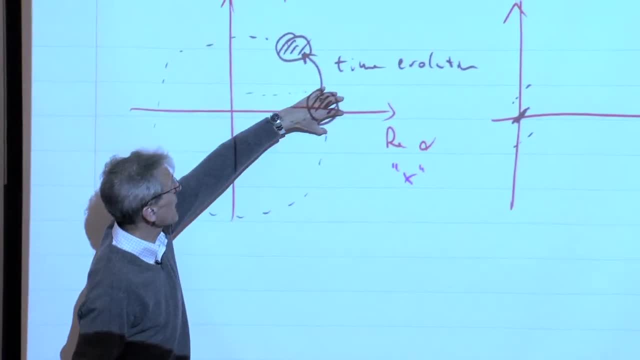 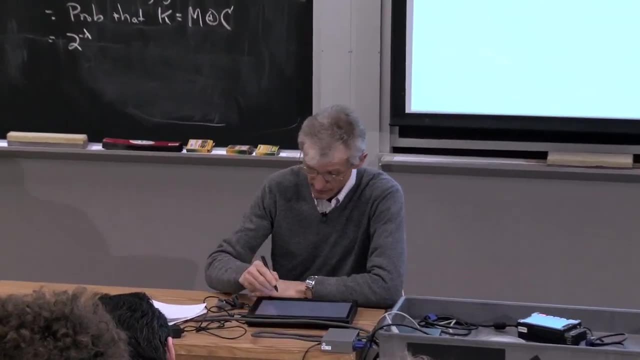 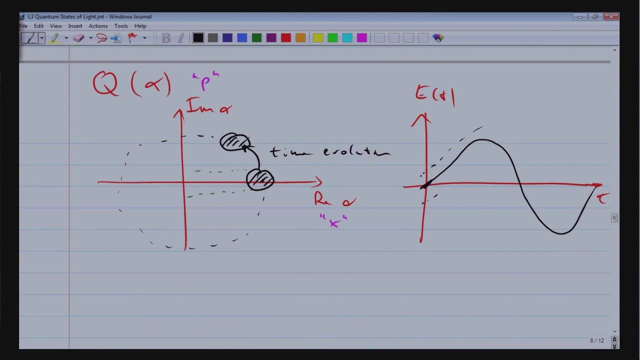 And if I now use this picture as a function, a function of time, as this fuzzy ball rotates around, the electric field goes up and down in one cycle And the fuzziness moves with it. So the fuzziness here for the electric field. 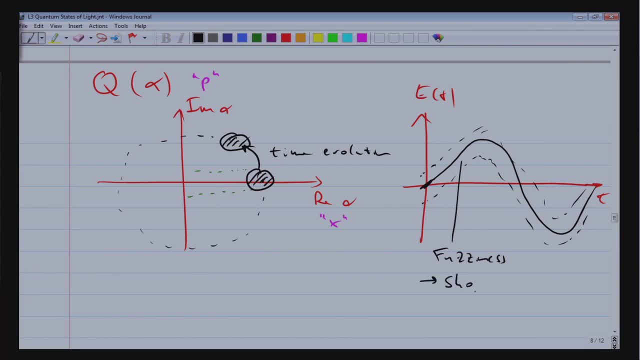 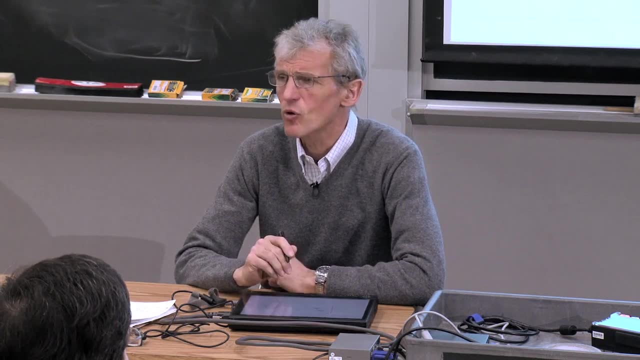 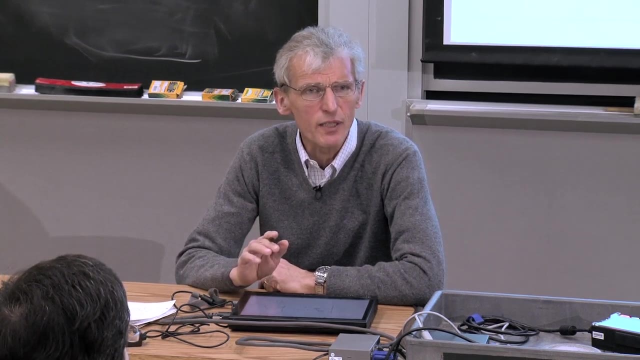 is related- and that's what we want to discuss next week- is related to shot noise. I also want to tell you that the coherent state is, to some extent, the best possible way to define an electric field. It's a minimum uncertainty state. 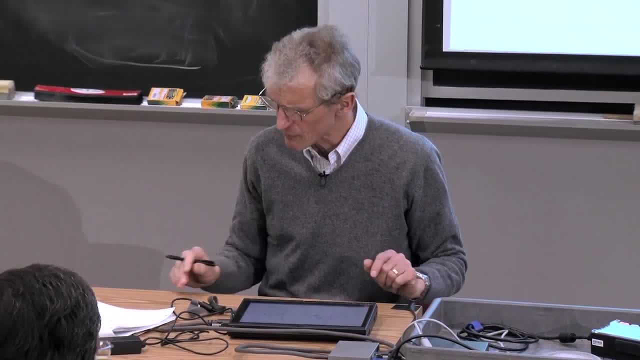 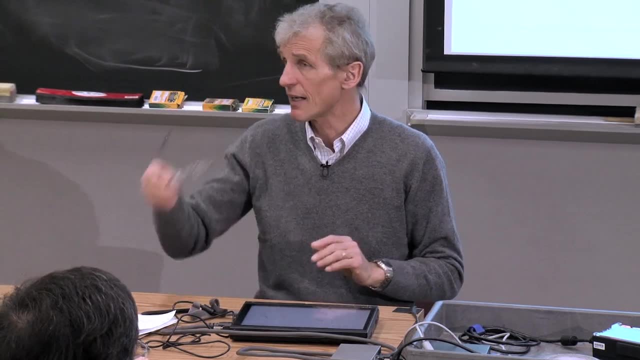 I'm going to show you that the coherent state is sort of, at the minimum, of Heisenberg's uncertainty relation. So I think if you take this picture you will immediately realize that you draw the quasi-probability You project on the vertical axis. 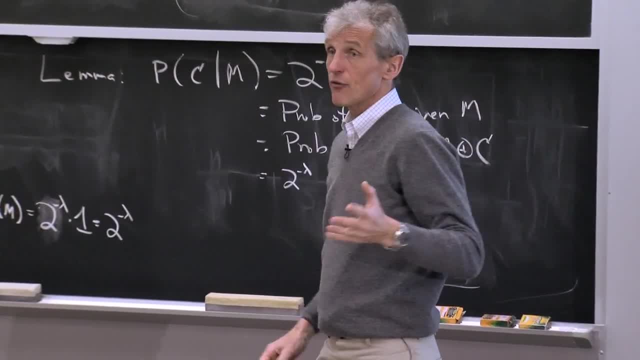 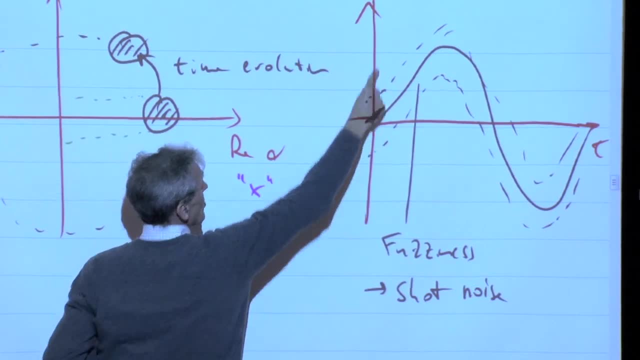 and you get the electric field That tells you immediately if you have a thermal state, which is the Gaussian centered here. you project it, You get an electric field 0. It has an enormous fuzziness but it's 0.. 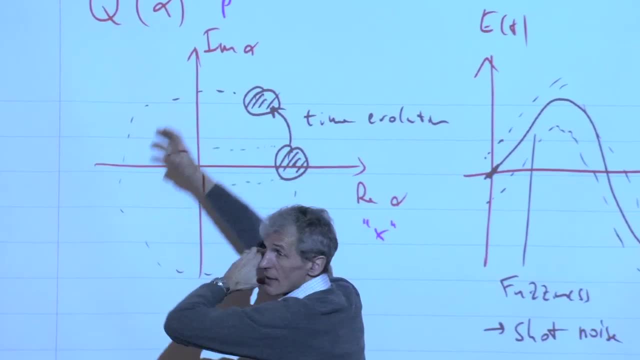 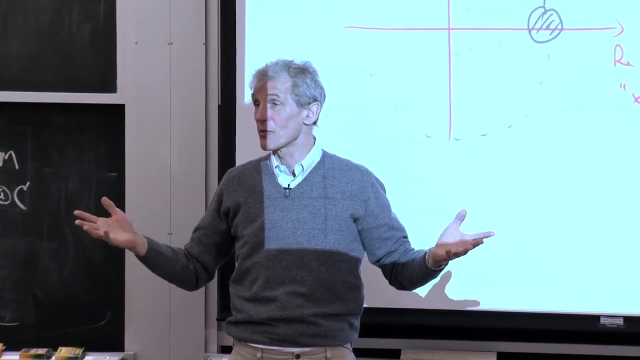 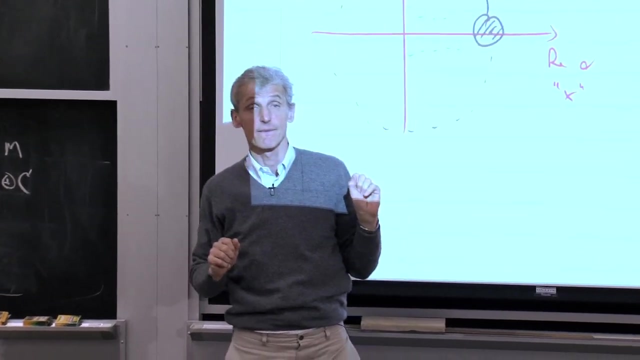 And this picture that everything rotates with angular frequency. omega also tells you, as expected, that in a thermal state, well, it's already a circularly symmetric distribution. When it rotates, nothing changes Since the equal operator is. couldn't you find the eigenstate of that operator? 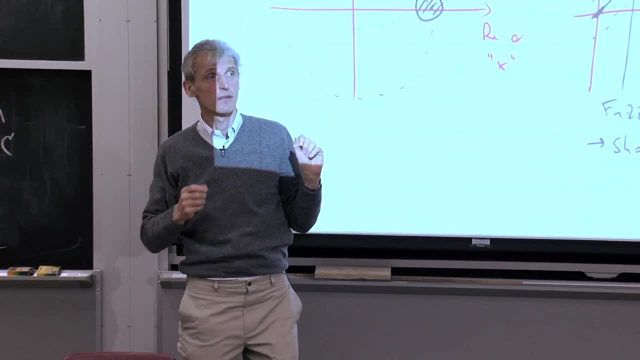 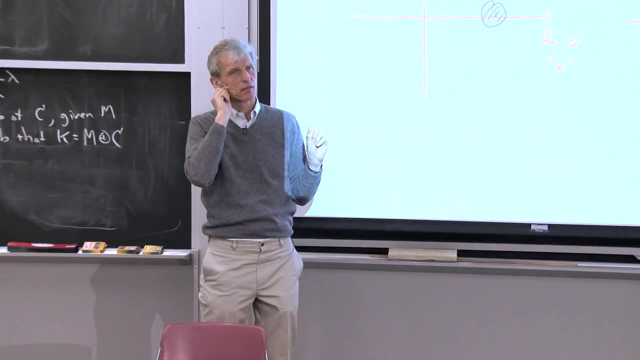 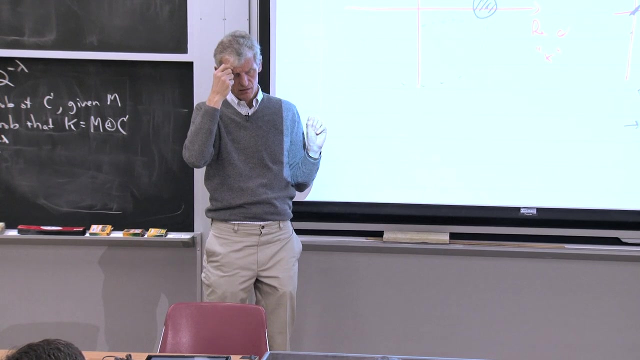 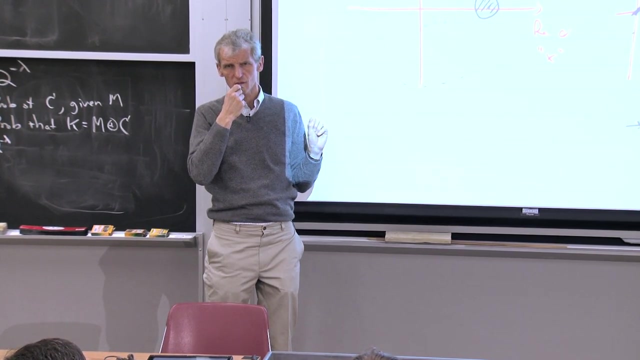 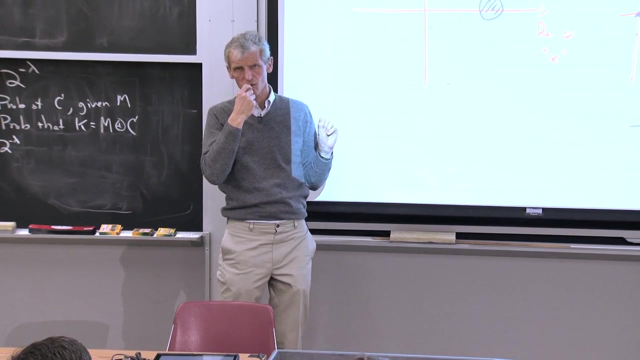 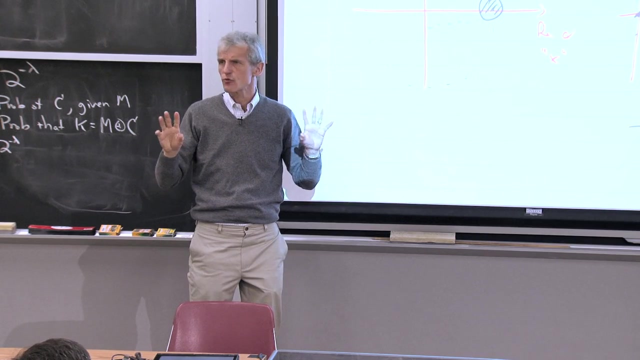 itself, and then get rid of this- the eigenstate of the harmonic oscillator, and so not stationary at all. A little bit confused now, Actually. do people mind if I teach a few minutes longer? I can just finish. I want to have one footnote. 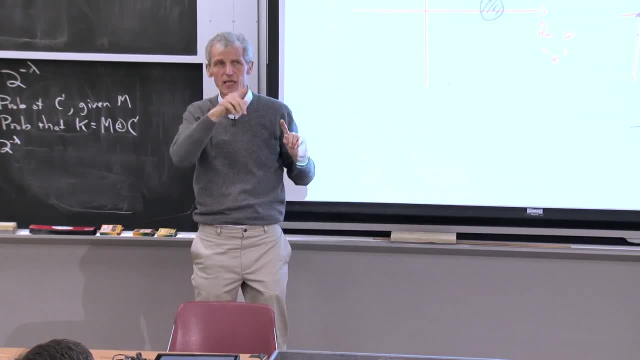 I really want to sort of give it to you because I think it will help. It will help some of you. Pardon, We have a class starting at 2.30.. There's a class starting at 2.30?? Yes, 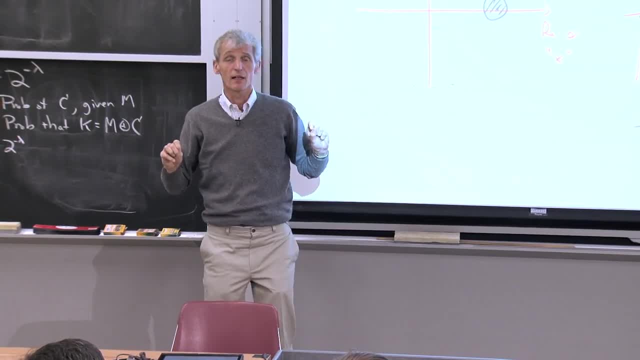 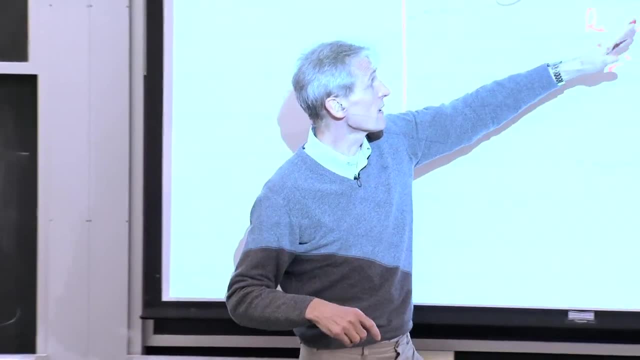 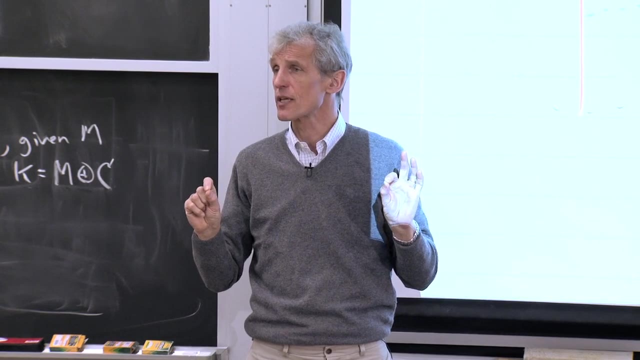 Then I have to wrap up, Sorry. Then let me just tell you what I will do at the beginning of the next class, What I've told you here with the projection of the electric field. this is not 100% rigorous for the quasi-probabilities Q. 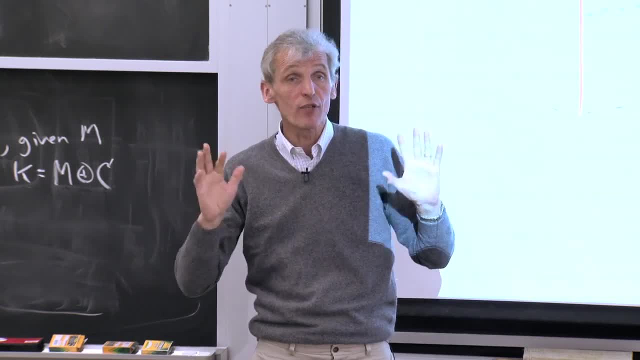 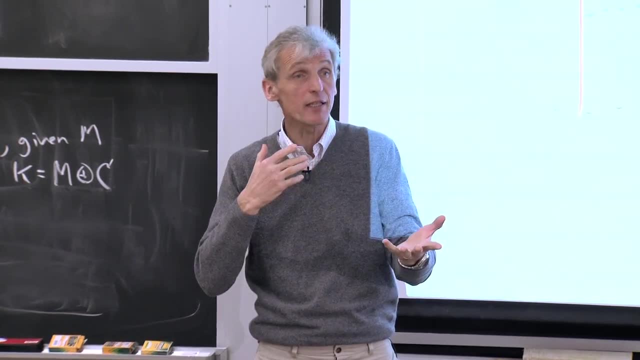 Due to the non-commutativity of operators. when we generalize phase-based function into quantum mechanics, we can order operators in a symmetric way, in a normal way, in an anti-normal way, And therefore there are three different quasi-probabilities. 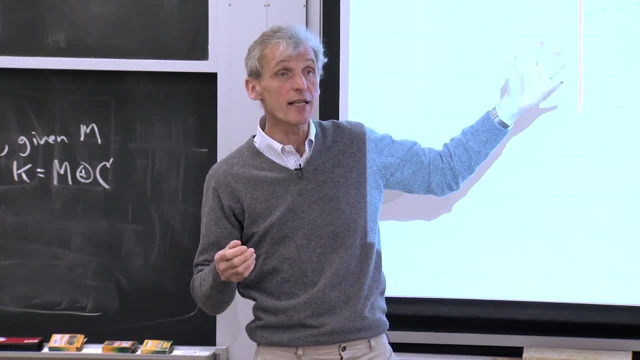 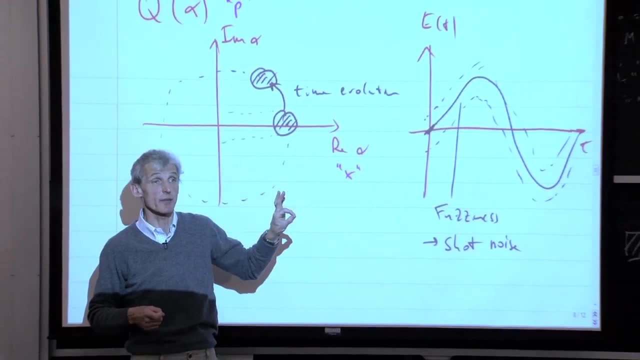 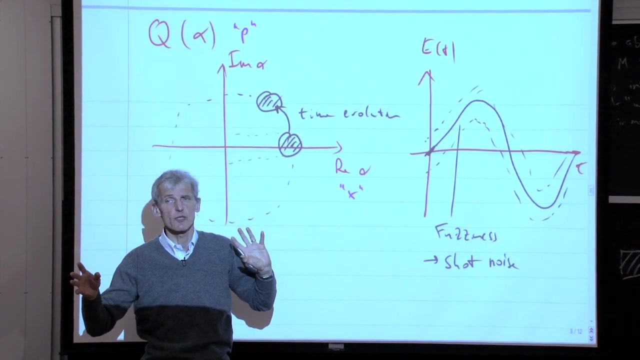 The Q probability is the easiest to define. It comes in very handy. But what I showed you with the projection does not rigorously apply to the Q distribution. It applies to the P or W distribution, But the difference is, unless you really go into subtleties, are minor. 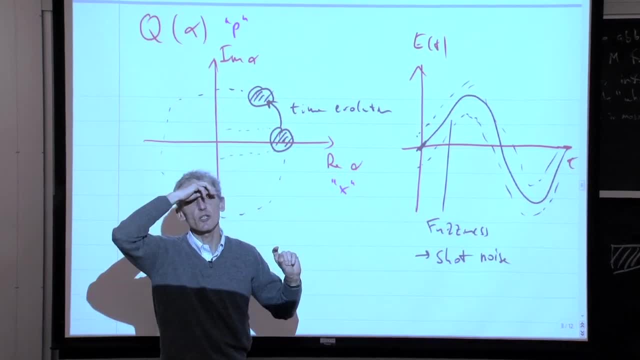 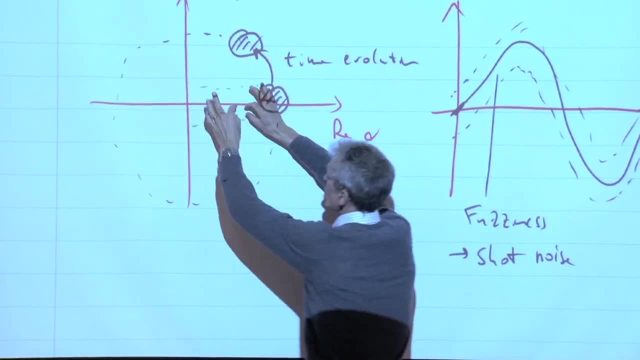 So, intuitively, what I did is correct And, to answer your question, an eigenstate of the electric field. I have a little bit problems with that Because if you take this projection, what you need is you need something which is very, very narrow.